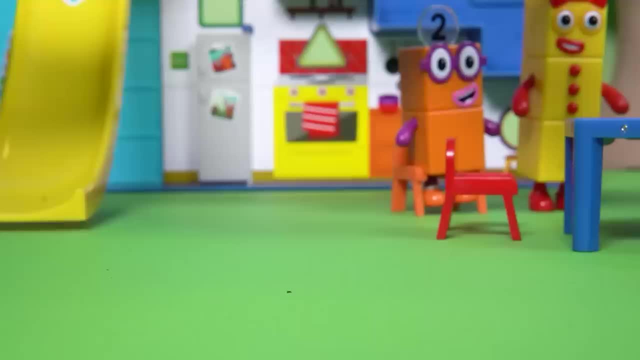 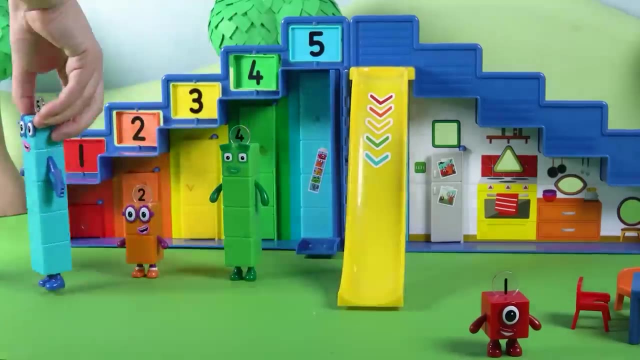 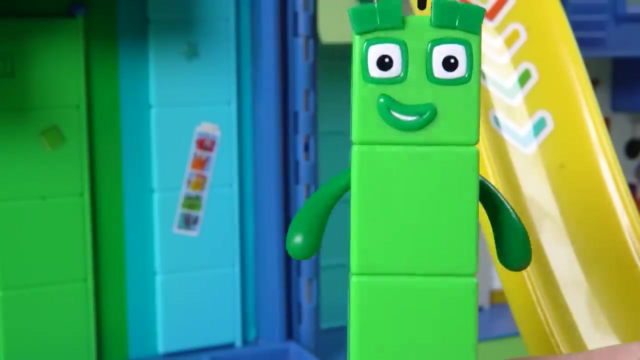 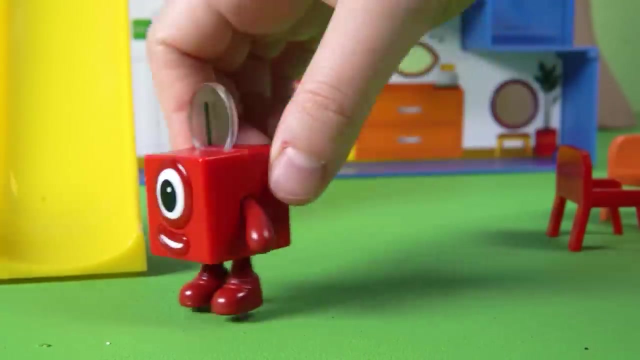 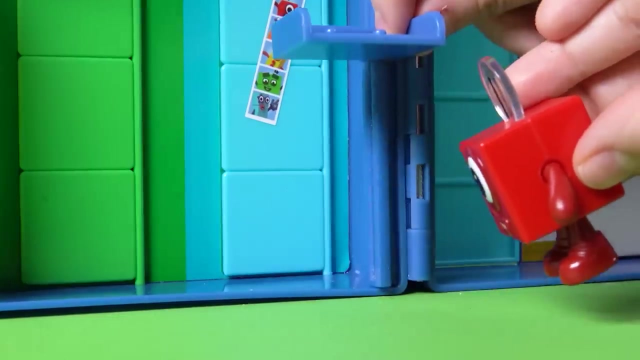 They're going to play hide-and-seek: Ready and Hide One, two, three, four, five, six, seven, eight, nine, ten Coming Ready or not? And off goes Number Block One. She's looking high and low, near and far. 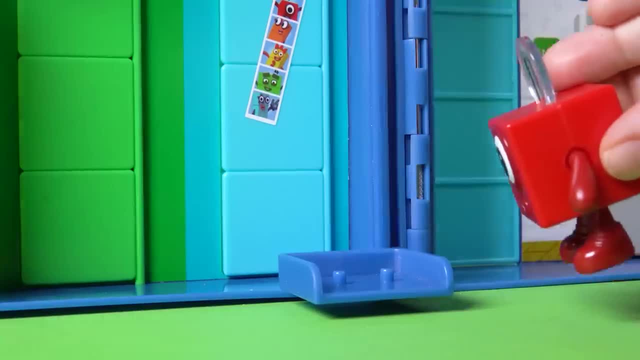 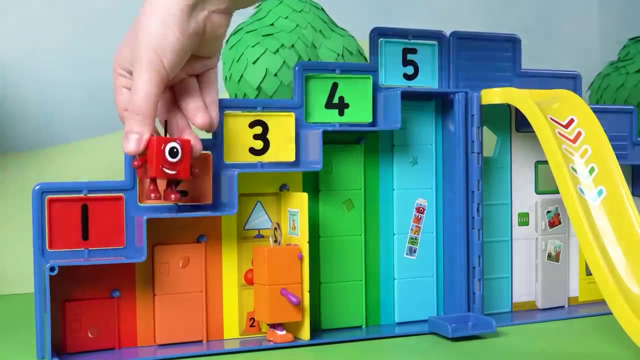 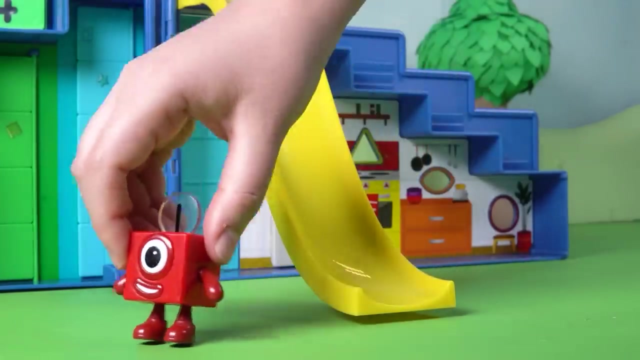 Up and down goes the lift, but no Number Blocks here. Let's keep looking Up up up the stairs. she goes Whee, Now down the slide. What's that? by the lockers? Ah, Those are Number Blocks. 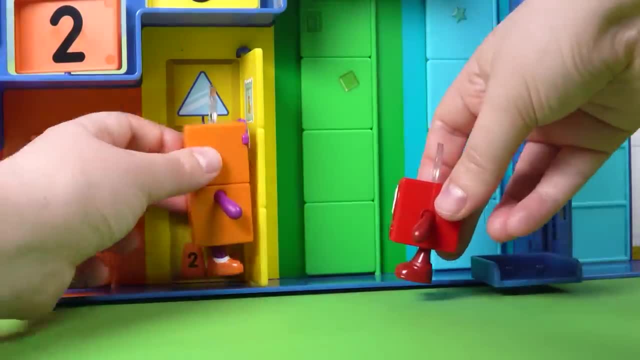 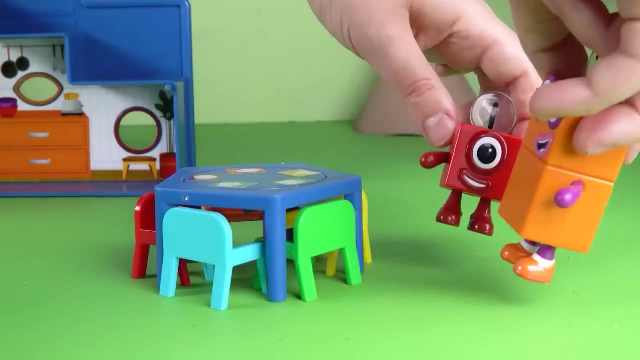 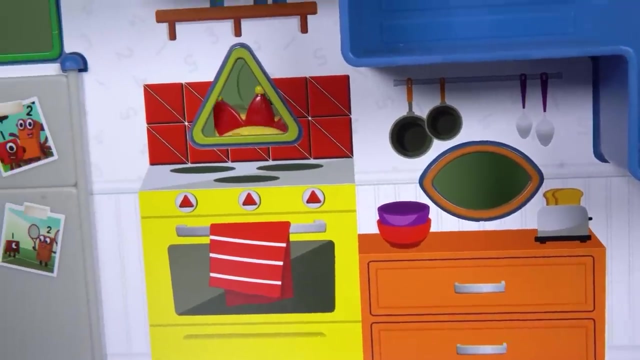 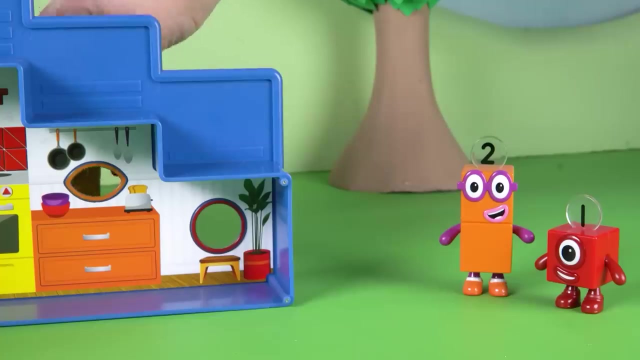 Number Blocks. Number Block Two's dancing shoes. We've found our first friend, Ah-ha. What's that sticking out behind Three's window? One, two, three red triangles. Of course It's Three's hat. We've found Number Block Three. 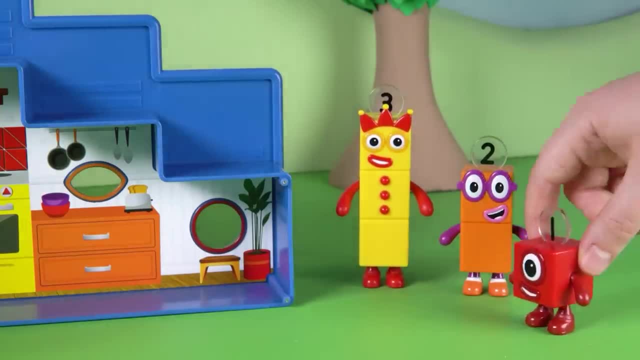 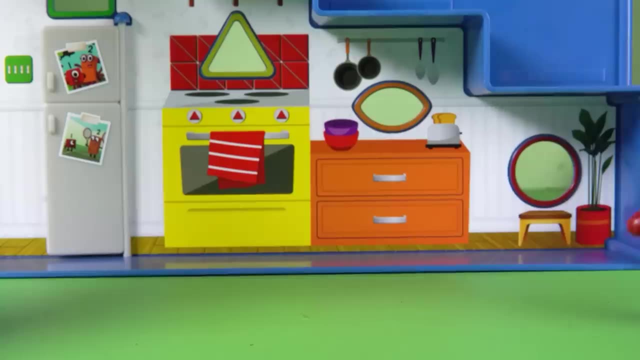 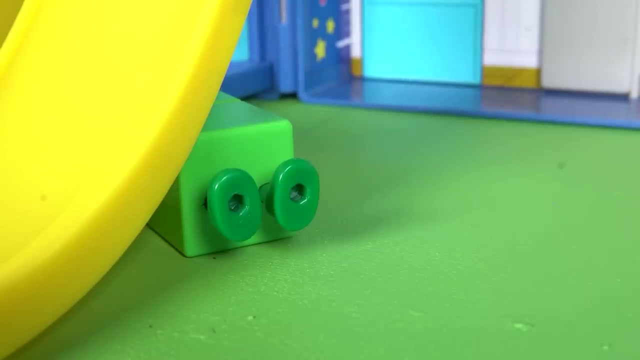 Hooray, Two friends found And two more to go. Let's keep looking Number Explorers. Where's one going? There's no one in the kitchen, But what's that under the slide? It's Number Block Four. 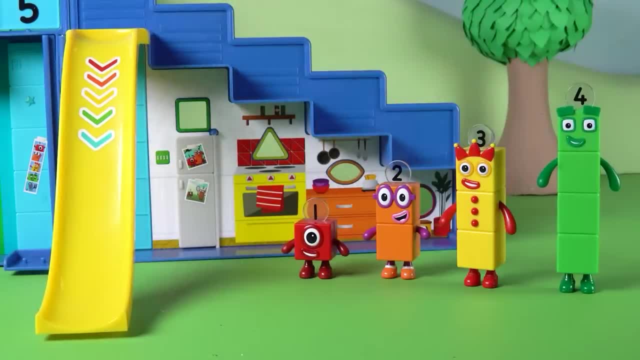 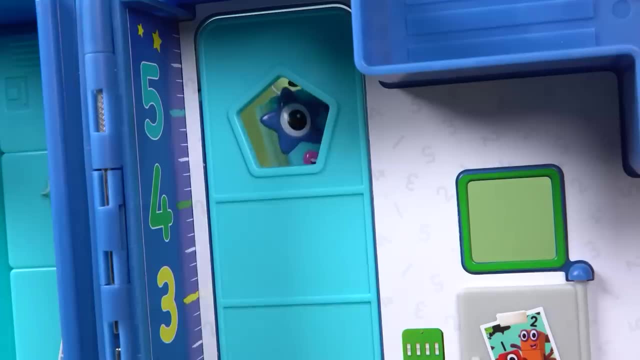 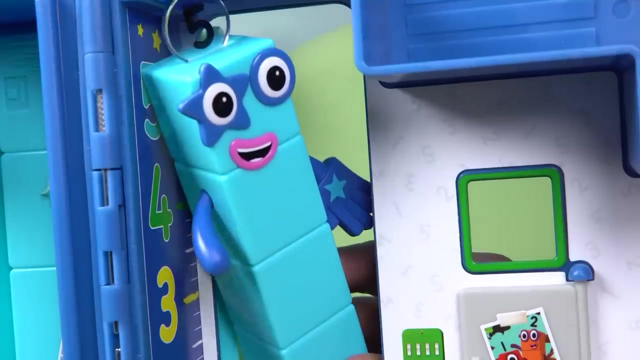 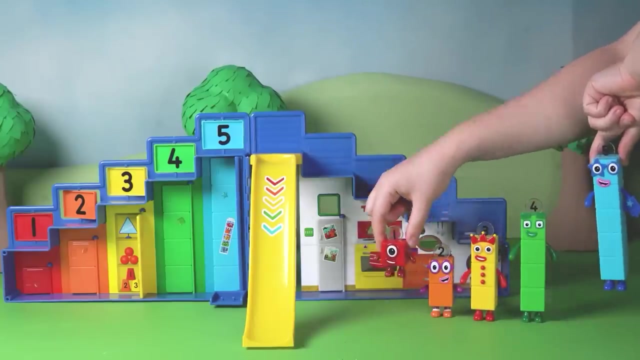 Only one more friend to find. Where could Number Block Five be? What's that behind the big blue door? It's Number Block Five's starry eye. We've found the last friend, Hooray. All of the Step Squad have been found. 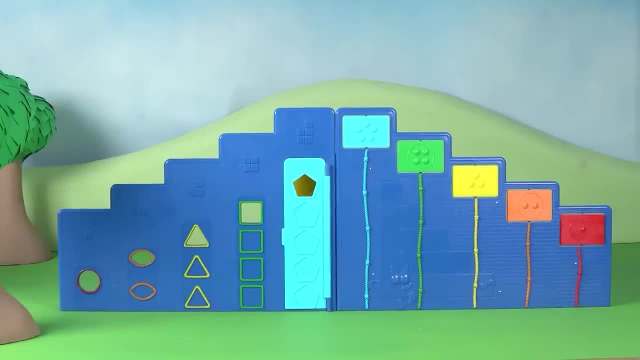 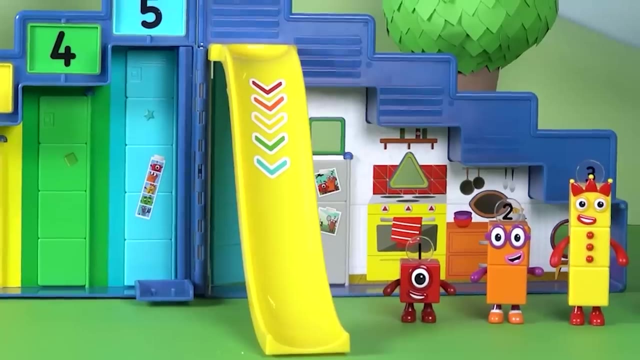 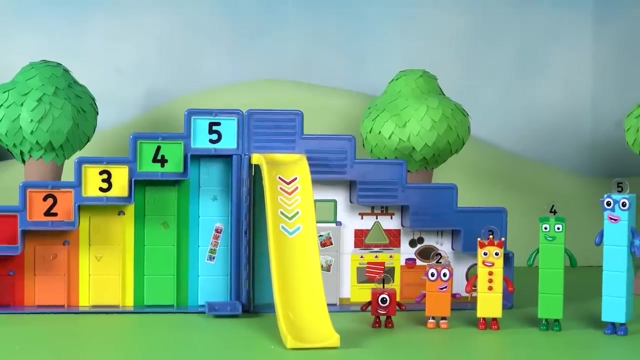 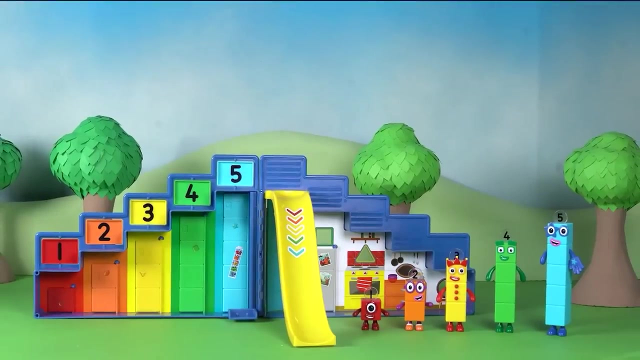 But wait, Who's that? Shh Hush hush, It's Number Block Fifteen. What a fun day at the Number Block Step Squad Mission Headquarters. Our Number Block friends had a great time playing hide and seek. I wonder what adventures we'll imagine next. 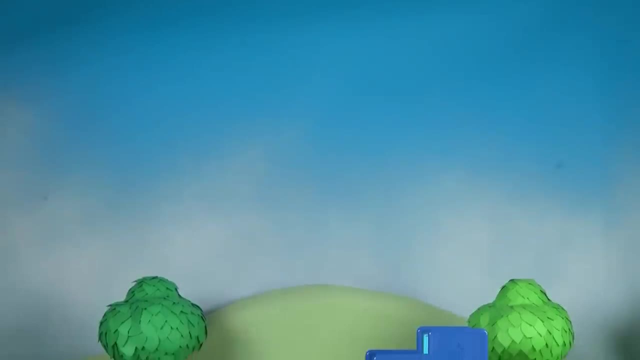 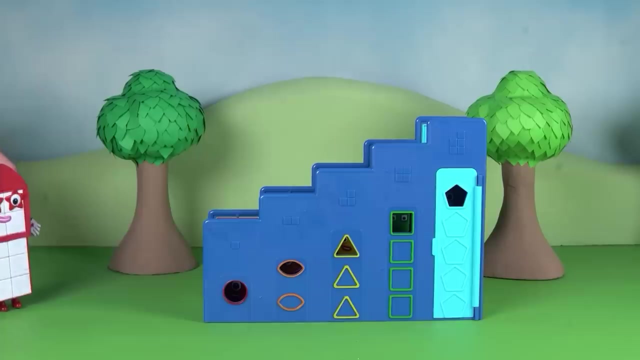 Welcome back Number Explorers to the Number Block Step Squad Mission Headquarters. Look, Number Block Ten is here And she's trying to blast off into space. Aha, Number Block Ten has a plan. She sees the big, big steps of the Step Squad Headquarters. 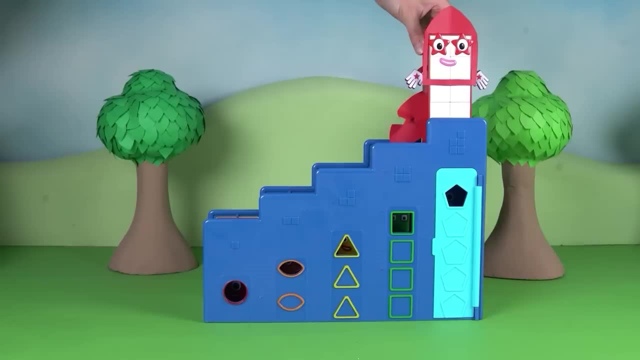 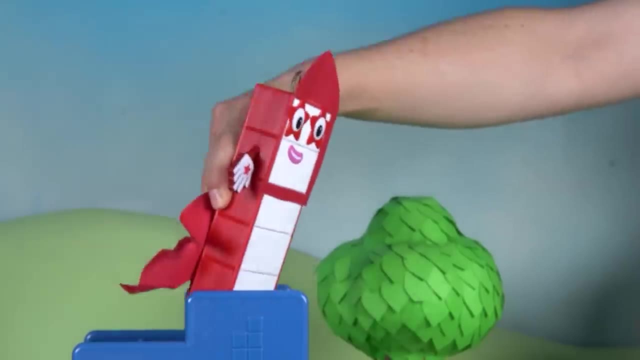 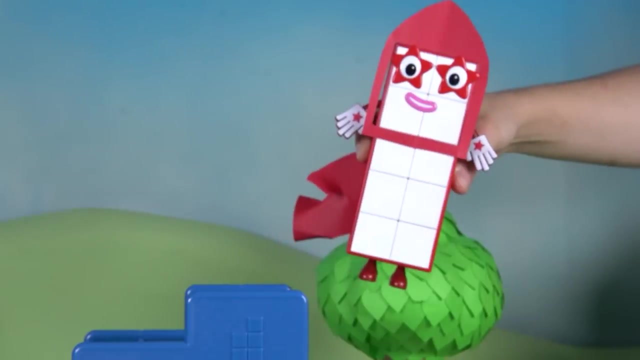 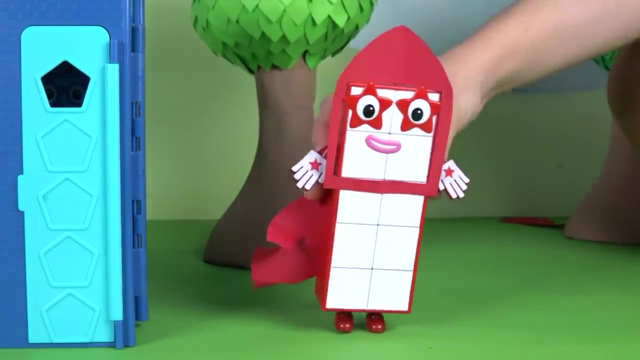 Maybe, just maybe, if she goes up, up, up, she can jump high enough to touch the sky. Oh no, Her rocket wings still won't work And she lands with a funny plop. Poor Number Block Ten. She wants to fly so much, but her wings are being very naughty. 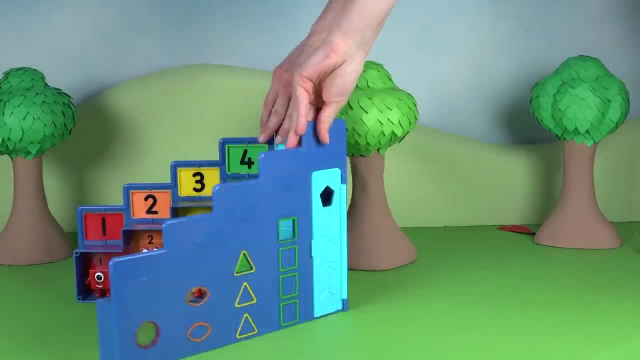 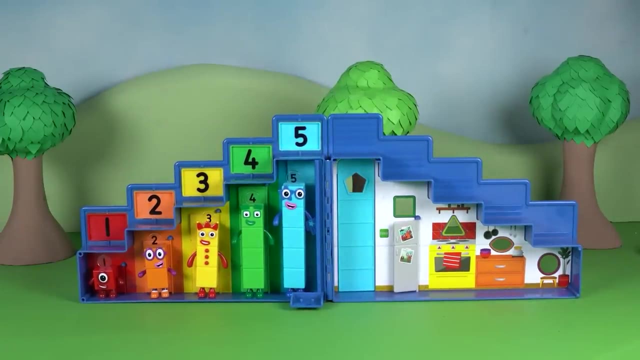 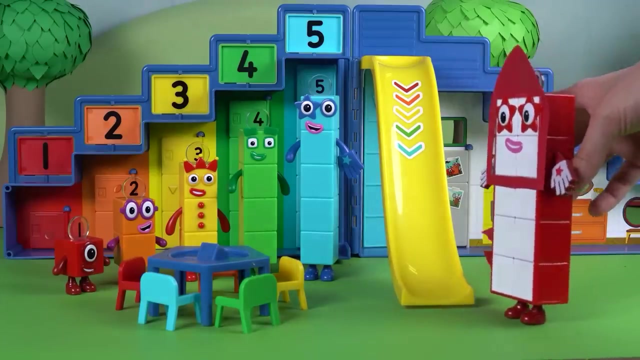 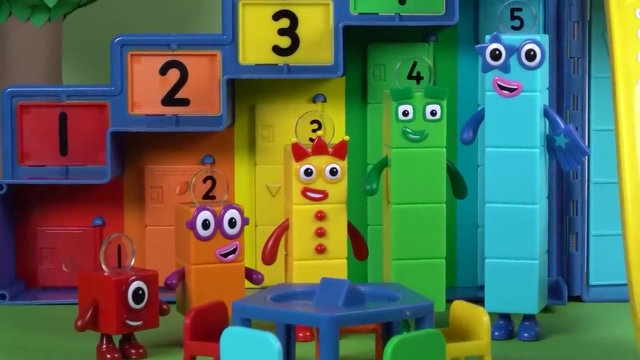 What can she do? Who can help her? Don't worry, Number Block Ten, The super special secret Step Squad, might have a plan. They're very good at helping their friends. The Step Squad is thinking, thinking, thinking. They need a big, big plan to help Number Block Ten fly. 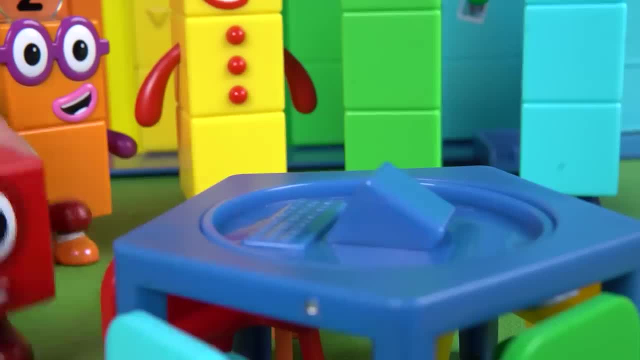 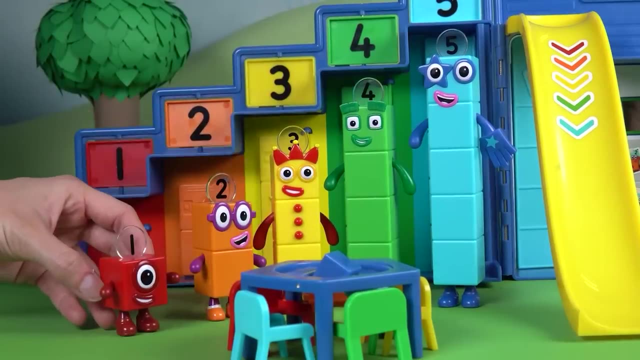 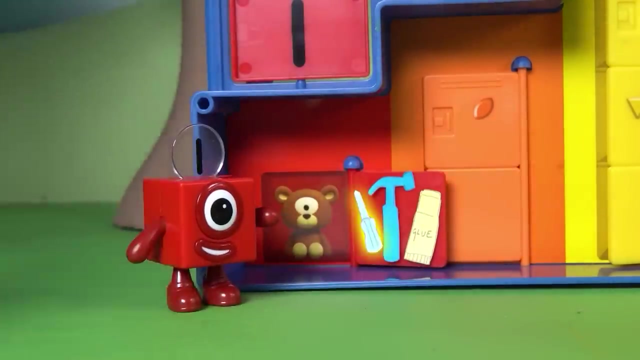 What can they do? Aha, They have a plan, A five-step plan. Let's see what it is. Step one: Gather all the tools they need: One screwdriver, one hammer and one glue stick Ready to start fixing. 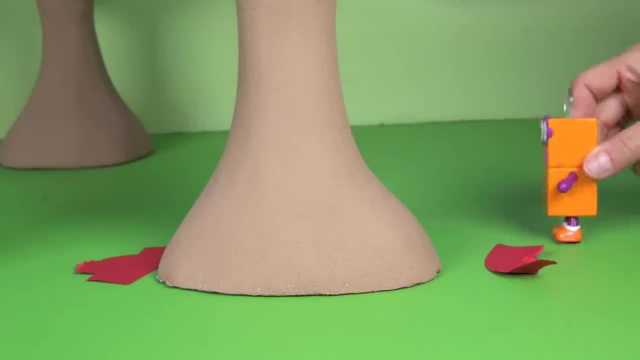 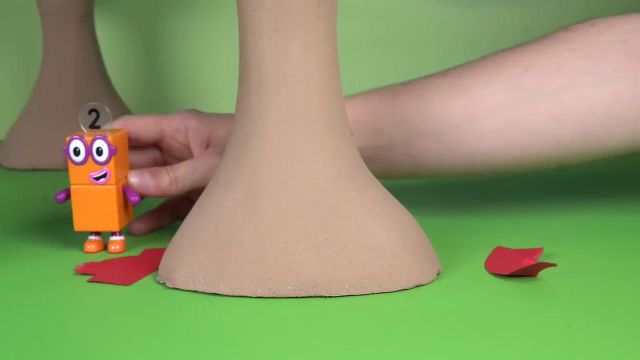 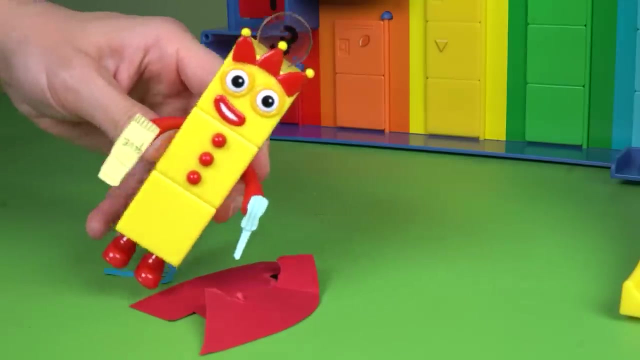 Step two: Find all the broken pieces of Number Block Ten's wings Look high and low. They must find them all. Step three: Carefully put the pieces back together. A little glue here, A little screw there, They're getting fixed. 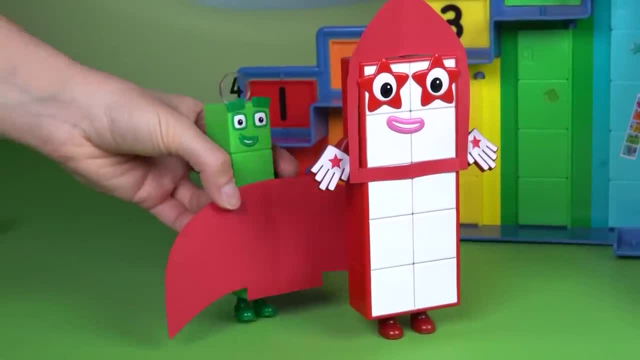 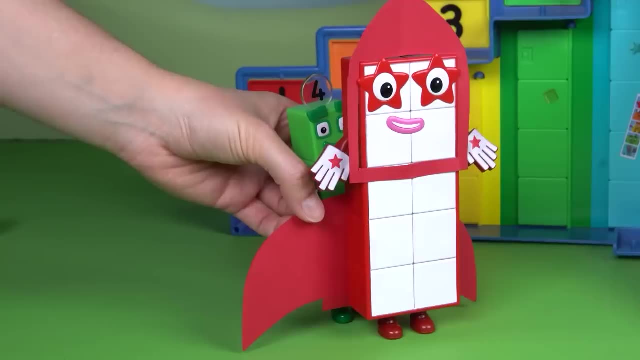 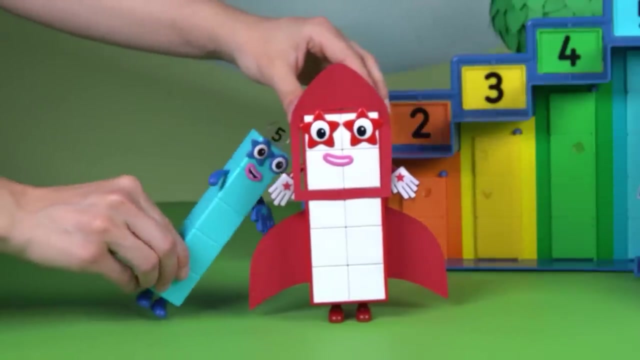 Step four: Put the wings back on Number Block Ten. They must fit just right, Not too loose, Not too tight. Step five: Give the wings a gentle wiggle to make sure they're strong and fixed. Hooray, No more broken wings. 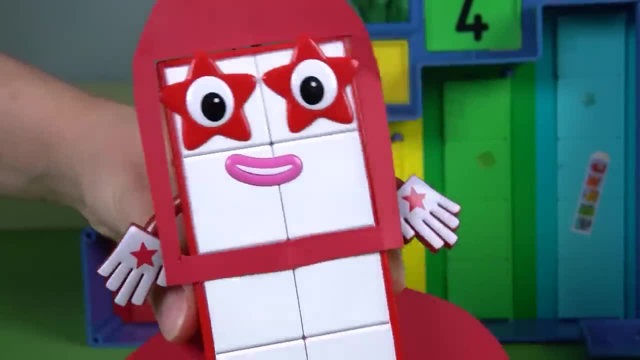 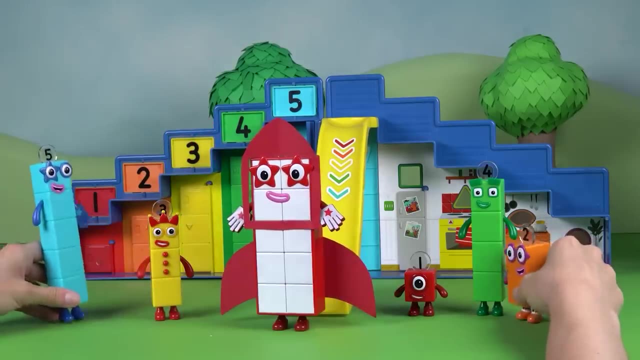 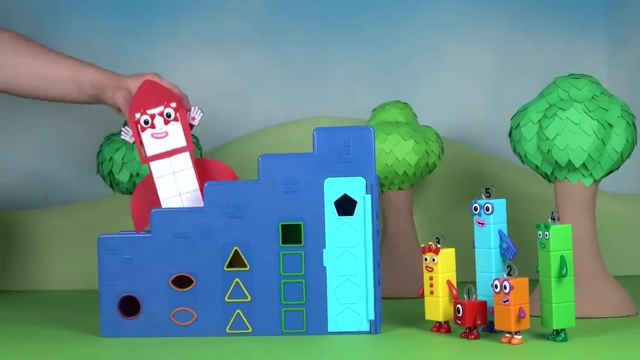 Look at those wings. They're all fixed and shiny thanks to the Step Squad. Number. Block Ten is so happy and can't wait to fly Up the stairs. she goes One, two, three, four, five steps. She's almost ready. 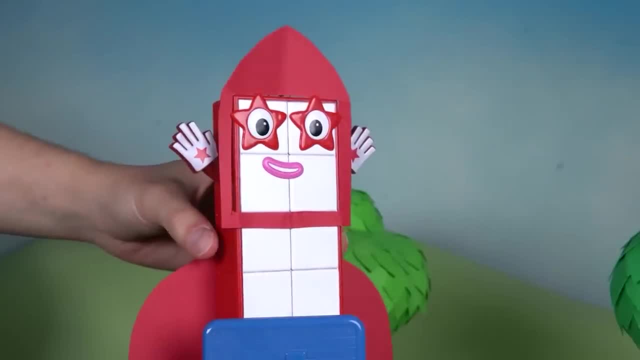 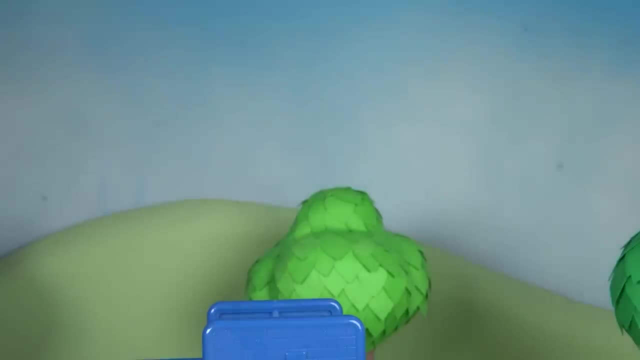 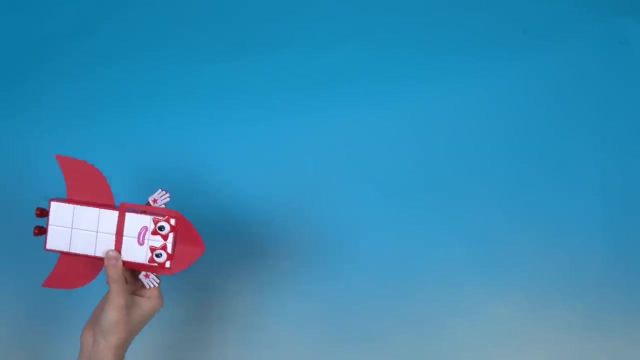 Are you ready to see her fly? Here she goes. Three, two, one blaster. Woohoo Weehee. Look at her, go Yeehee. Number Block Ten is flying. She's off to explore space. 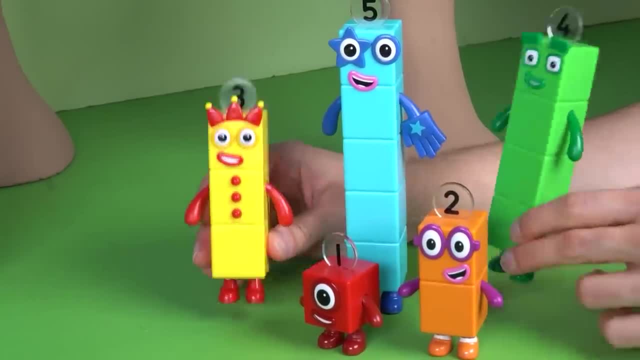 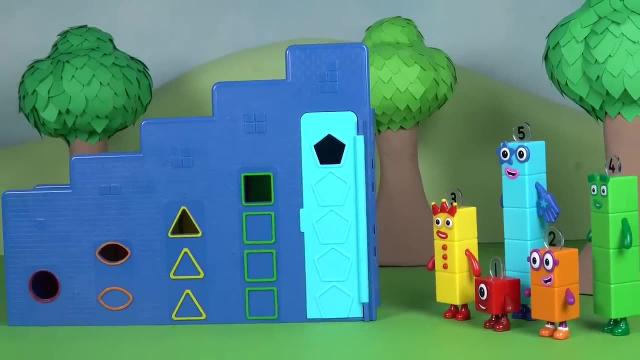 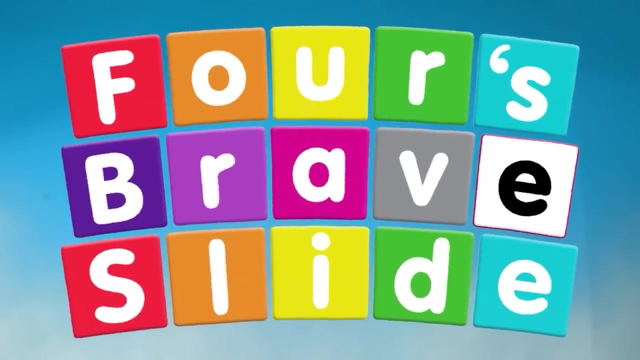 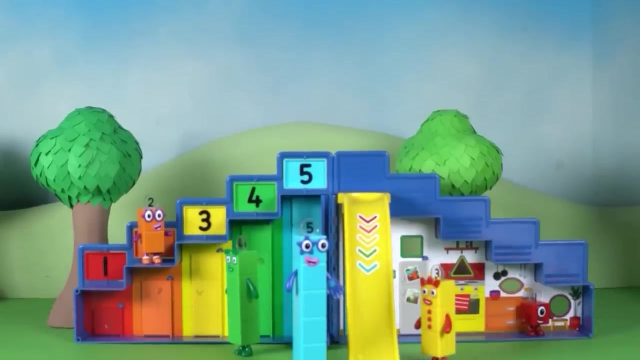 All thanks to her friends, the Step Squad Hooray. What a fun soaring adventure. I wonder what we'll imagine next time. Welcome Number Explorers to the Number Block's Step Squad Mission Headquarters. Let's see what stories we can imagine today. 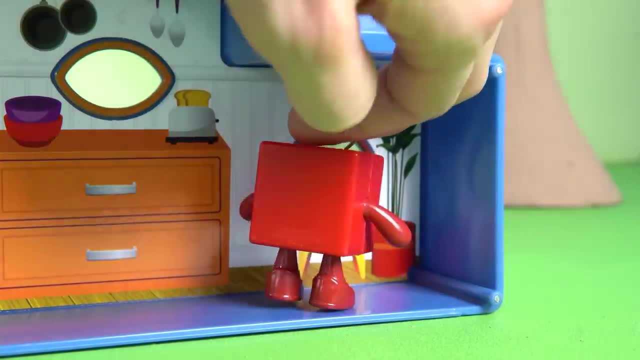 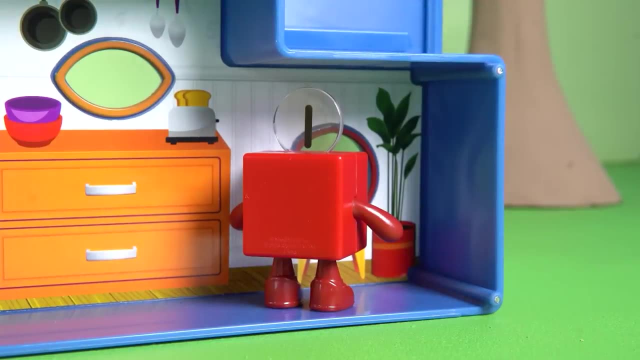 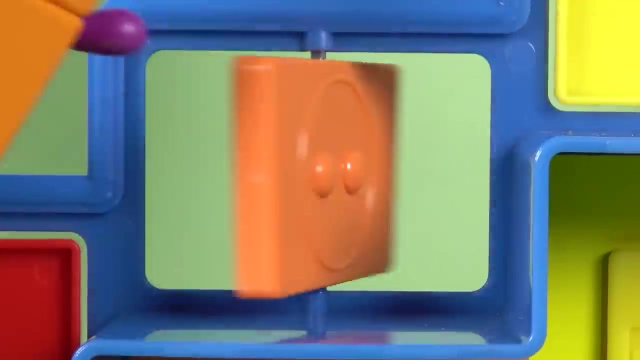 Look, here's Number Block One having fun by the window. She loves to see one big world outside. And here's Number Block Two spinning his number plate. His number plate has two little dots on it. Spin, spin. How funny. 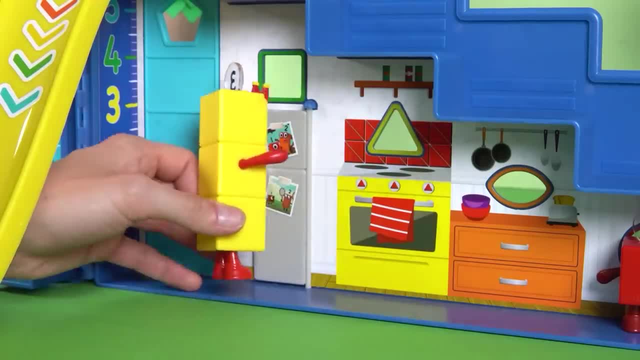 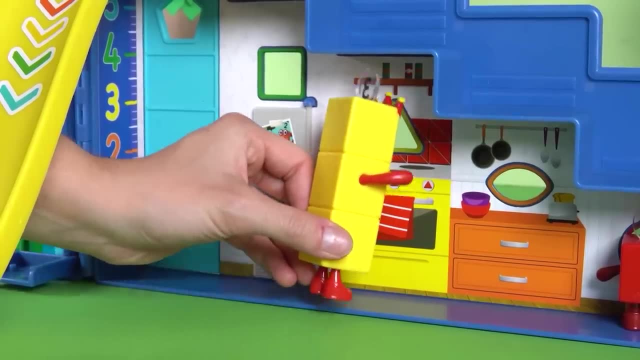 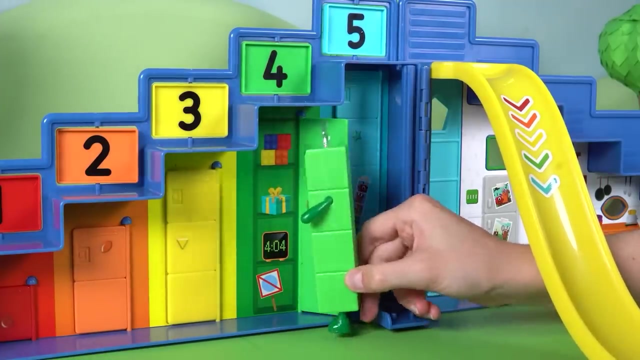 Yummy. Number Block Three is in the kitchen making tasty triangle snacks for everyone. She's having so much fun. Number Block Four is looking at his collection, A collection of square things in his locker. Look, there are four of them. 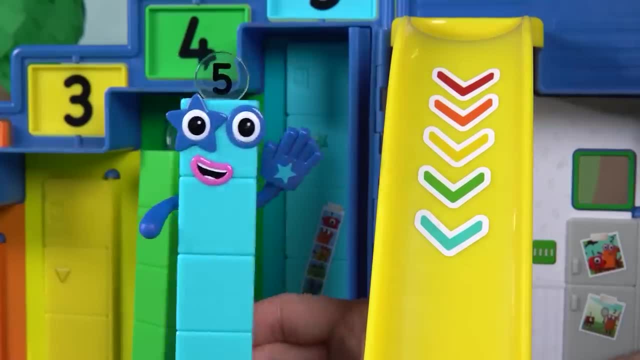 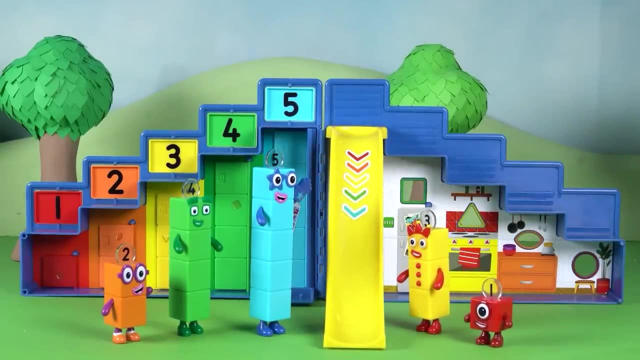 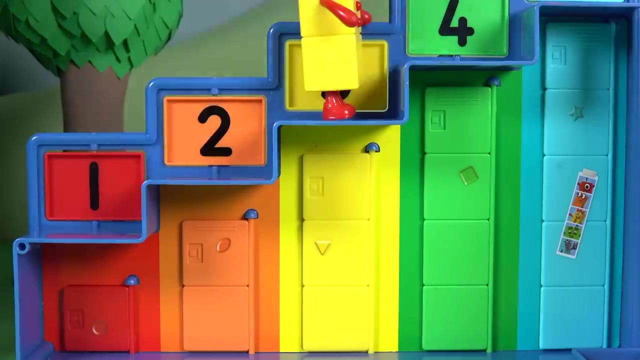 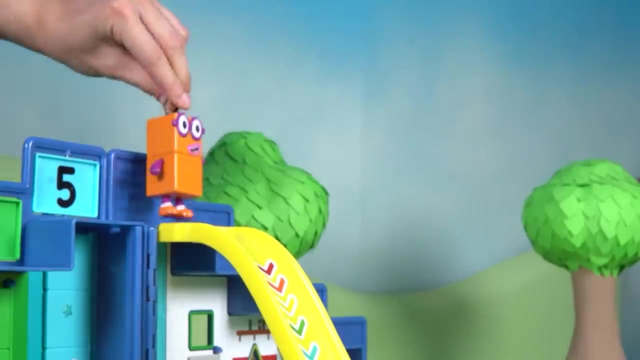 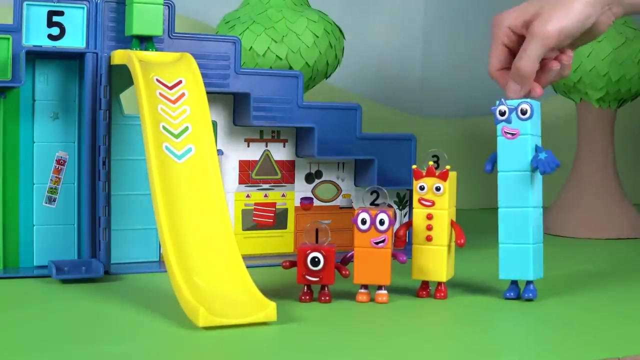 And there's Number Block Five with a big idea. She thinks it's time for everyone to go down the slide. One, two, three and five slide down one by one. Oh no, Who's missing? Of course, it's Four. 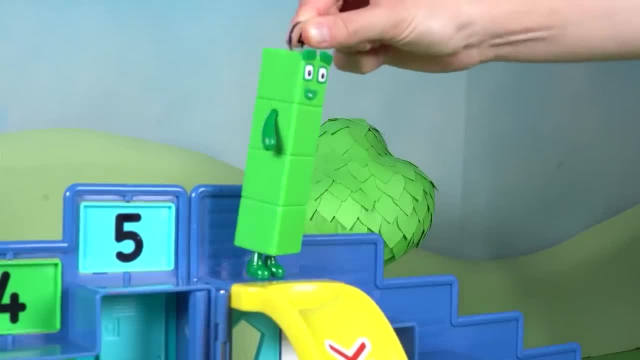 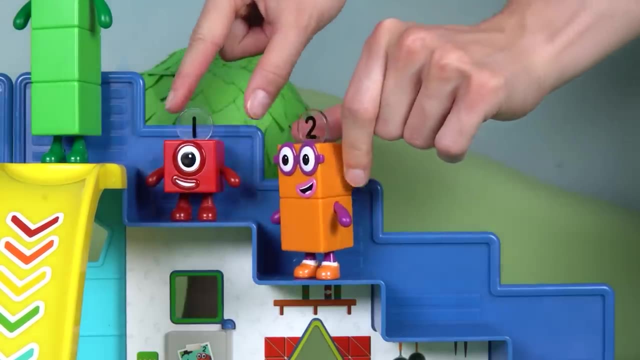 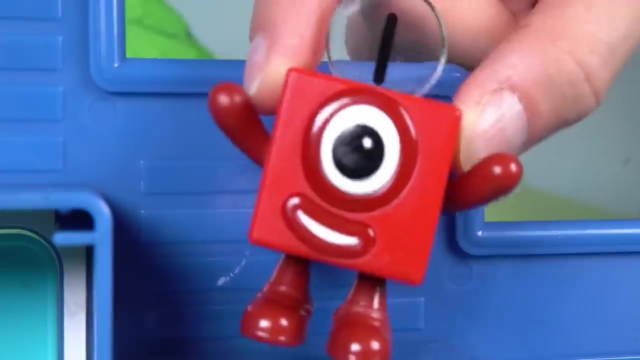 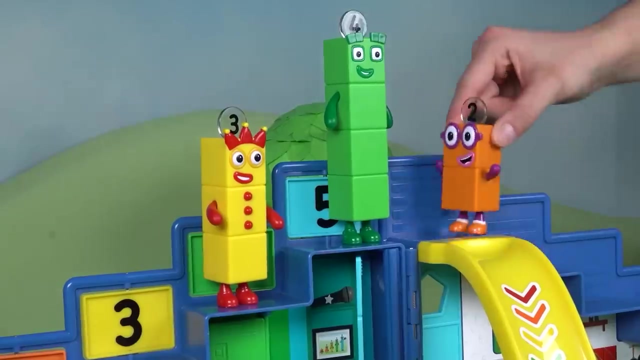 He doesn't want to go down the slide, The other Number Blocks go back up and help him. This looks like a job for Step Squad. Step One: One gives Four a big hug. Step Two: Two shows Four how to slide. Whee. 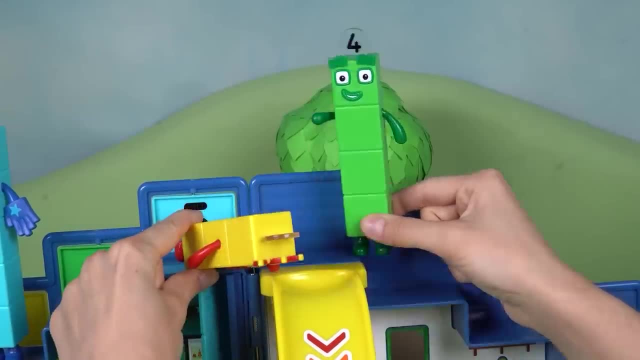 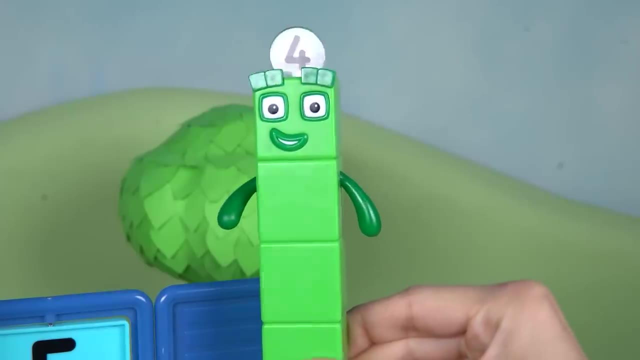 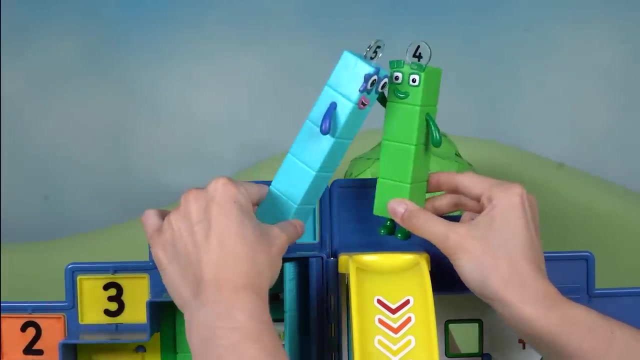 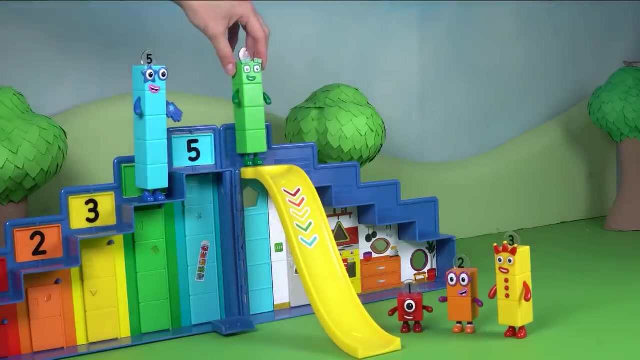 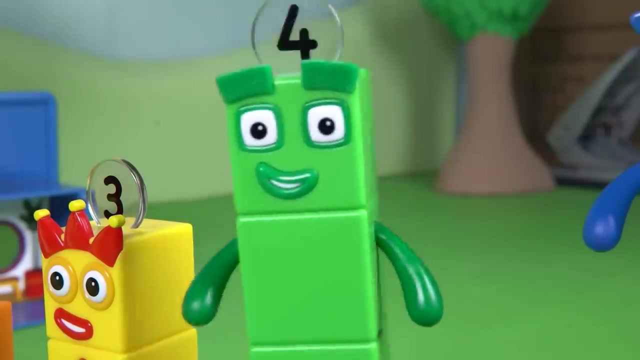 Step Three: Three gets Four to touch the slide. Step Four: Four takes a deep breath. Step Five And Five gives him a high five. He's ready to go. Hooray for Number Block Four And hooray for the super special secret Step Squad. 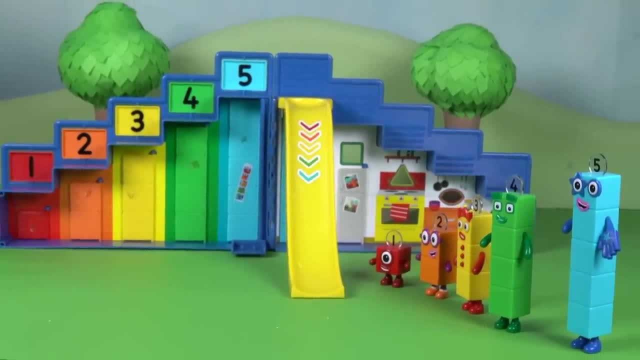 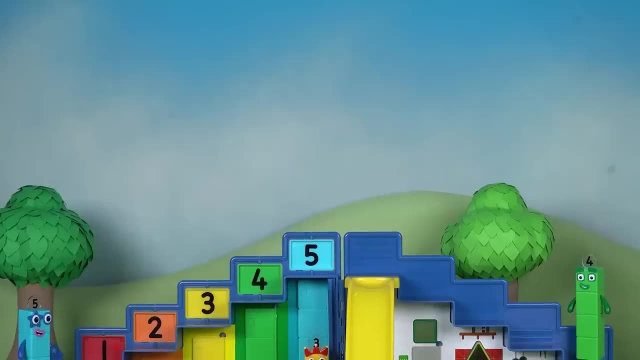 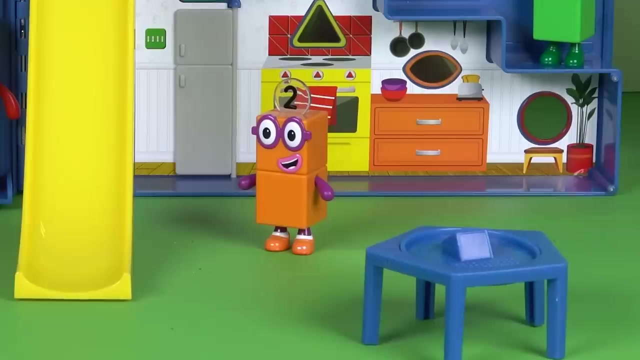 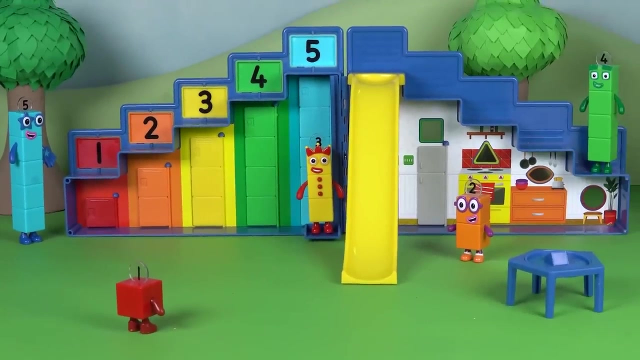 They helped their friend and had a wonderful time. Hello Number Explorers. In the heart of Number Land, the Number Block Step Squad Mission Headquarters is buzzing with Number Blocks One, Two, Three, Four and Five who are busy playing and exploring. 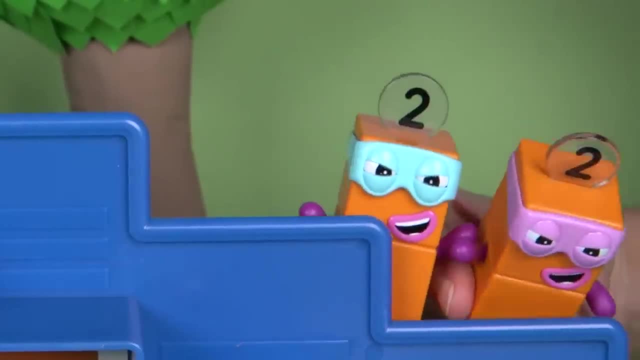 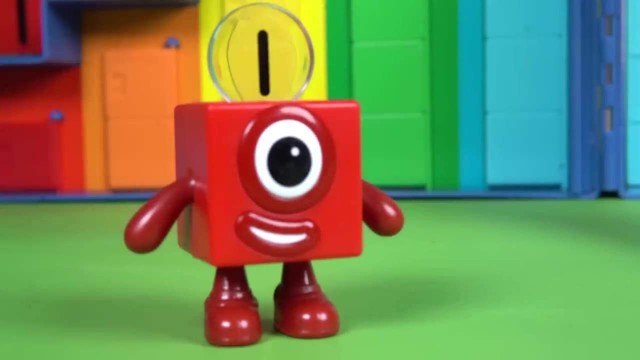 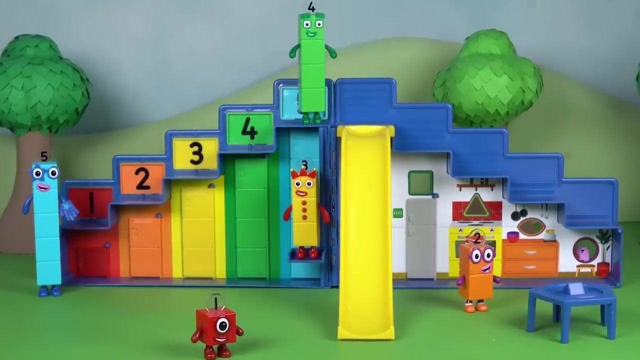 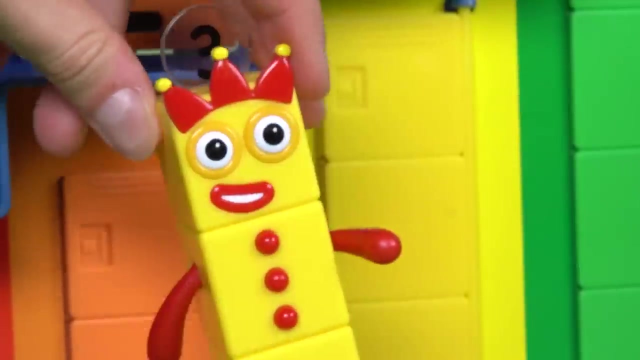 I wonder what adventure we'll imagine today. Wait, What is it? Number Block One. Something is missing. Can anyone think what it is? Haha, They've got it. They're going to decorate the headquarters. It's time to make it bright and fun, just like them. 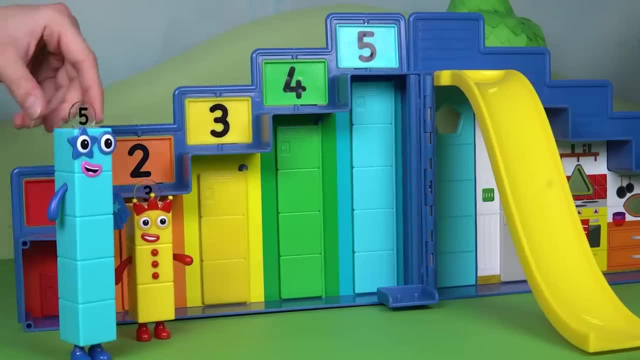 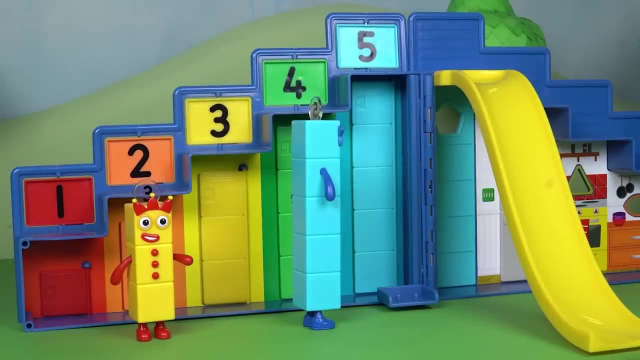 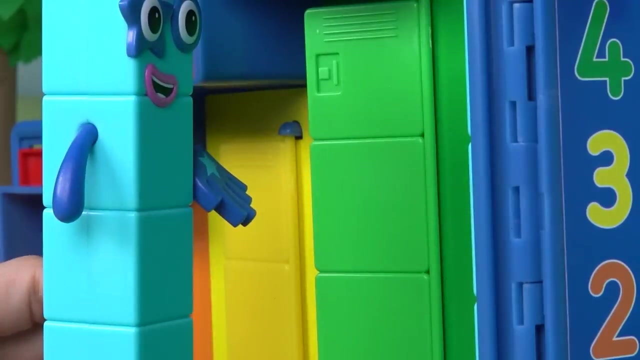 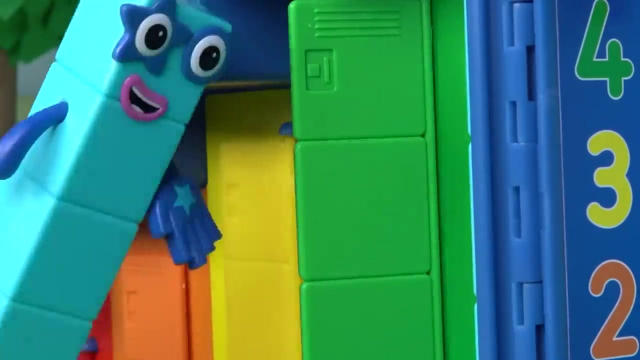 Number Block Five knows exactly what she needs to brighten up these headquarters. The Number Blocks are all set to decorate. Number Block Five, the tallest of them all, goes to the locker to find the sticker sheet. She looks in Four's locker and finds the sheet. 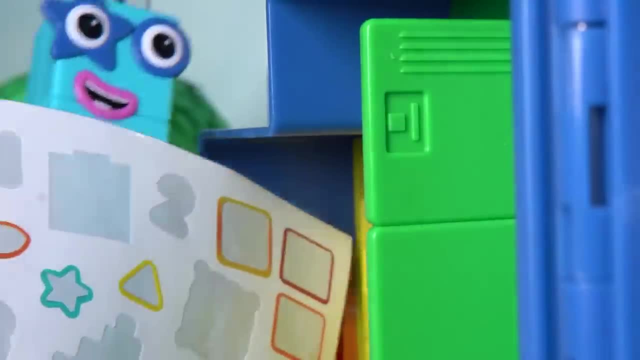 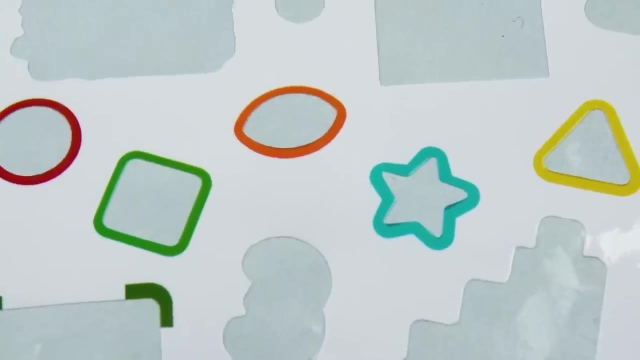 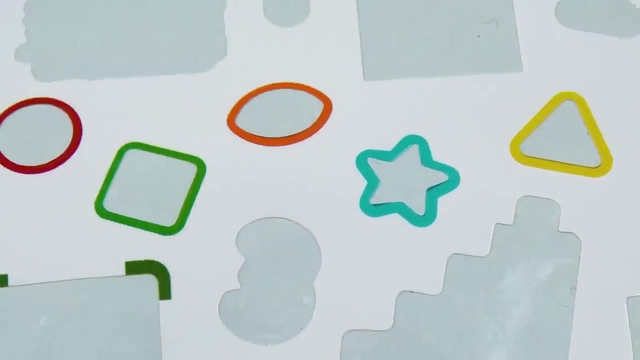 The day is saved. Uh-oh, Number Block Five stops and looks at the sticker sheet. Something's not right. She turns the sheet this way and that way, But it's not quite right. Oh no, All the stickers are missing. 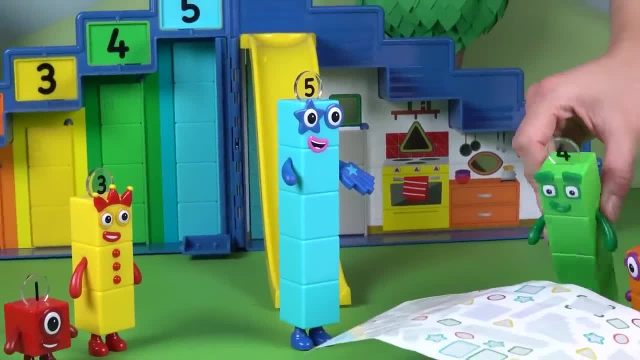 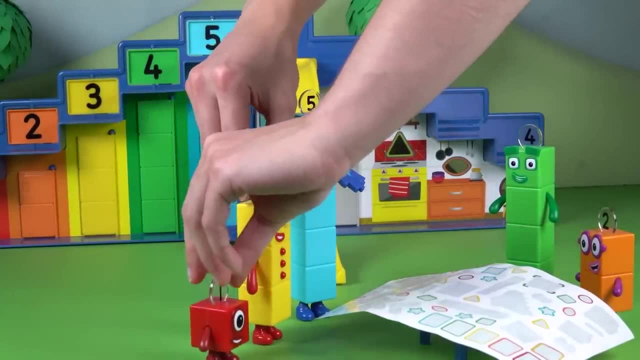 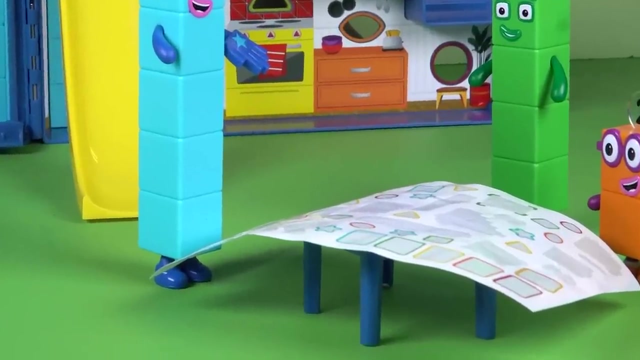 Where could the missing stickers be? They wanted to make the headquarters even more bright and colorful. What will they do now? How will they find the missing stickers? It's a job for the Step Squad. Aha, They've got it: The Terrible Step Squad. 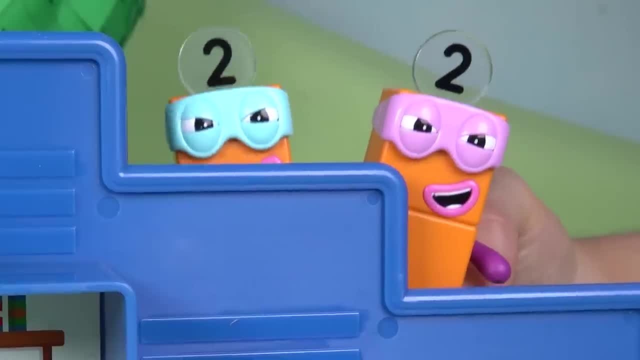 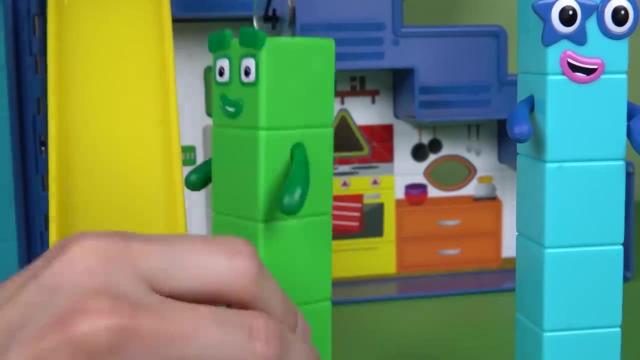 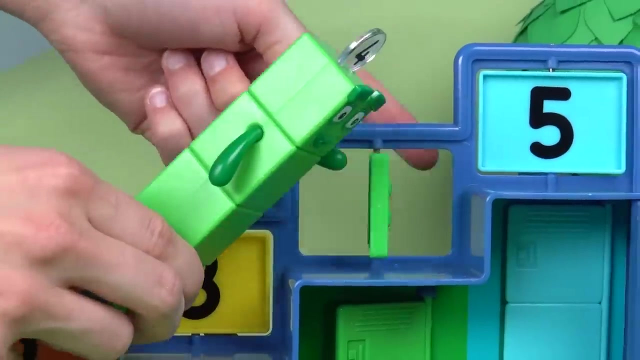 The Terrible Step Squad, The Terrible Twos, must have taken the stickers and hidden them somewhere. It's time to find those missing stickers. The Number Blocks are on a mission. They search high and low, spin the number plates and peek through the lockout windows. 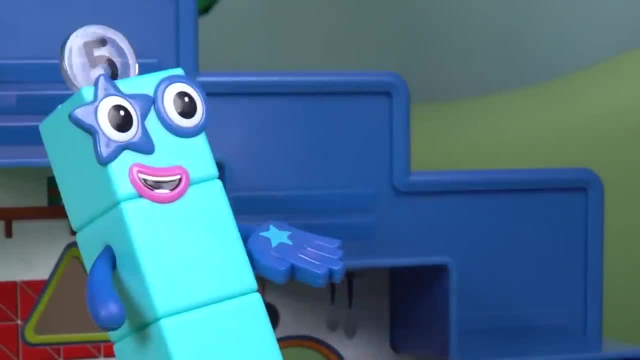 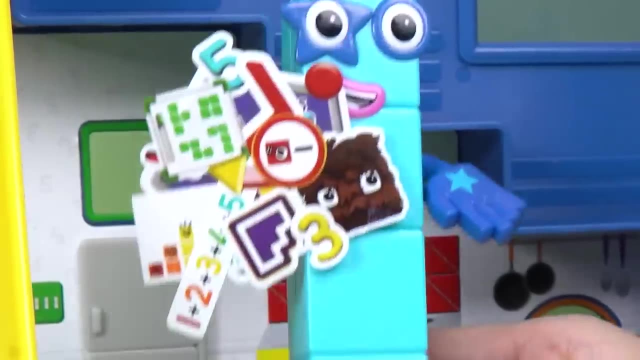 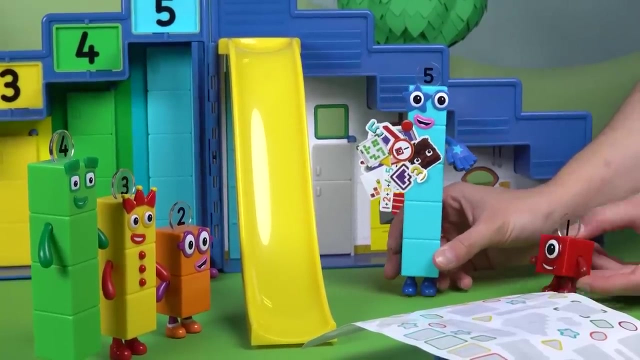 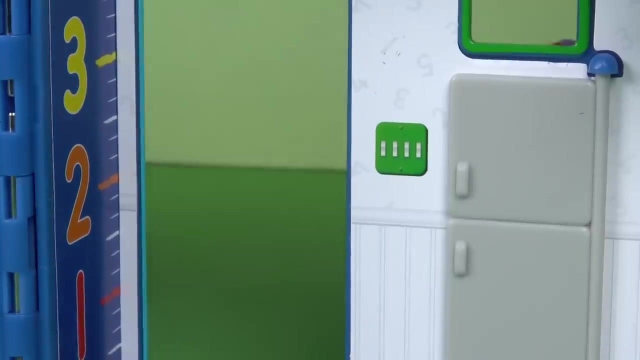 But wait, Five stops near the slide. She looks down and gasps: Could it be? Hooray, Number Block Five found the missing stickers. They were under the slide all along The Number Blocks cheer and high-five each other. They've solved the mystery and found the missing stickers. 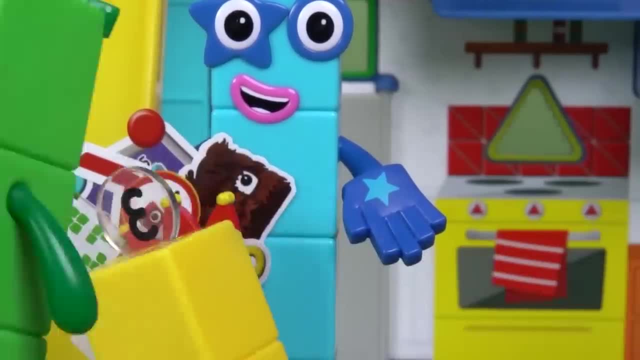 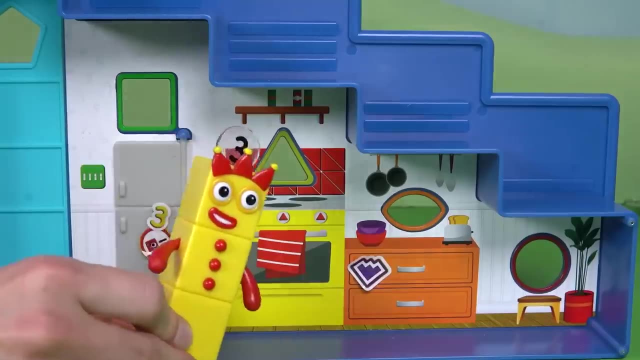 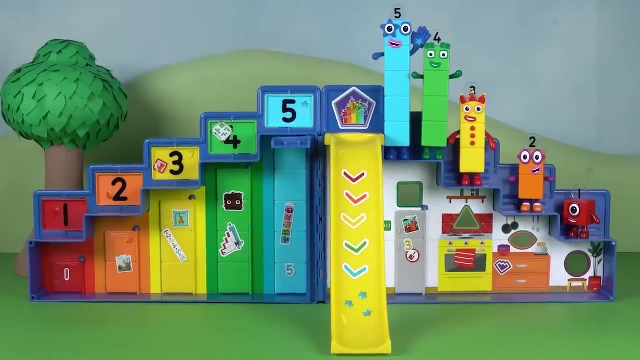 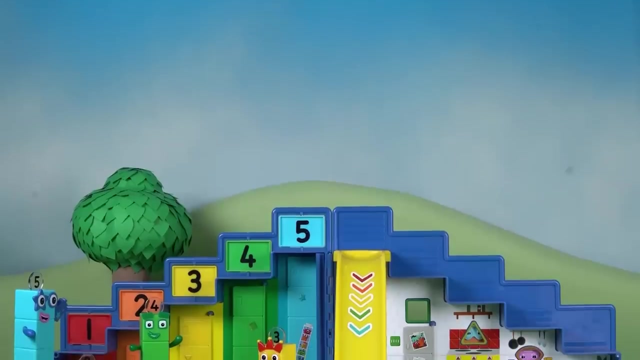 Now they can finally decorate their headquarters and make it bright and fun, And so the day is saved. thanks to the Step Squad, They've turned their headquarters into a wonderful sticker set. Hello Number Explorers, and welcome back to the Number Blocks. Step Squad- Mission Headquarters. 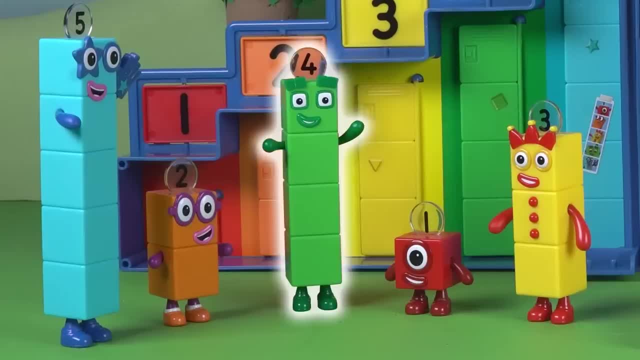 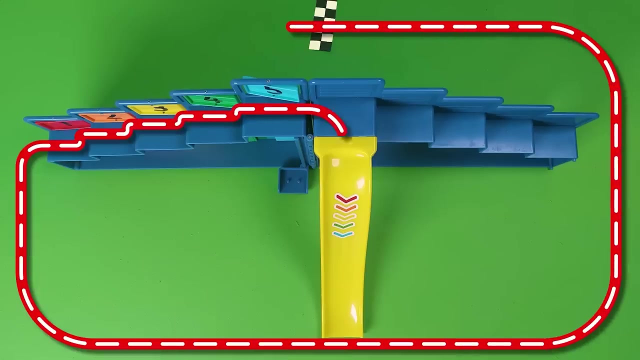 Where Number Blocks One, Two, Three, Four and Five are busy getting ready for a fun day of Number Exploration. Number Blocks Two, Three, Four, Five and Six are on their way to the headquarters, But they have a trick up their sleeves. 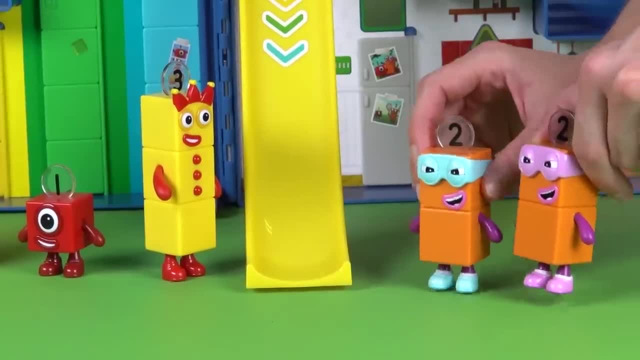 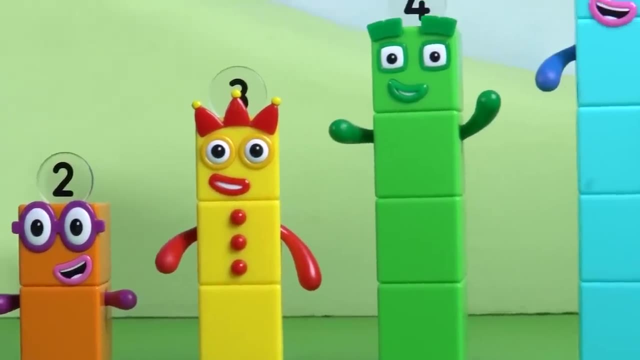 Everybody is getting excited about the race. They line up at the big blue door ready to run On your marks. get set, go. The Number Blocks are racing. They go past the colorful number blocks. Number Blocks One, Two, Three. 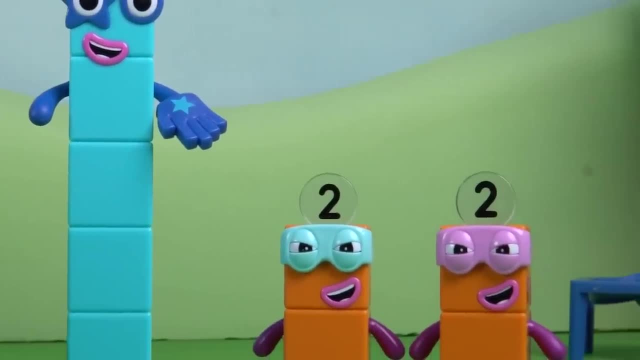 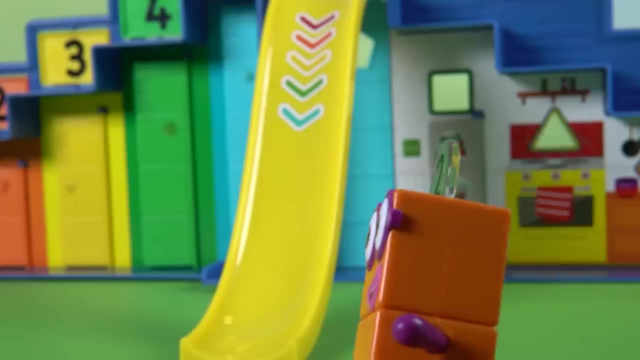 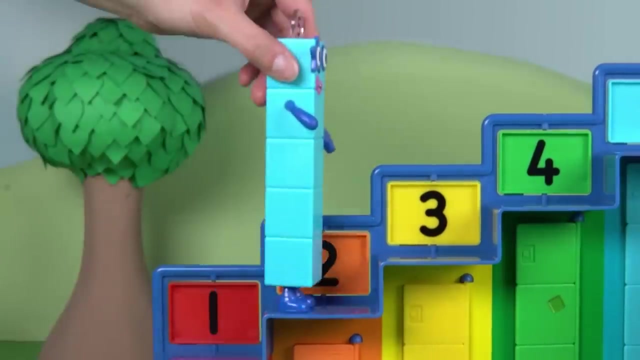 Four, Five and Six Number Blocks Two, Three, Four, Five and Six. They go past the colorful kitchen, around the big slide, past the lockers and up to the stairs. Here they go, jumping up up. 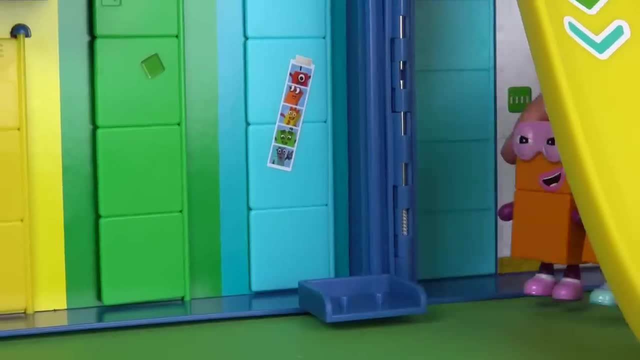 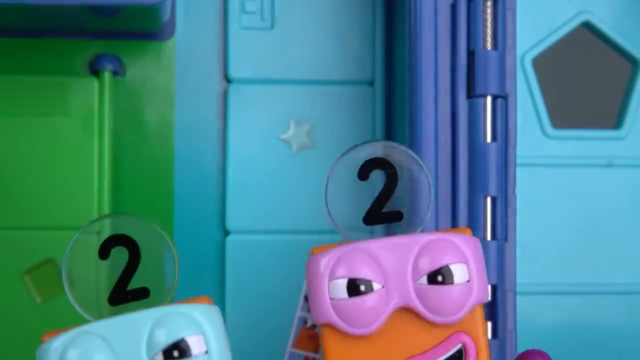 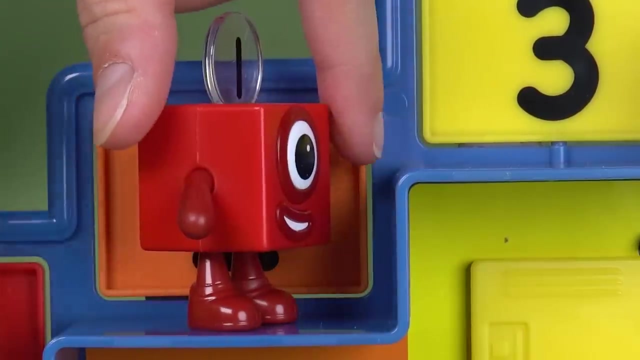 up the stairs. But wait, Where are the terrible twos? The terrible twos are using the lift to go up instead of the stairs. Where, Oh no, Will the other Number Blocks see them? The terrible twos have reached the top. 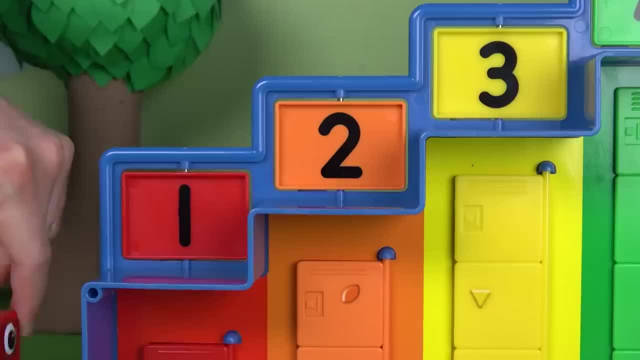 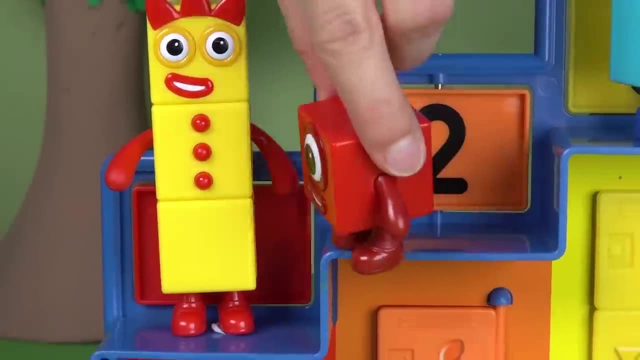 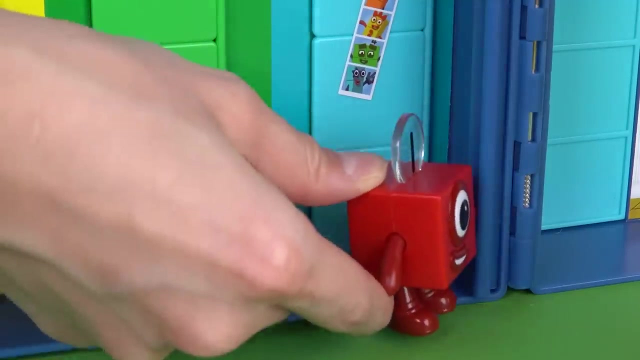 But the race is not over yet. The Number Blocks are still trying to reach the top. The terrible twos think they're going to win, But the Number Blocks have a plan. Look at One. She sent the lift back to her. The terrible- 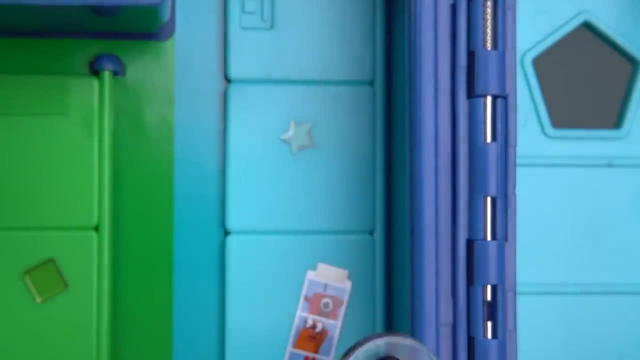 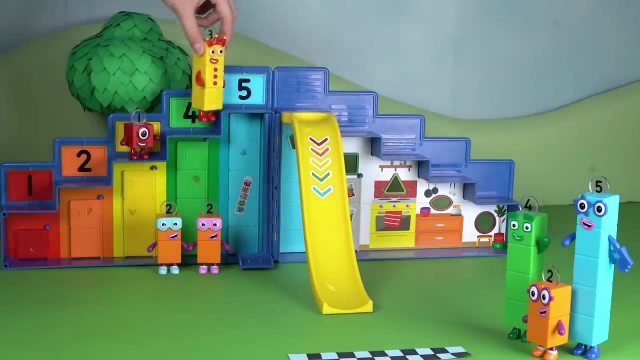 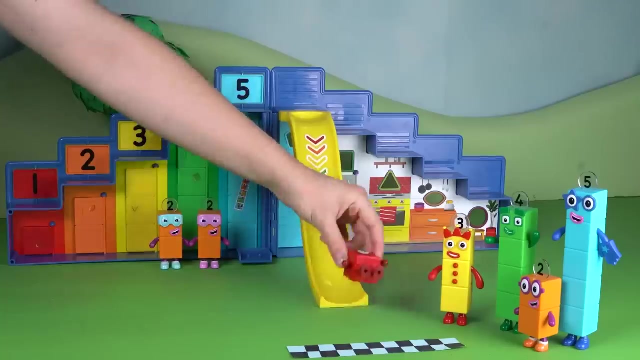 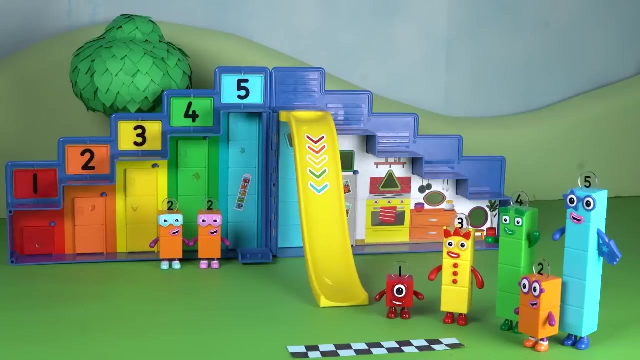 twos are surprised and don't know what to do. And the Number Blocks have done it: They've won the race. fair and square, That was close. Ah, what a fun day at the Number Blocks Step Squad Mission Headquarters. So Number Explorers. 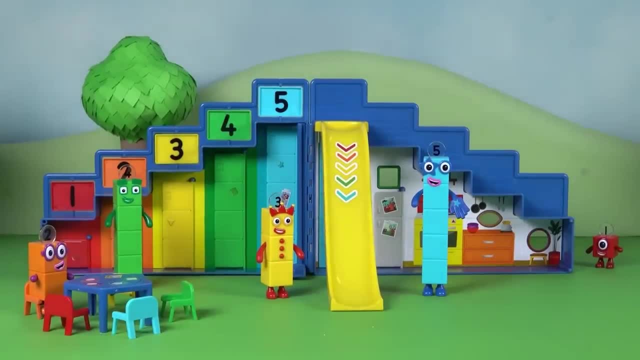 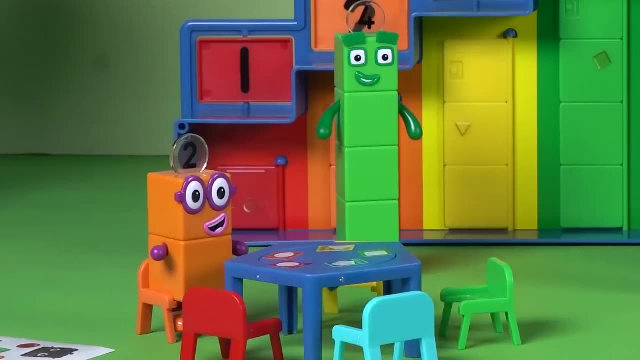 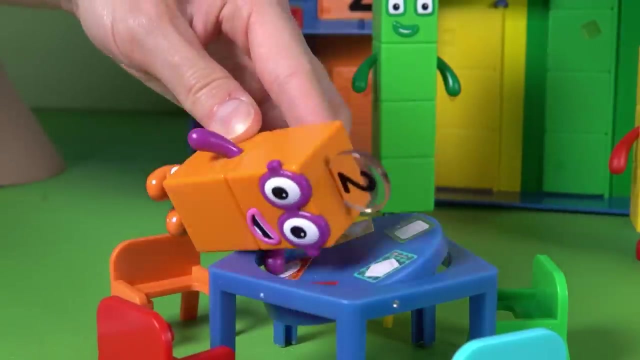 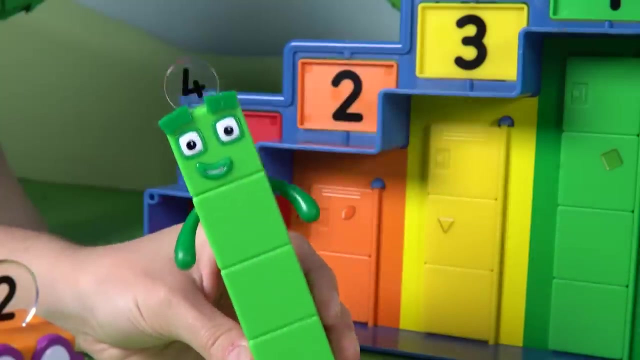 ready for another adventure. Let's find out what's being imagined today at the Number Blocks Step Squad Mission Headquarters. Oh look, our Number Block friends are all together. Something's not quite right. They can't decide what to do today, But wait. 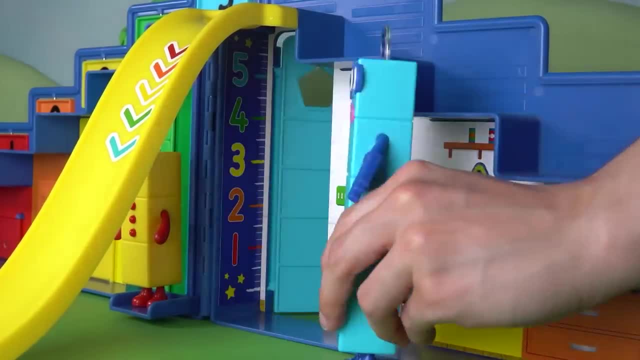 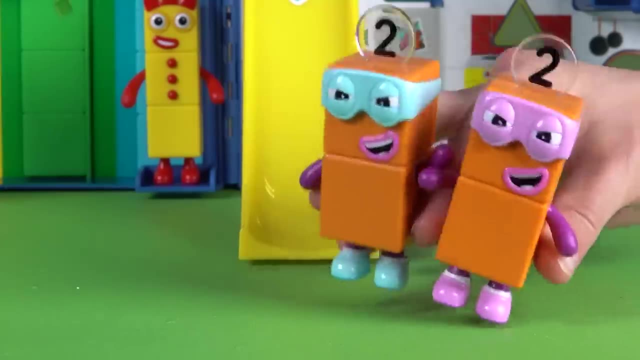 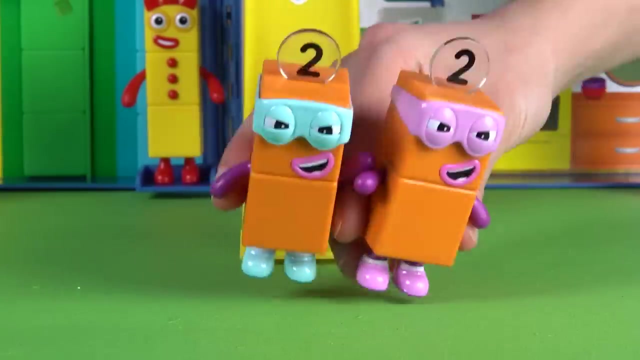 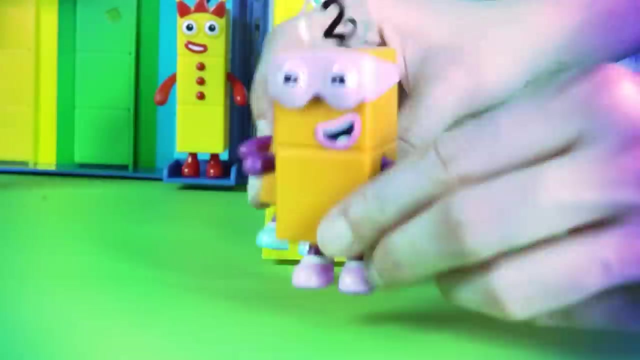 what's this? It's the terrible twos. They've arrived and they're full of mischief. They bounce around the room waving their arms up and down. Oh, it looks like the terrible twos have a challenge for our day. Well, 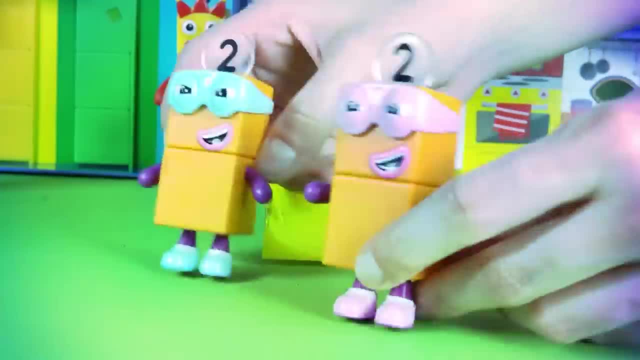 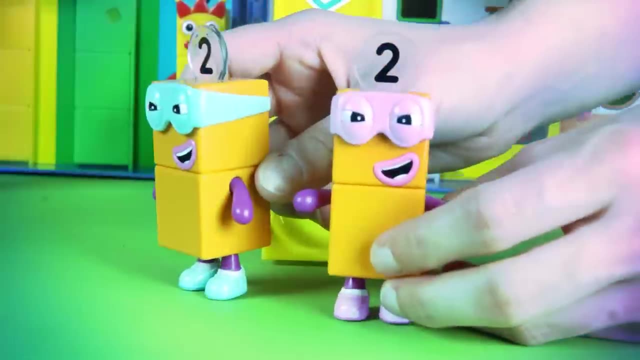 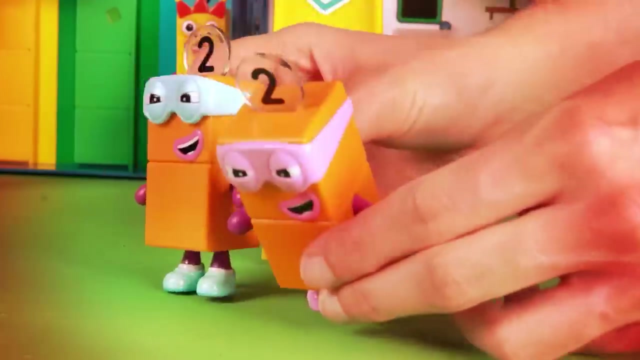 this is going to be fun. The Number Blocks are ready and the terrible twos can't wait to show off their moves. Look at the terrible twos go With their arms moving up and down. they dance and twirl, trying to impress. 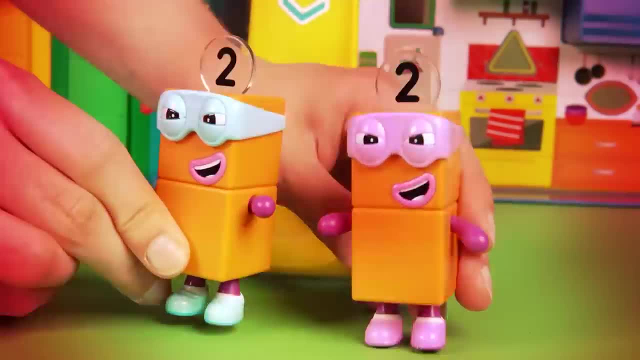 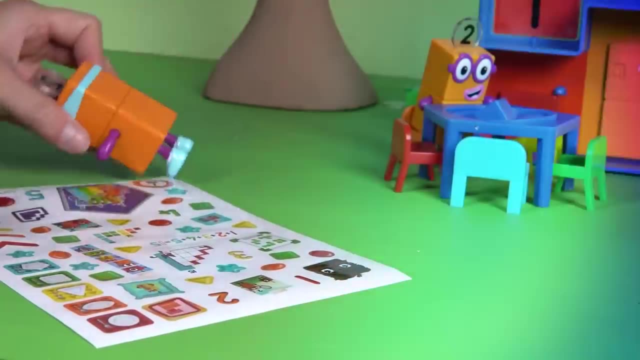 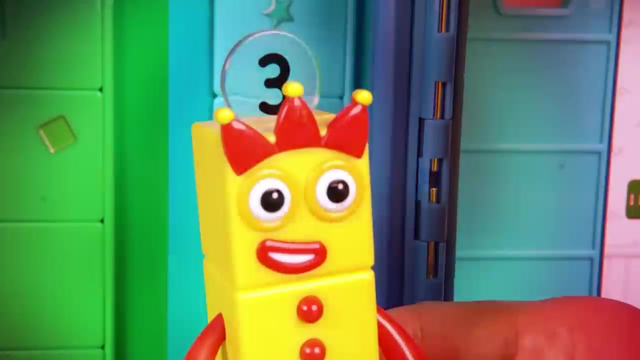 everyone with their moves, But wait, what are they up to? One distracts the other is trying to snatch the stickers. Three's having so much fun she doesn't even see what's happening right under her nose. And five, she's getting. 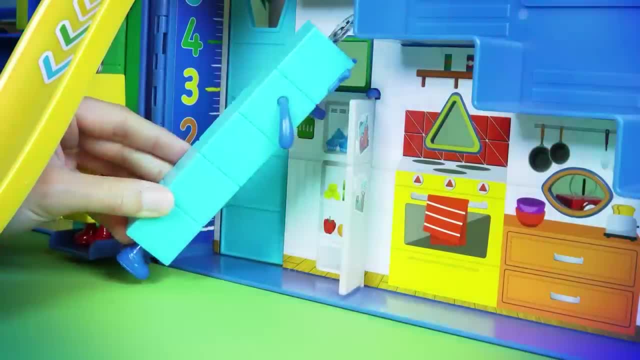 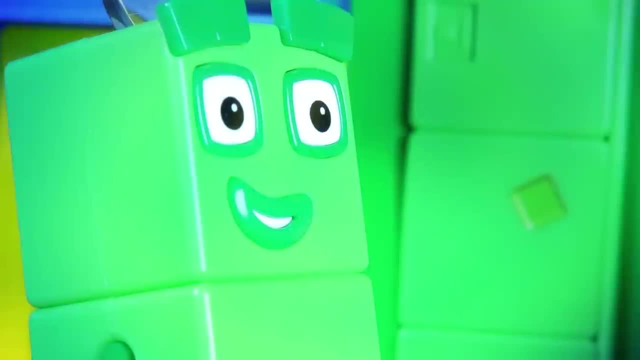 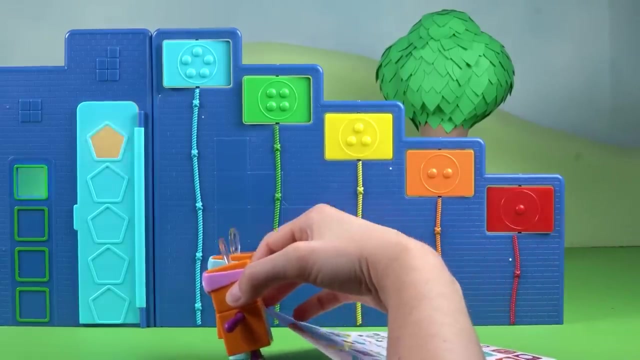 snacks ready for everyone. Dancing really does make you hungry. Oh no, the terrible twos have some of the stickers Time and time. Shh, the terrible twos think they're so clever sneaking away with the stickers, But little. 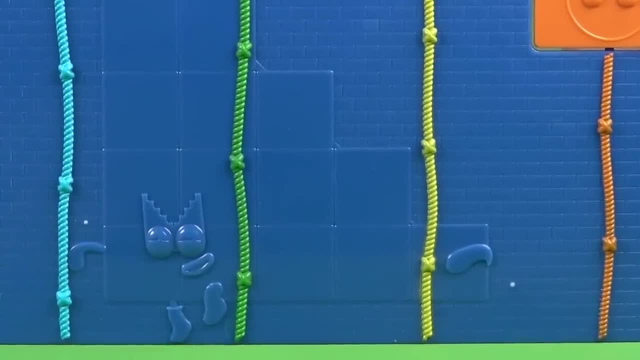 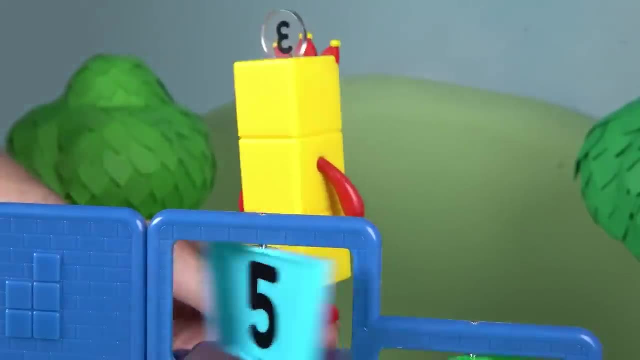 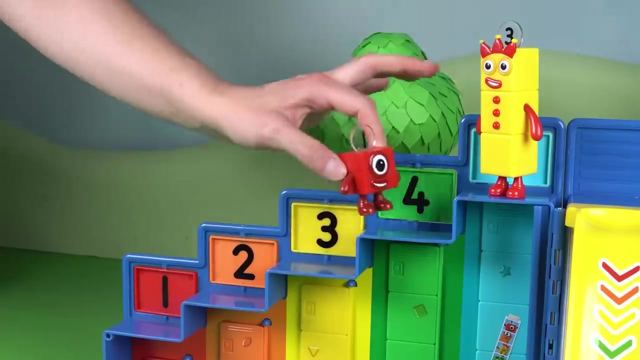 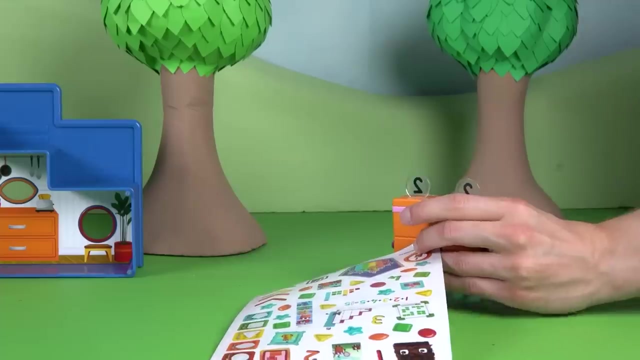 do they know? someone is watching Hush hush. Oh, what's this? A signal from number block 15.. She's trying to tell the step of the day. Ha ha, caught red-handed thanks to number block 15's. 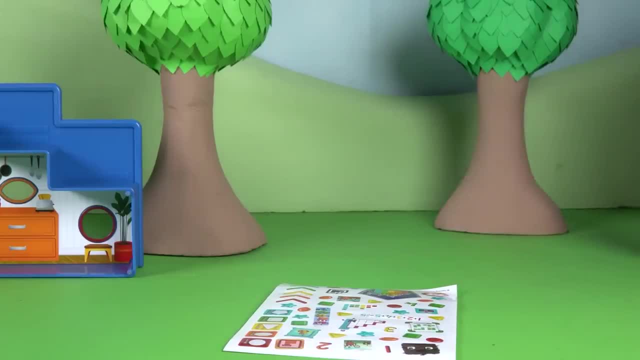 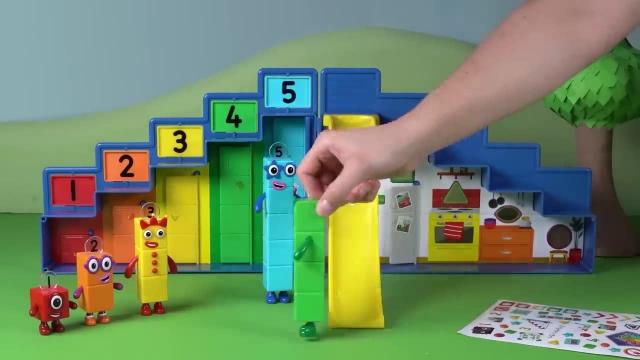 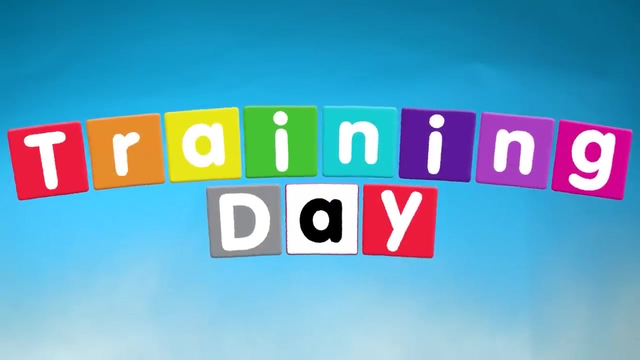 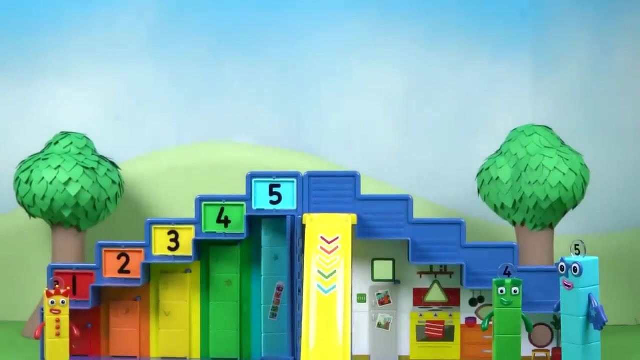 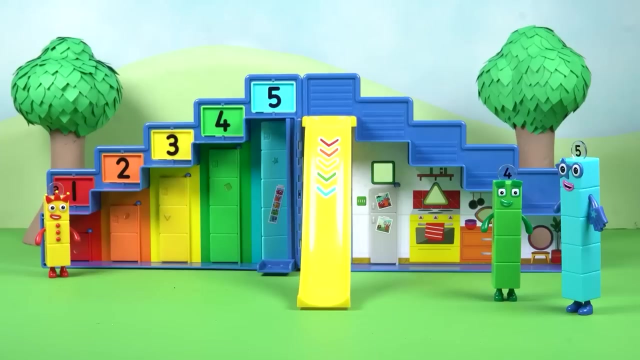 alert, And so the day is saved, all thanks to the watchful eyes of number block 15 and the teamwork of our favourite number blocks. It's a sunny day and inside the number block step squad mission headquarters, number blocks 3,. 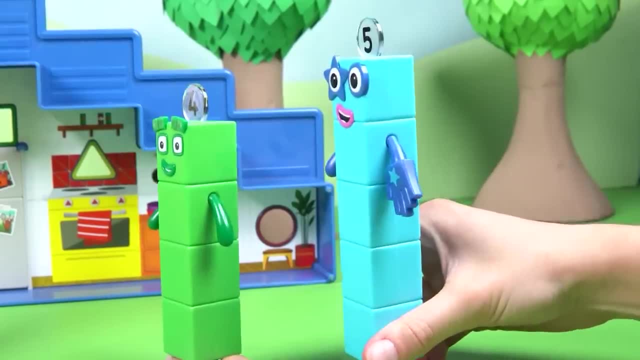 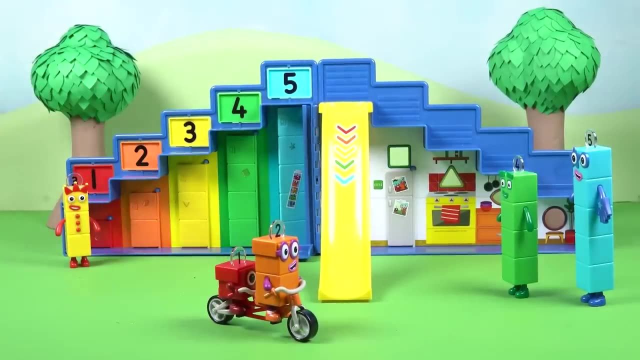 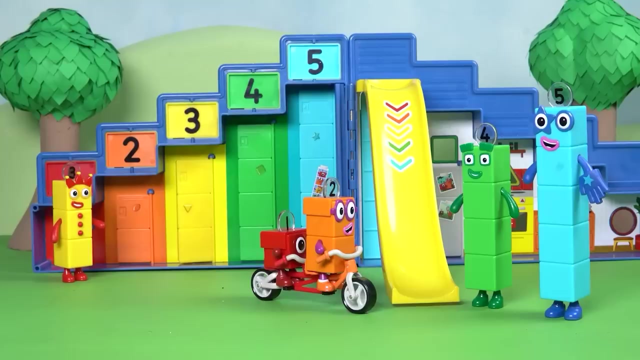 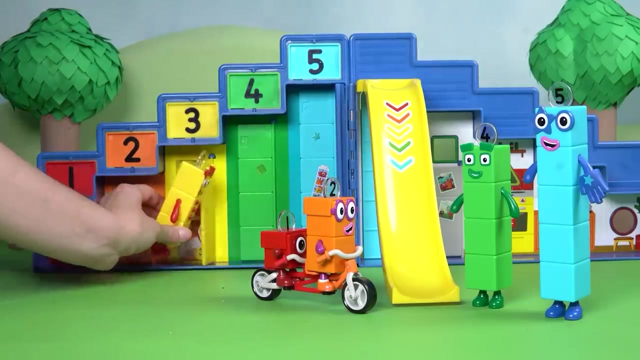 4, and 5 are having a lovely time. What's that sound? Could it be? It's number blocks 1 and 2.. And look, it's the number block 3.. Ha ha, number block 3 has an. 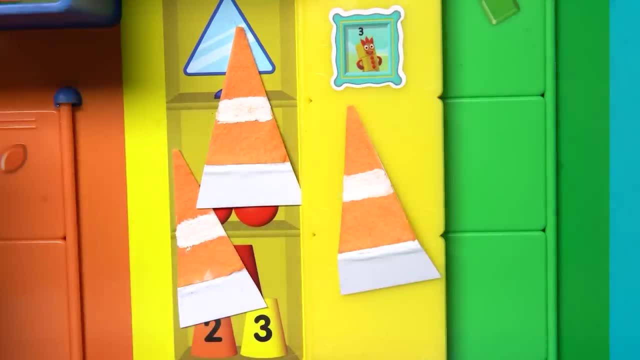 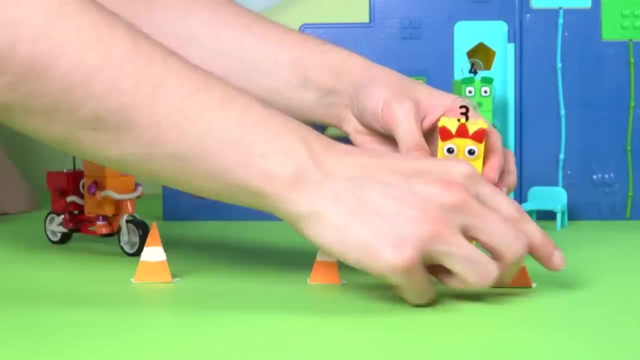 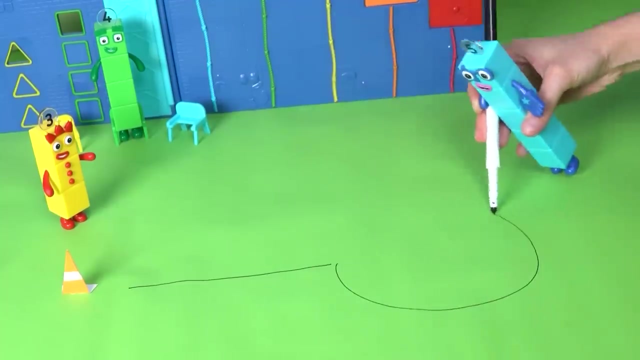 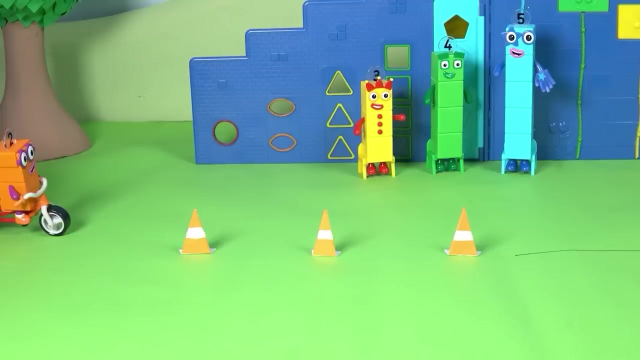 idea. What could those orange cones be for? Looks like our step squad is setting up a training course for four. Oh, riding in a circle, That's a fun challenge. All right, little number blocks. first up the zigzag challenge. 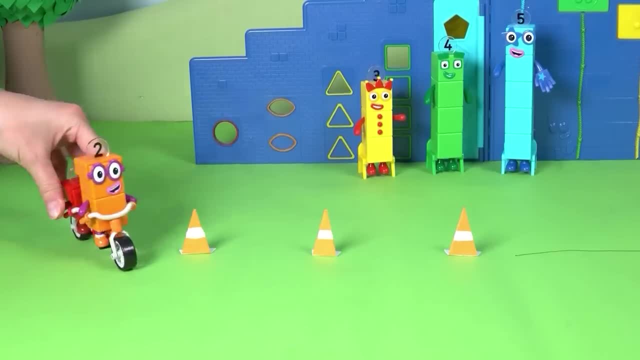 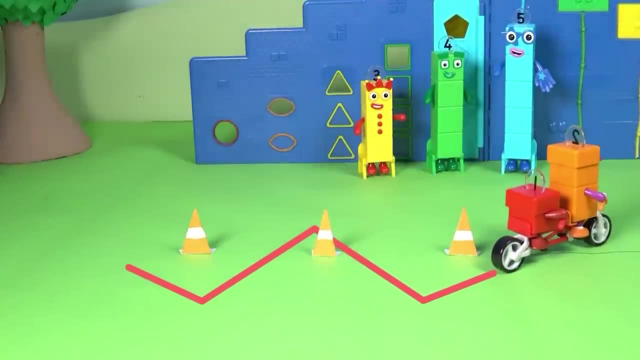 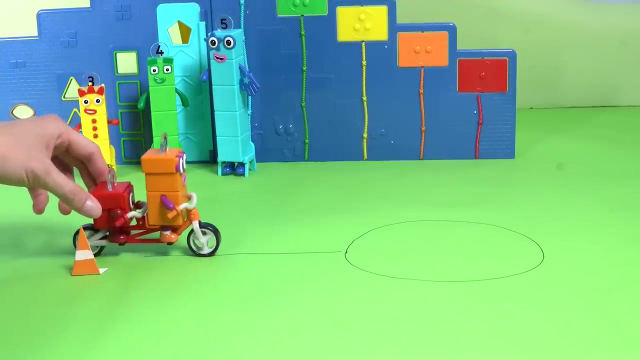 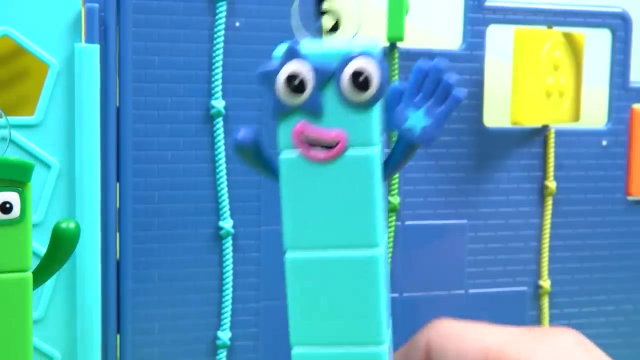 Can our dynamic duo navigate through without knocking any cones? Look at them: go zigging and zagging. Now let's see if they can follow the line. Stay steady: number blocks. That's it. Follow the line You're doing. 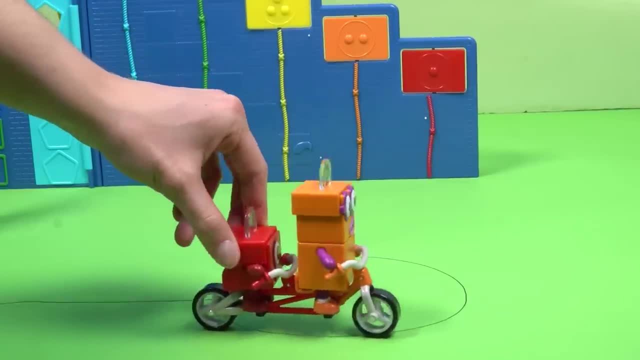 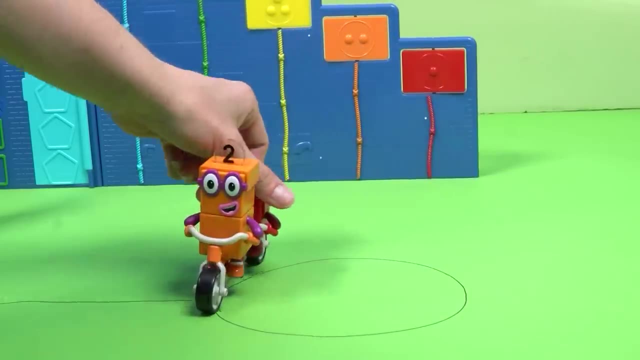 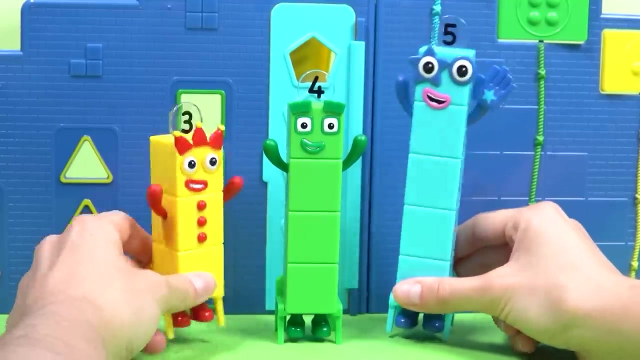 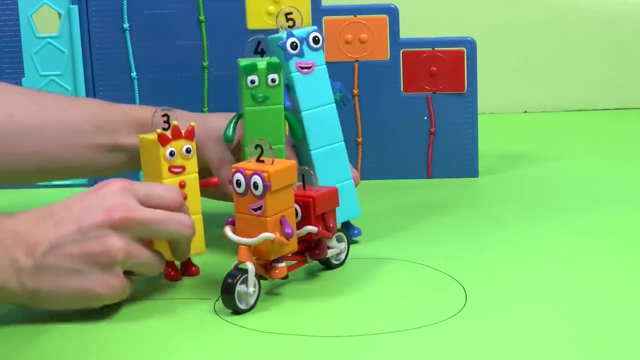 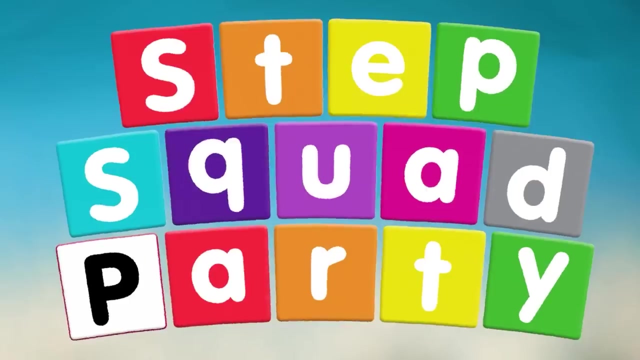 brilliantly And for the grand finale, riding in a perfect circle Round. they go all the way around the circle. Number blocks one and two have shown us some impressive riding skills today. What a wonderful day we've imagined, with so much fun at the. 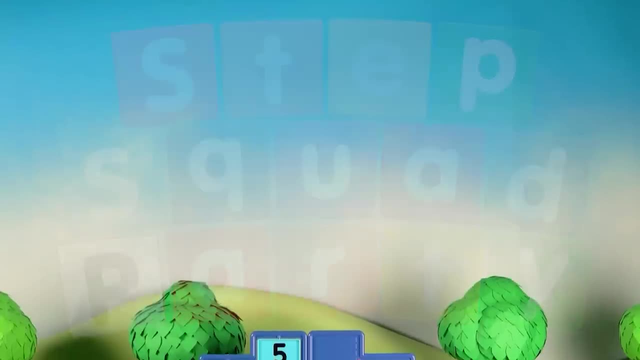 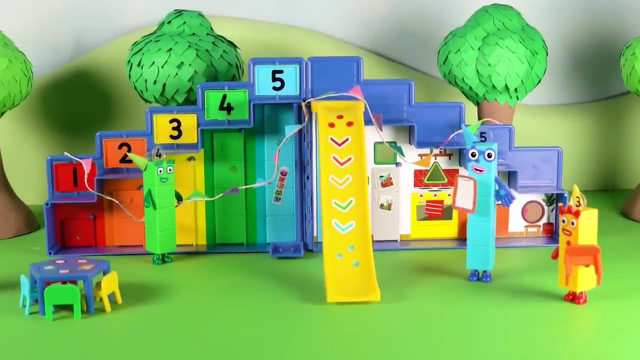 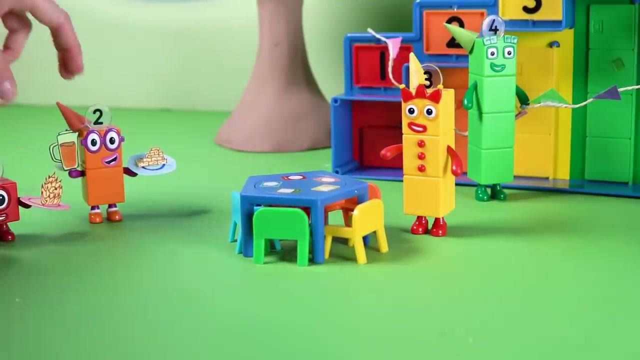 Step Squad Mission Headquarters. Hello number explorers, It's a bright and sunny day today. Our number blocks are buzzing with excitement. Let's find out what story we're imagining today. Number block three is getting everything ready. It looks like they're. 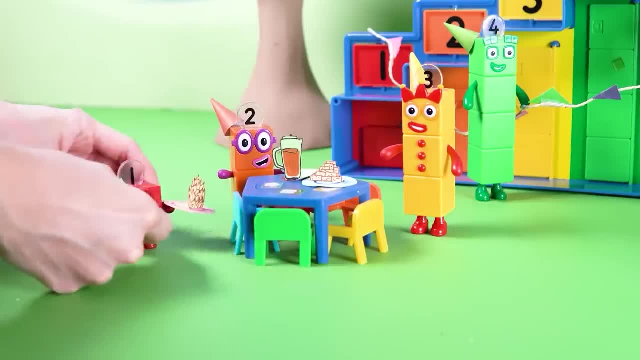 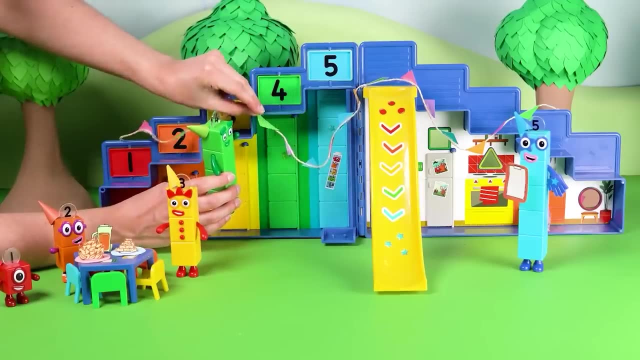 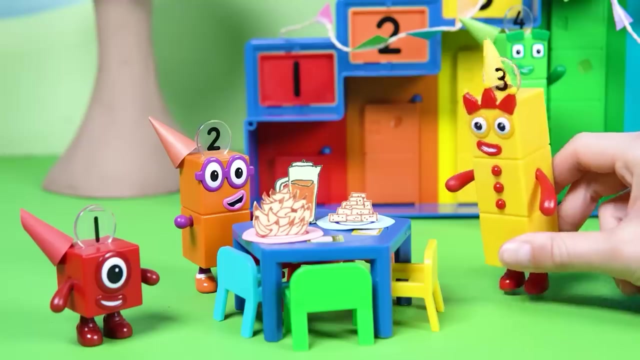 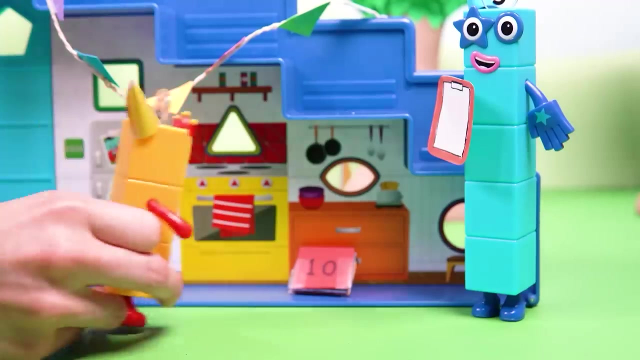 planning a party. Number blocks one, two, four and five are helping out too. Everyone's working together. Number blocks six, seven, eight, nine and ten to join them. Oh dear. Number block three looks worried. I wonder what's on. 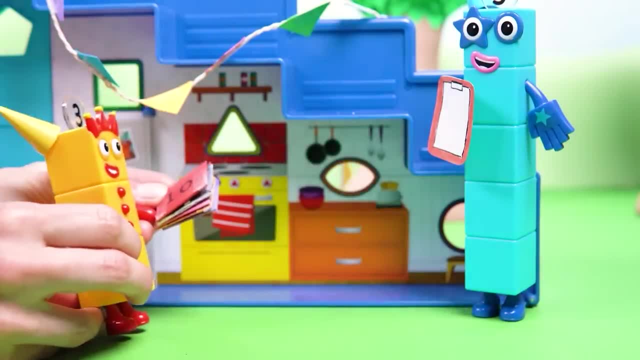 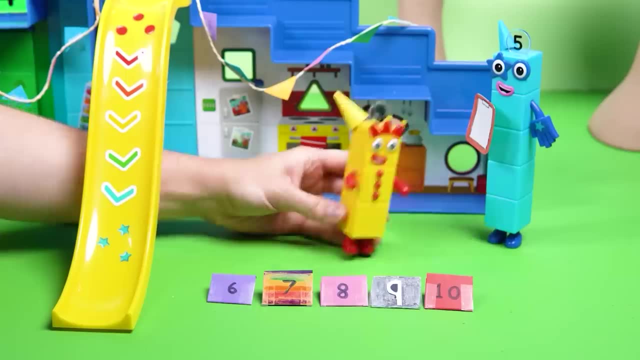 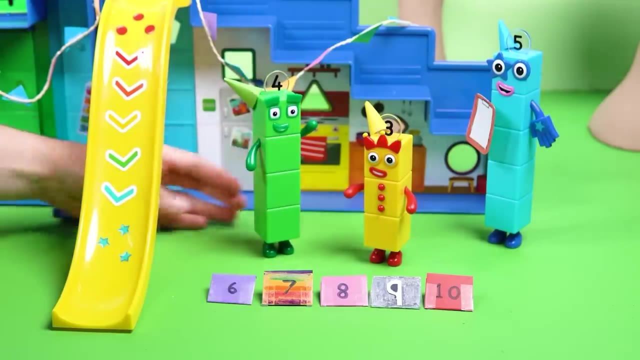 her mind Whoops. It looks like three forgot to send out the party invitations to number blocks six, seven, eight, nine and ten. Oh no, Four is getting everything ready. What can they do? Great idea two, One and two can. 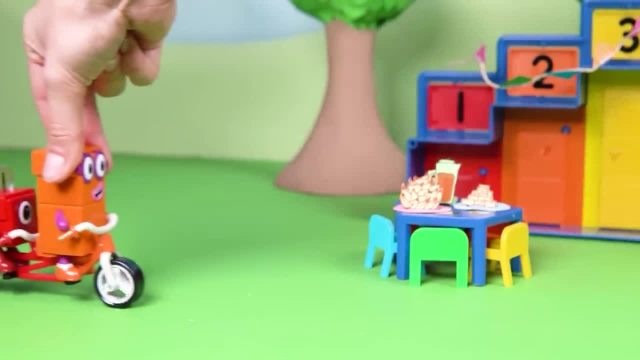 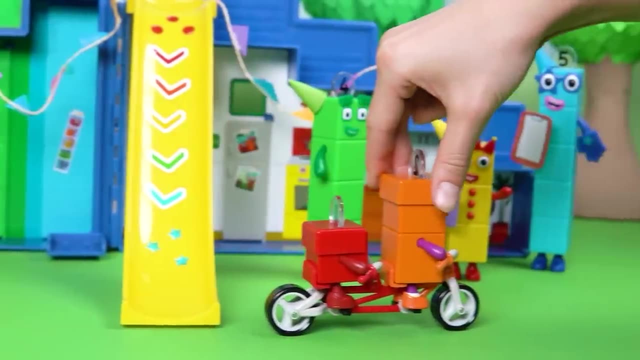 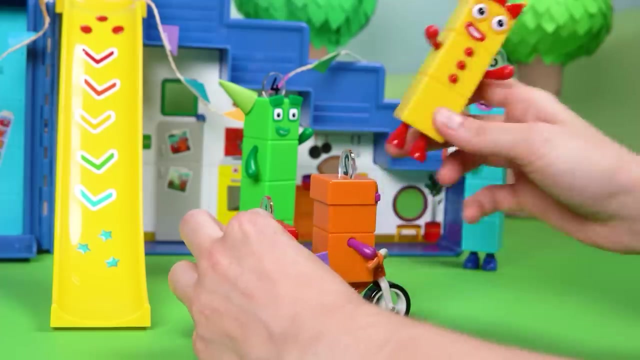 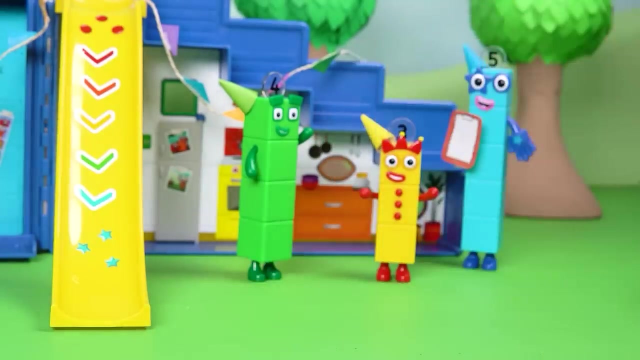 quickly deliver the invitations on their bike. It's much faster than walking. One and two are always ready for an adventure and today they have a very special mission Off they go riding together to help the party. Let's hope they make it in time. 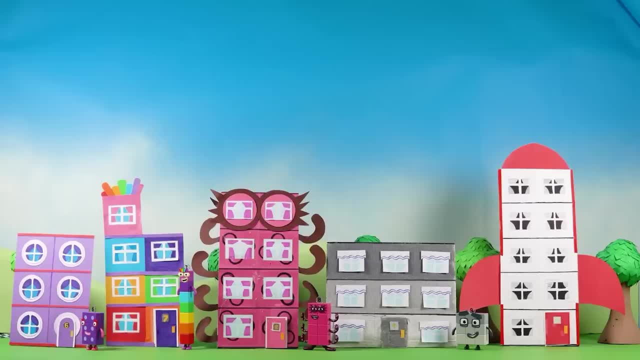 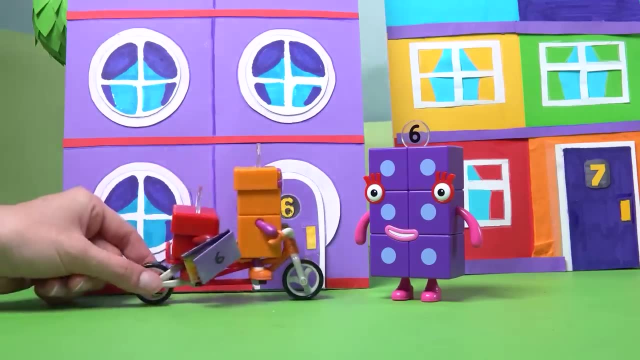 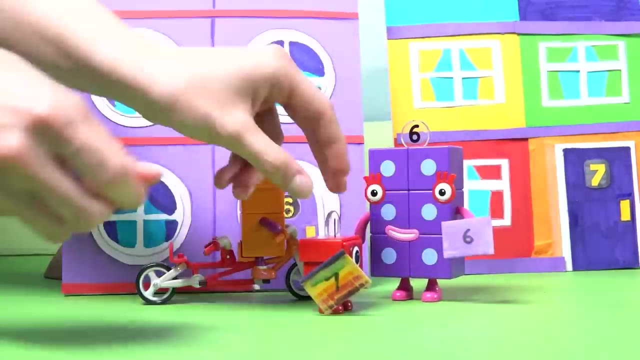 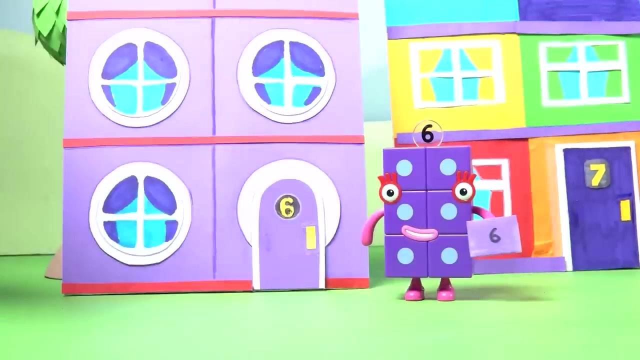 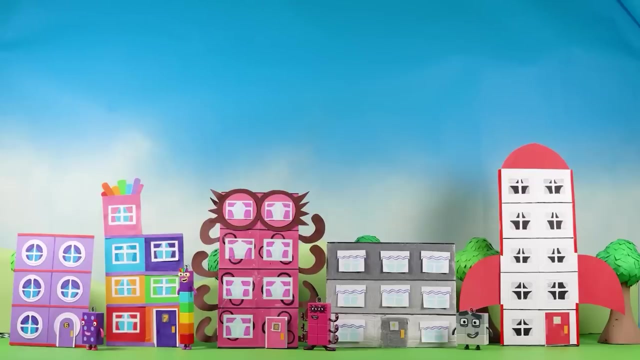 First stop, number block six's house. It has six round windows, just like her dice pattern. Oh yay, Six. got the invitation. Right Now on to the next house. Look at that. Number block seven's house has seven rainbow colours. Let's deliver. 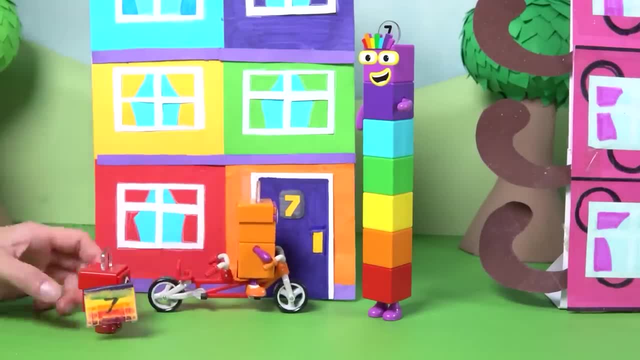 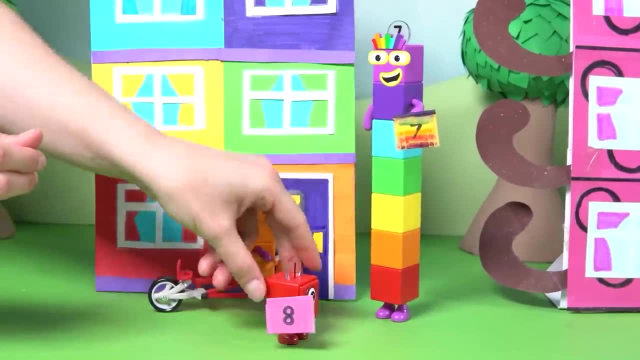 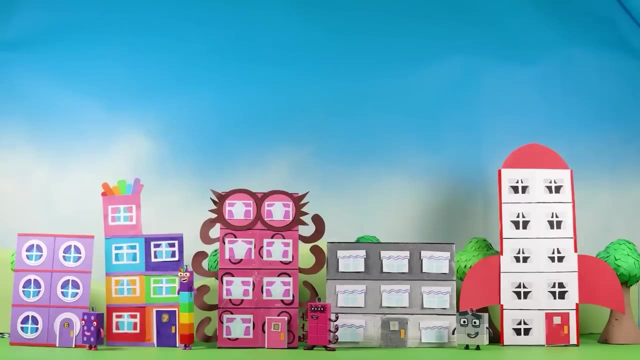 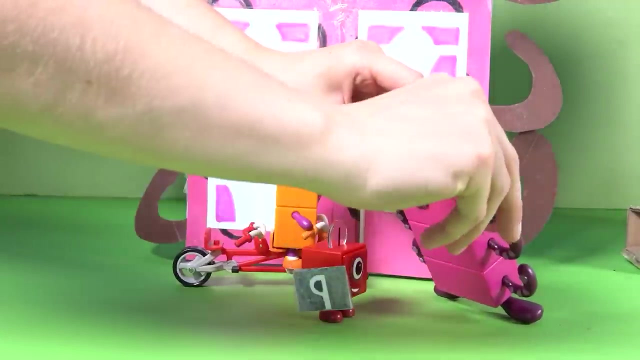 the next invitation. Oh, seven is thrilled and jumps with excitement. Now we're off to eight's house. Eight's house has one, two, three, six, seven, eight tentacles on it And look, eight is home. Here's nine's. 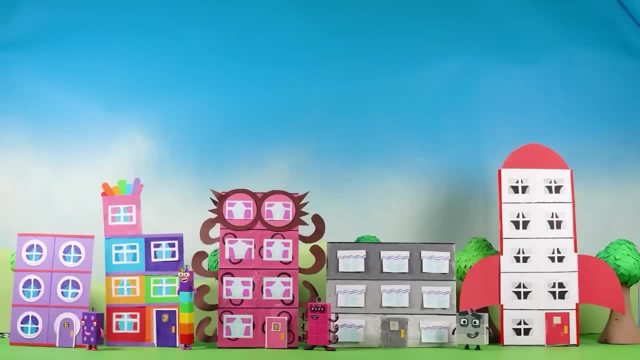 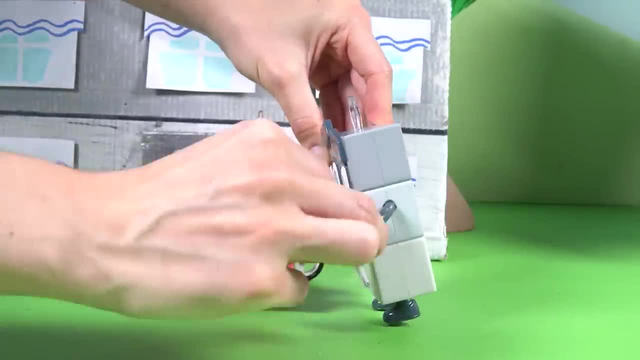 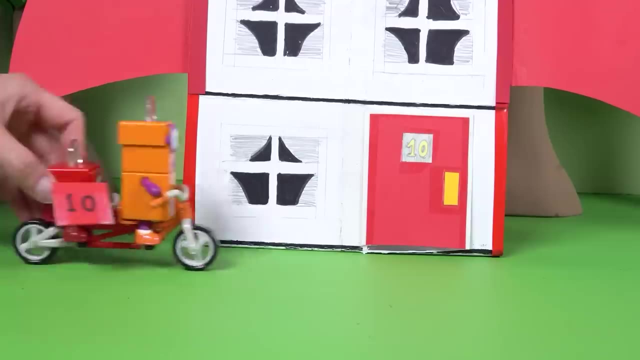 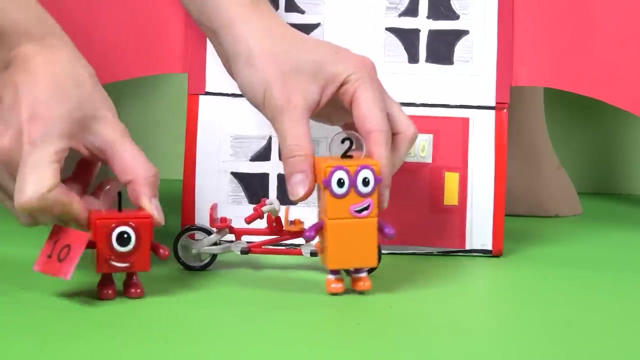 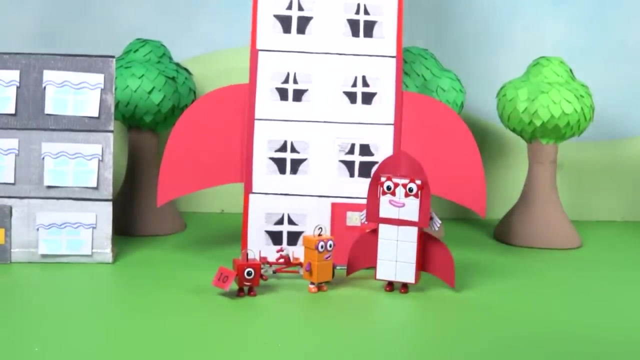 square house with three rows of three grey squares. Time for another invitation delivery. Nine loves parties, but he loves parties even more. Last stop, number block ten's rocket house. But where is she today? Perhaps she's not in. Ten is always full of. 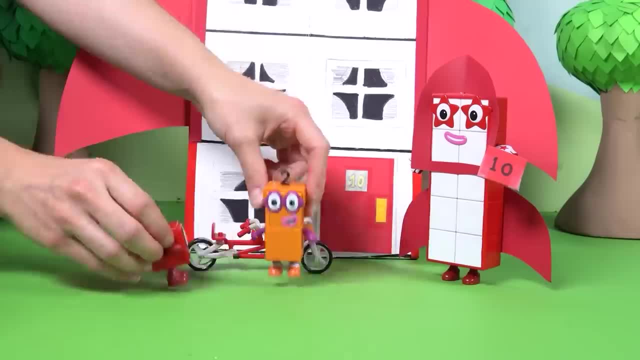 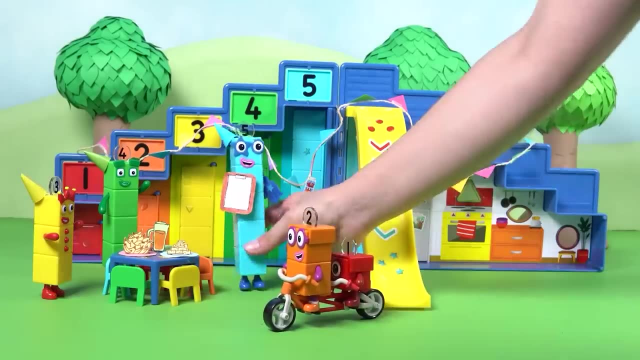 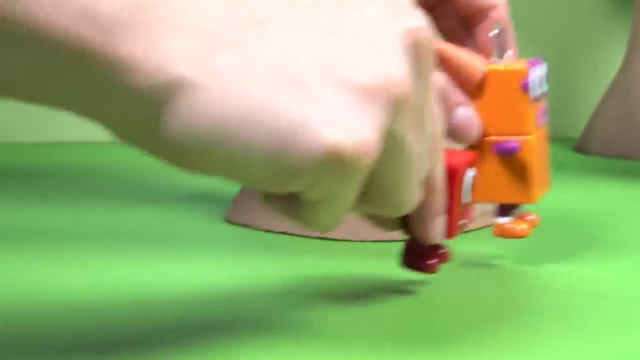 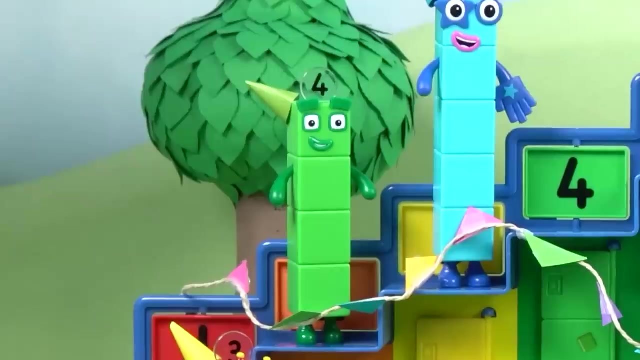 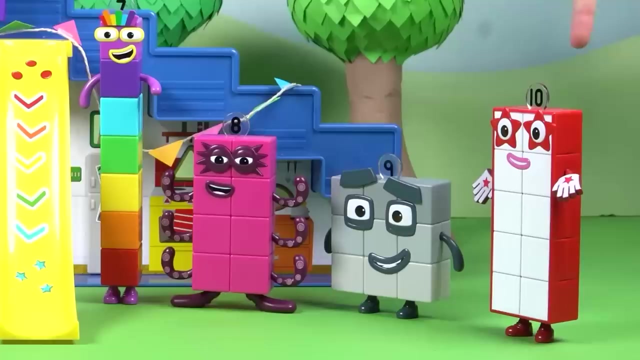 surprises. And now, with all the invitations delivered, it's time to head back. Well, thanks to their speedy delivery, everyone knows about the big party. Is everyone here? Let's check. One, two, three, four, five, six, seven, eight, nine, ten. It's a. 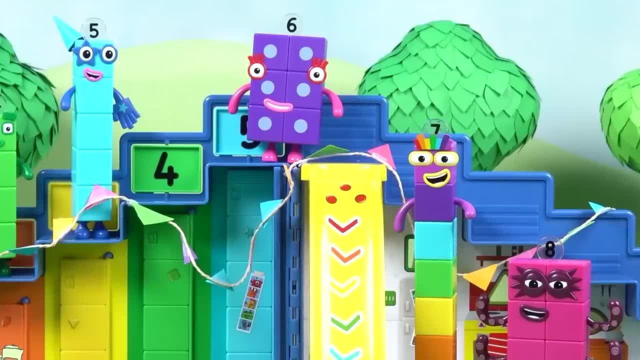 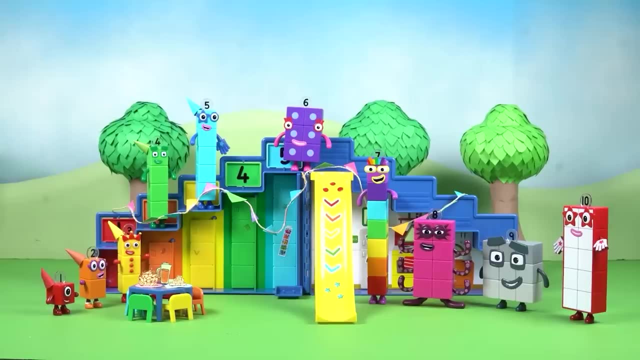 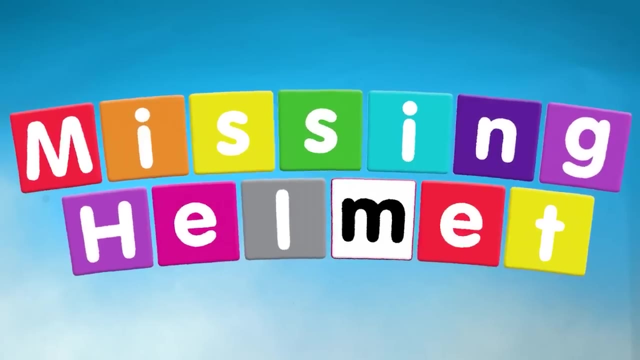 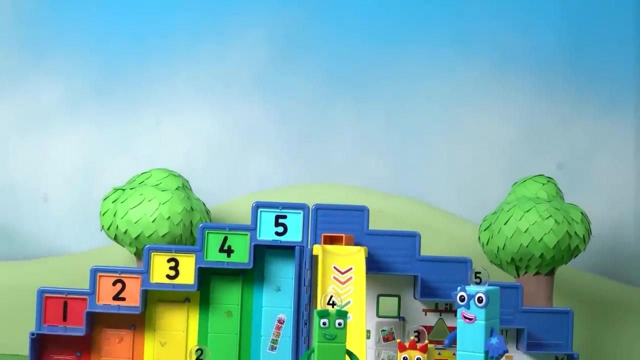 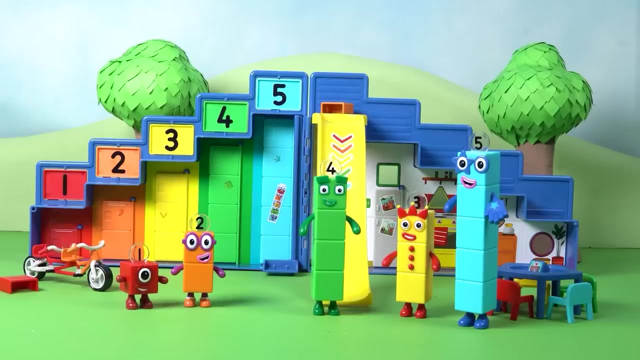 perfect number land. party Number blocks one and two saved the day with their brilliant tandem bike. Hello, number explorers. It's a bright and sunny day in number land And our favorite number blocks are gathered at the top of the hill. I wonder. 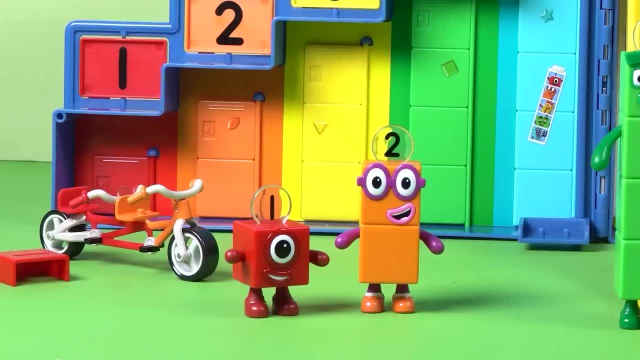 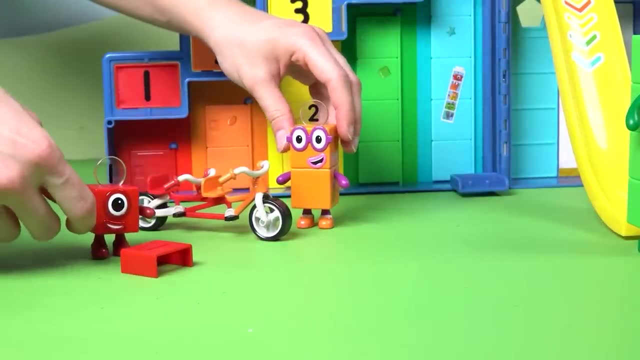 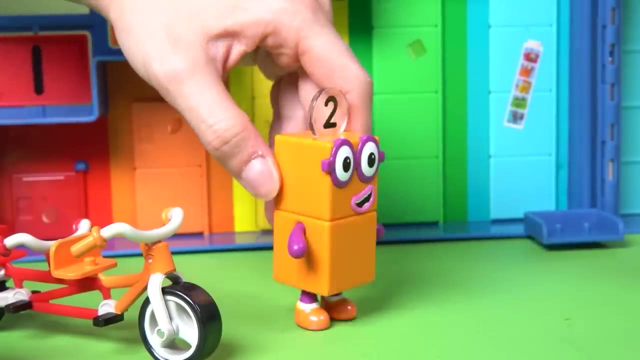 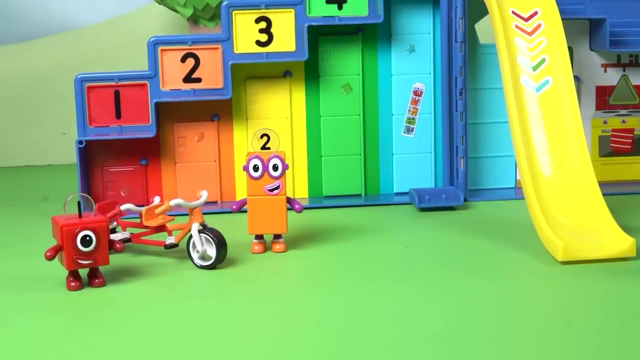 what adventure we'll imagine in number land today. Look, there's a tandem bike, all ready for an adventure, And it seems like number blocks one and two have a plan. Aha, a bike ride. What a great idea. Oh dear, Two can't. 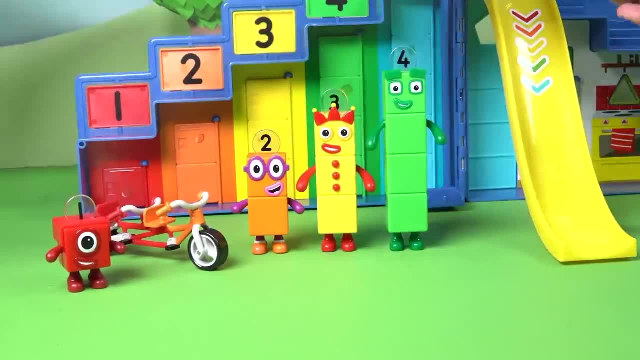 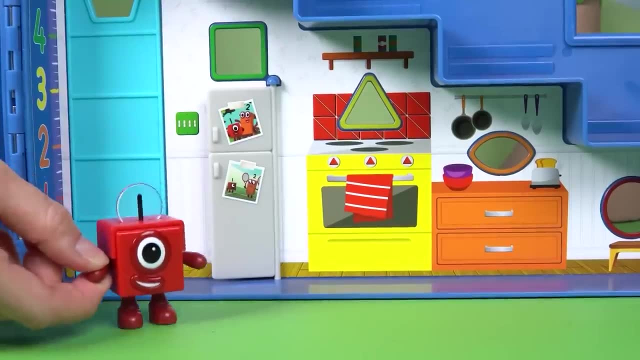 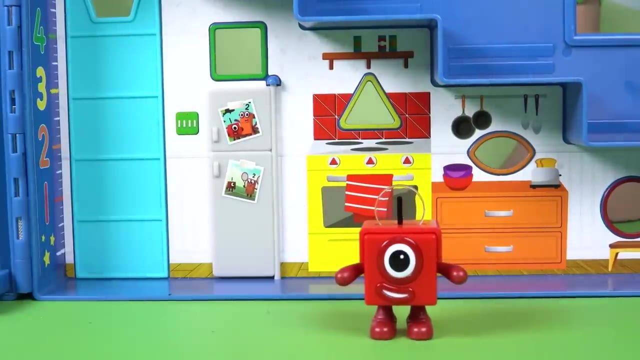 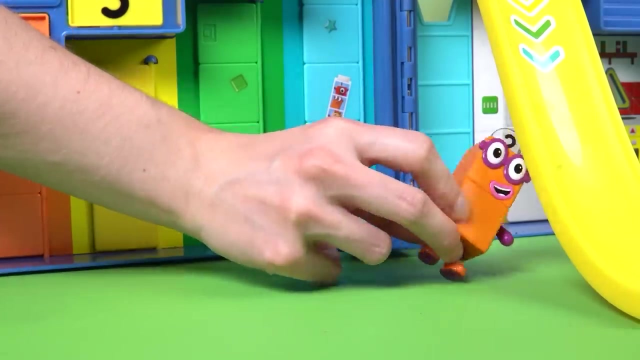 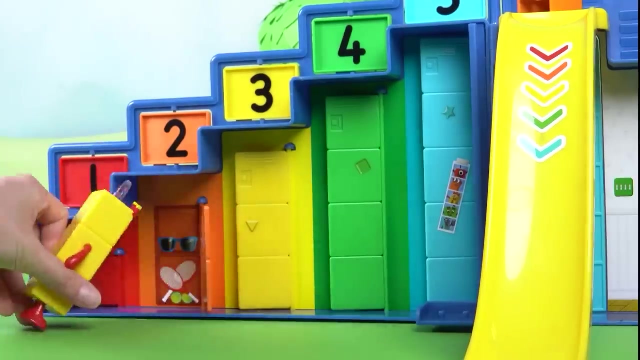 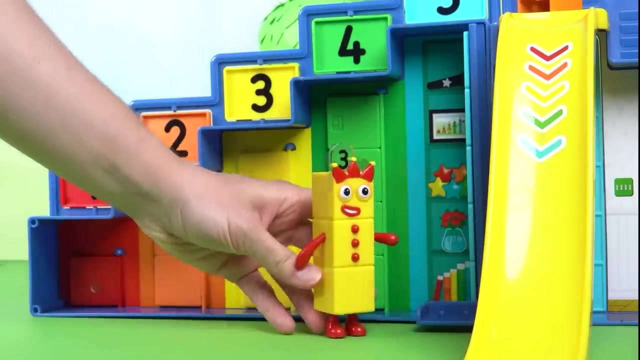 time. This looks like a job for Step Squad. Step one: check the kitchen. Oh no, the helmet isn't there. Step two: check under the slide- Nope. Step three: check the lockers. It might be in one of those. Step four: check. 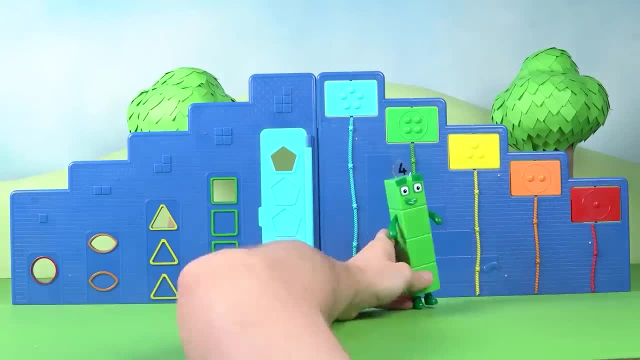 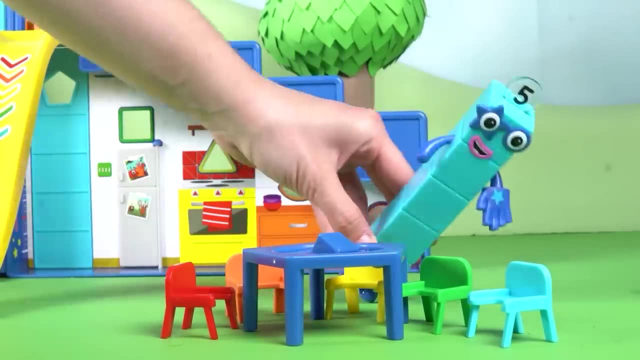 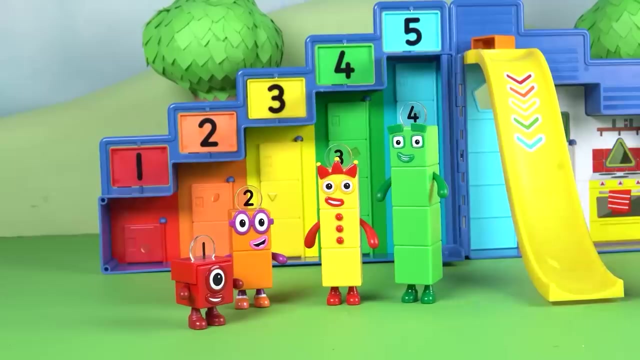 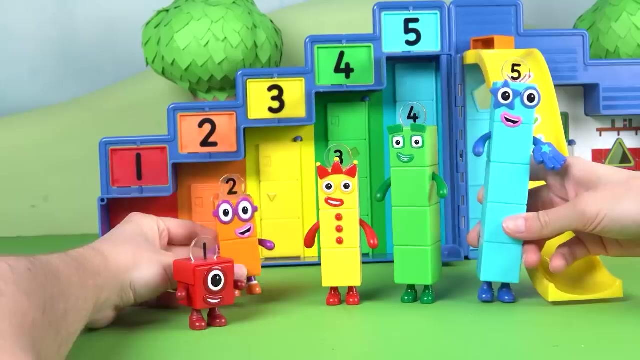 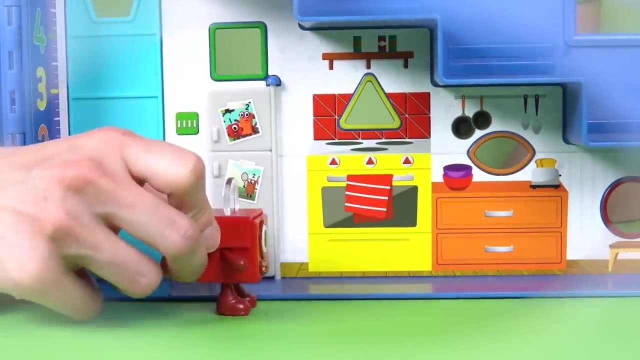 outside the building. Step five: check under the table and see if it's there. Oh dear, The five step plan is complete, But the helmet is still lost, Let's think. Hmm, One checked the kitchen, Two checked under the slide. 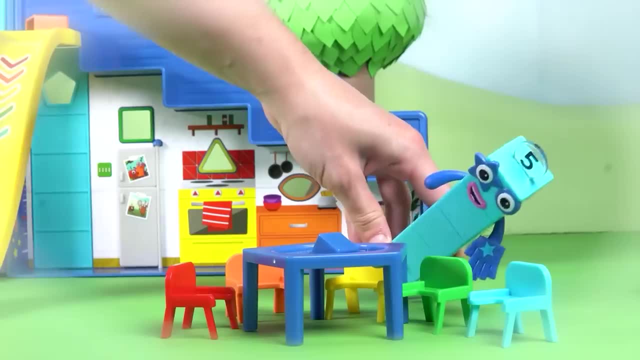 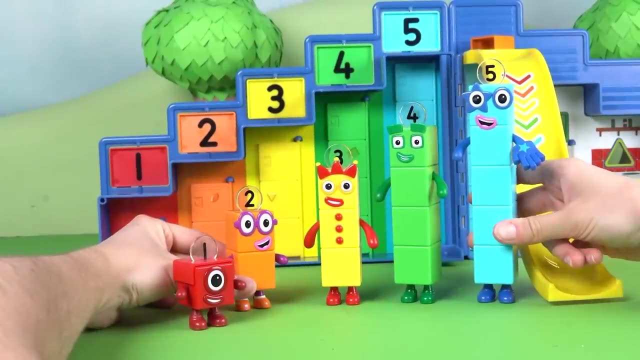 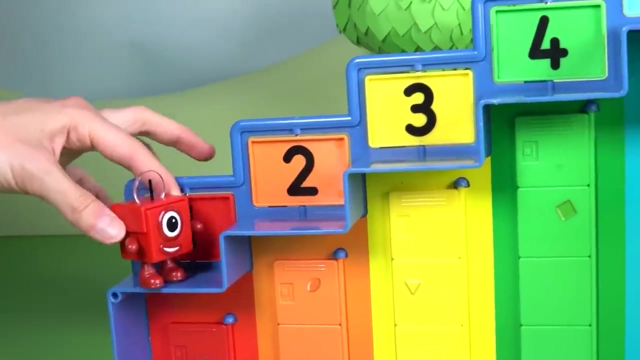 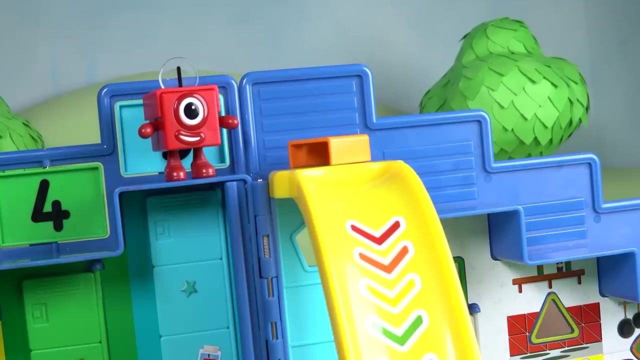 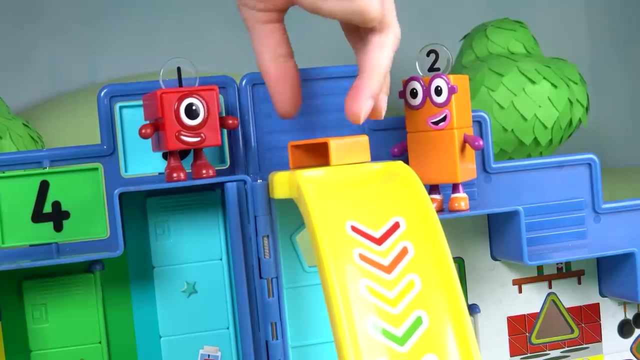 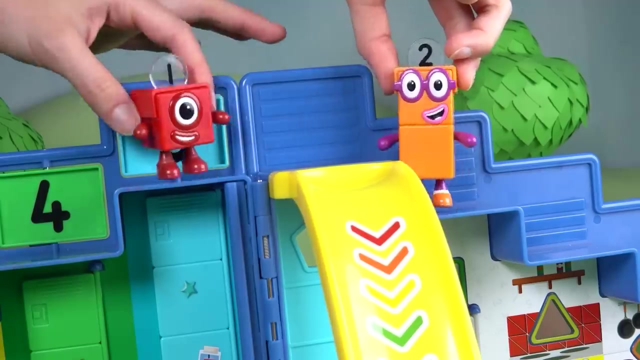 Three checked inside the lockers, Four checked outside, where they haven't checked. One has an idea: The steps. Fancy that The step squad forgot to look on the steps Number block. one has found something And there it is: The head. 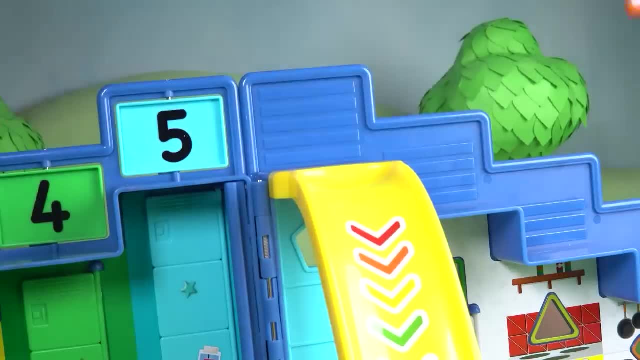 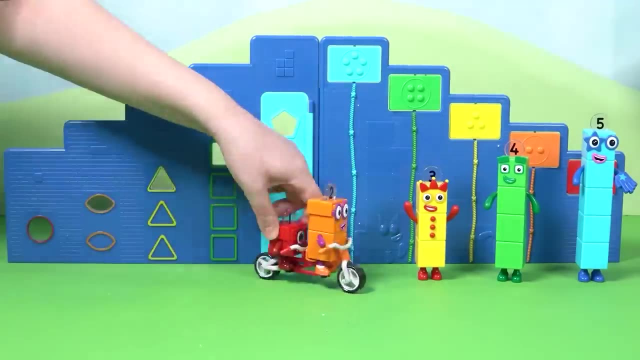 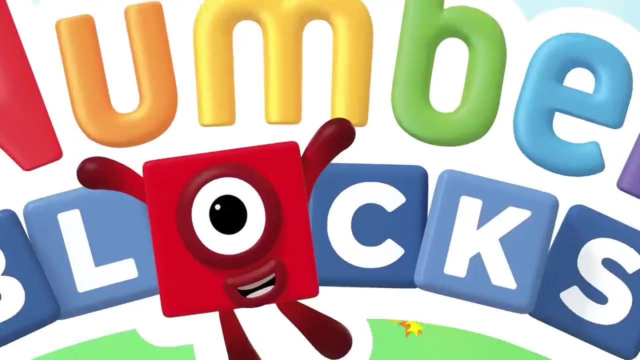 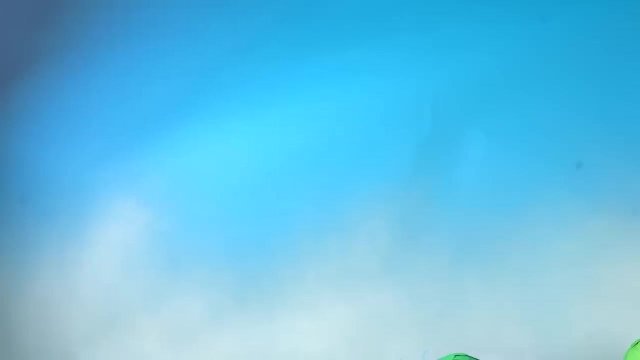 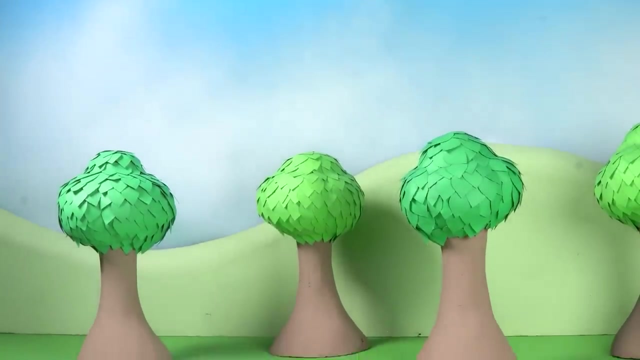 And so another exciting day at the mission headquarters comes to an end. With a bit of teamwork, the super special secret step squad can solve any mystery. I wonder what adventures they'll find in the next episode. Let's find out what story we're. 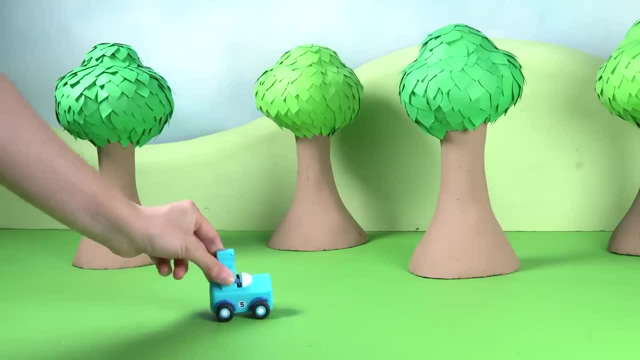 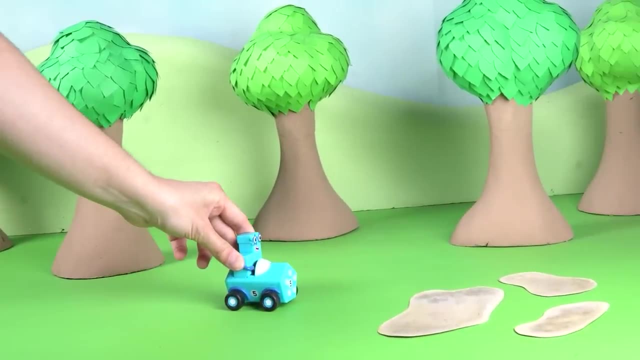 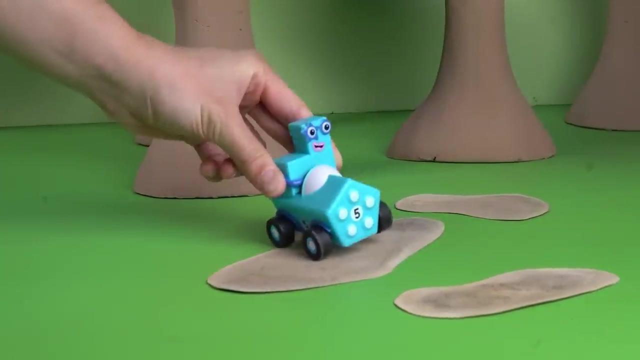 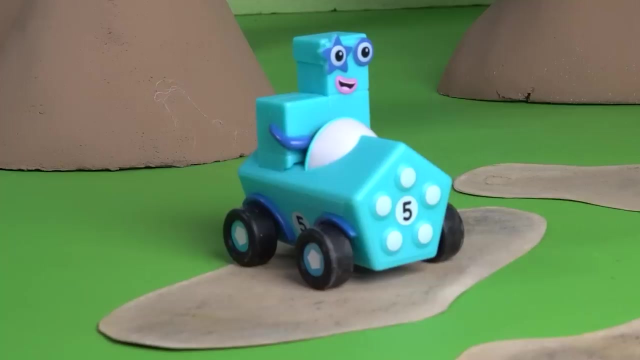 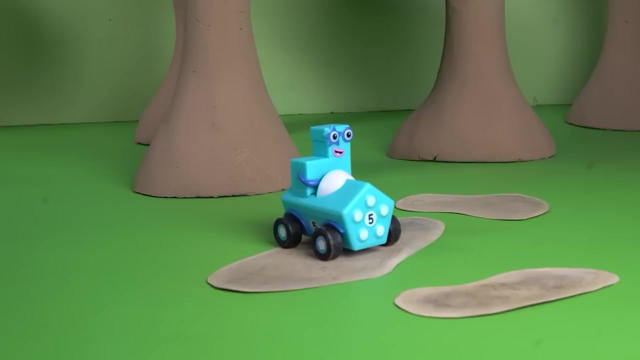 imagining today. Look over there, It's number block five driving her car- Vroom, vroom. She's having such a lovely time. Number five has driven into the ditch. She's okay, but her vehicle is stuck. She needs some help. 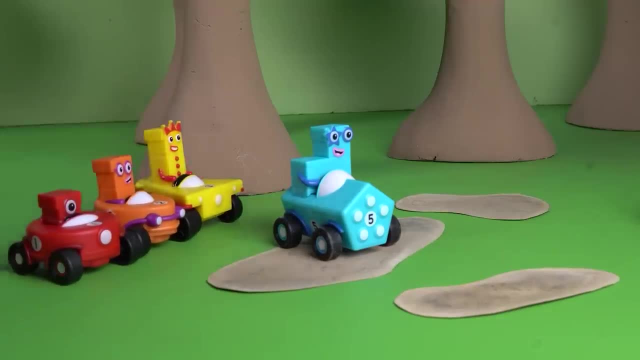 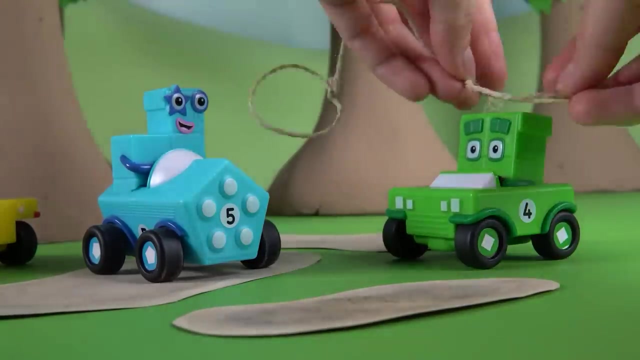 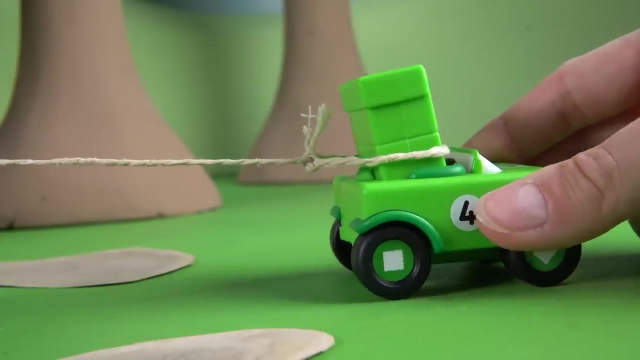 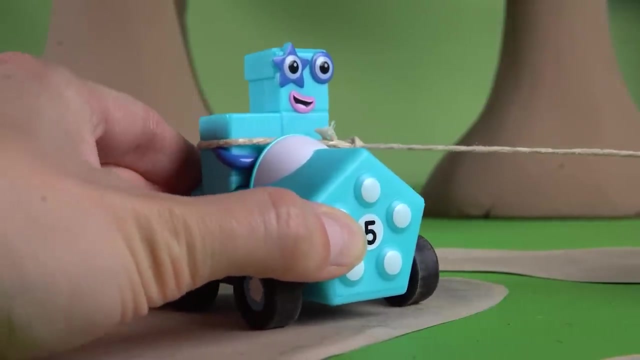 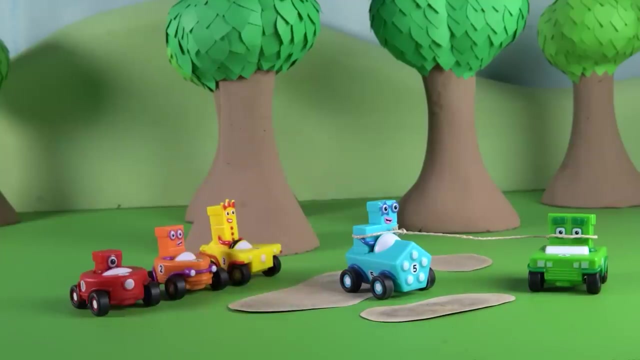 Can you think of who might come to her rescue? Listen, Do you think they can do it? Four seems to have an idea. He's attaching some string to Five's vehicle. Do you think he can pull her out? Oh, no Even. 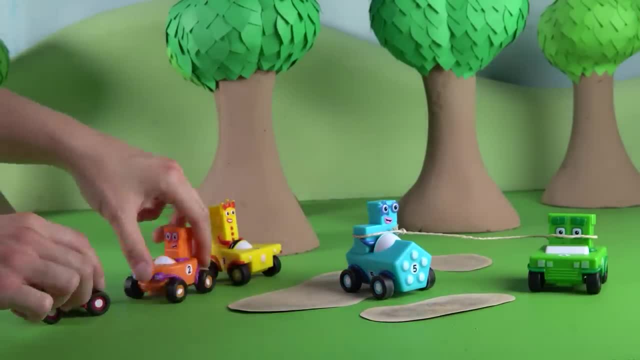 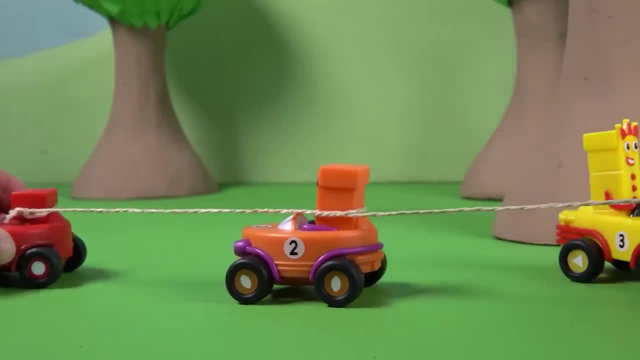 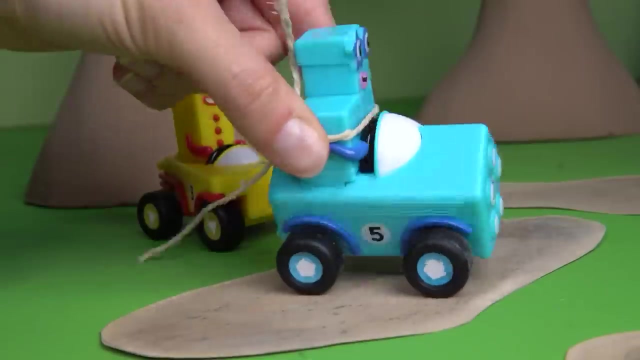 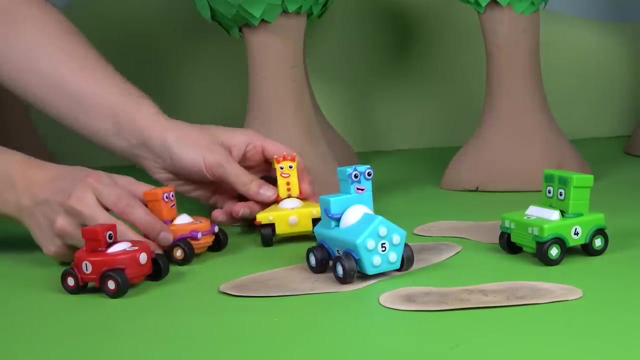 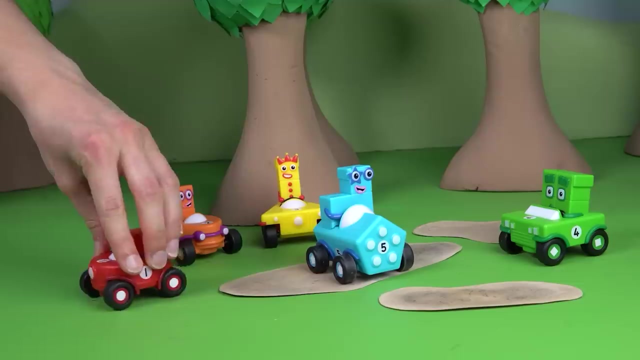 with number block one. they seem to have a plan. Working together is always a good idea, isn't it? One and two are giving it their best shot. Can they do it? Oh dear, Even working together, number blocks is a good idea. 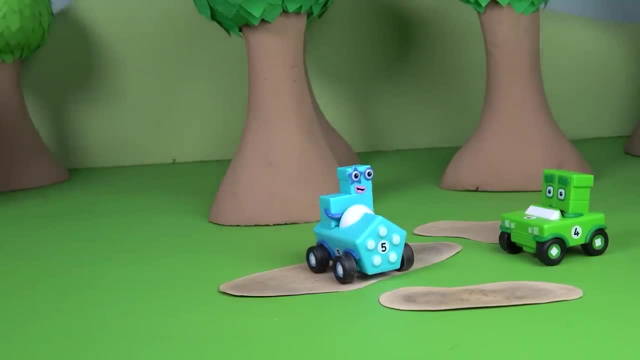 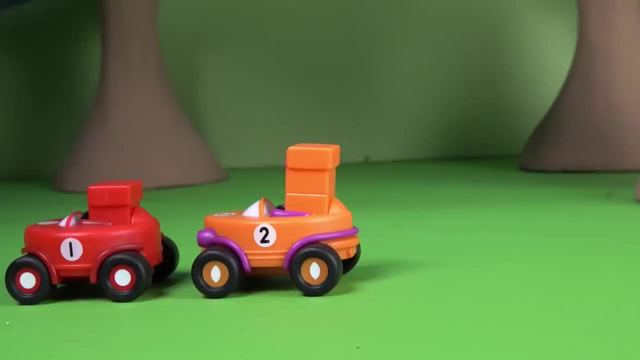 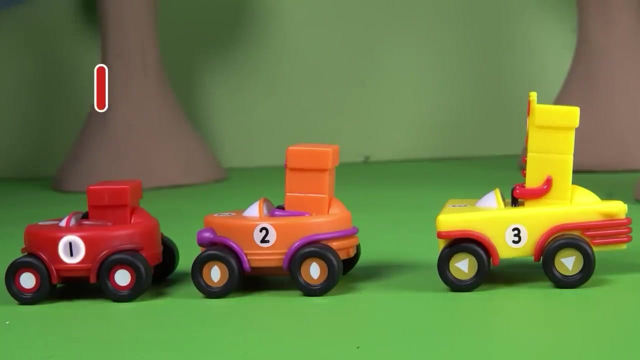 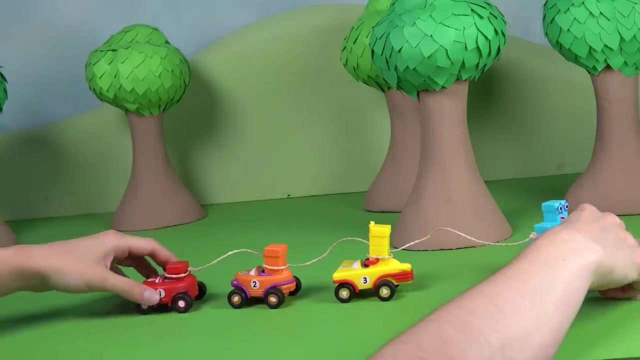 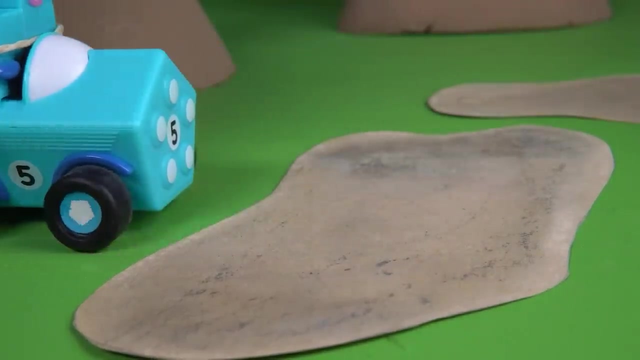 What if they add their numbers together to make a bigger number? Maybe only numbers bigger than Five can pull Five out of the ditch. Let's see: Plus two plus three equals six. Six is greater than five. Oh hooray, Thanks to. 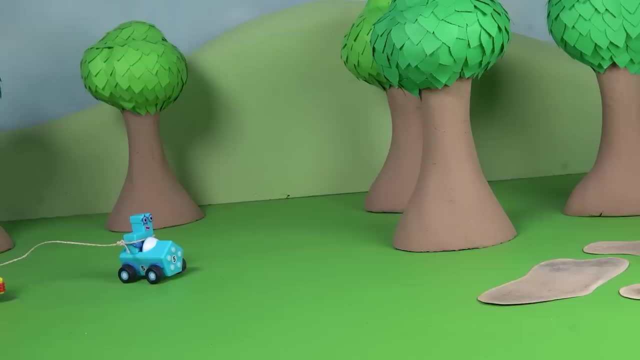 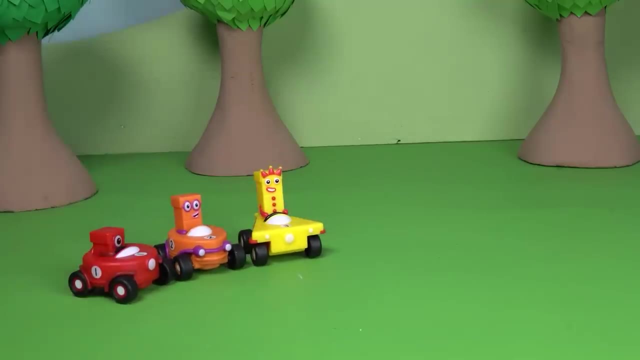 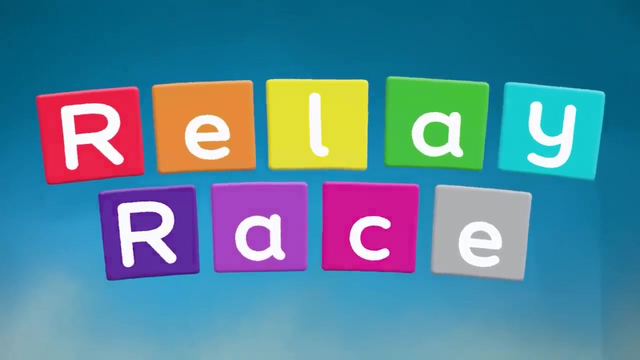 teamwork and some clever adding, the number blocks can solve any problem. And that's the end of our mini adventure today. number explorers, Remember, when we work together and use our number skills, we can solve any problem, Until the number blocks. 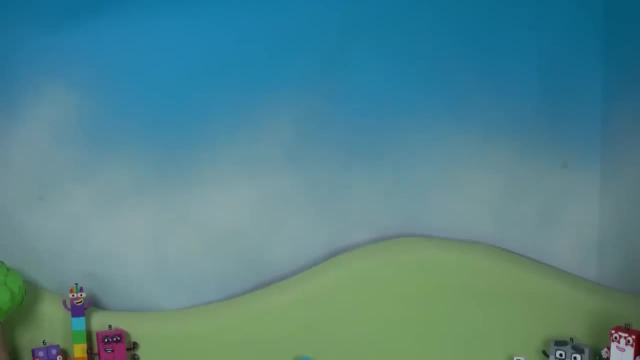 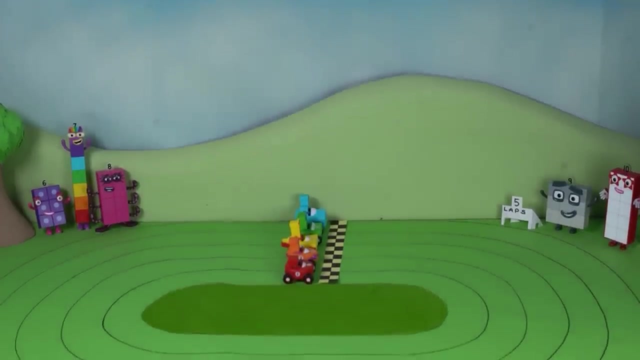 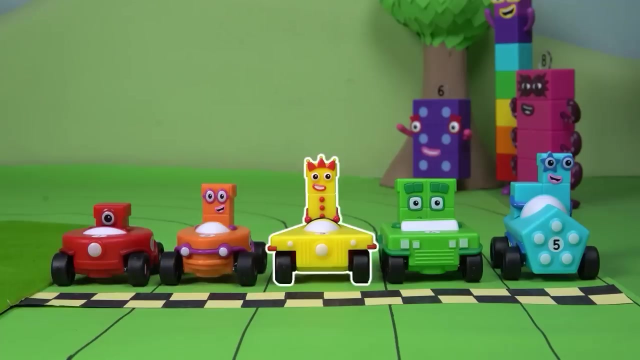 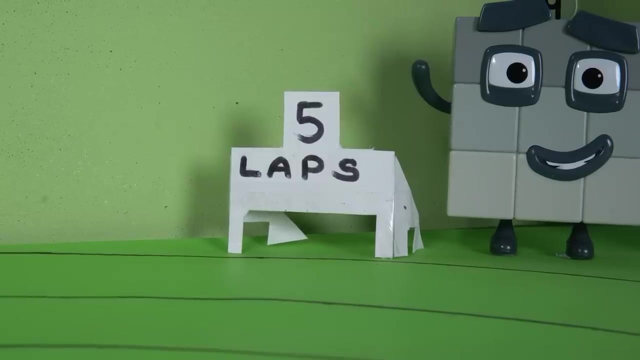 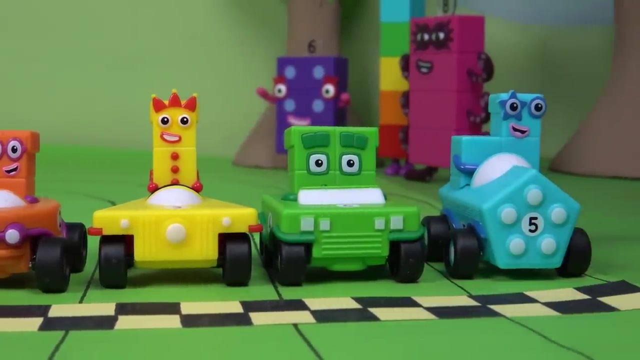 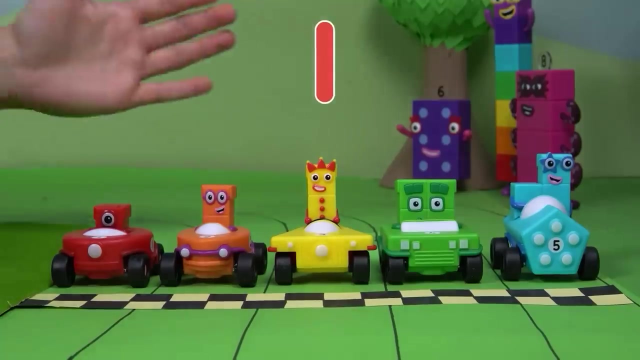 grand race day. Let's see what wonderful adventures we'll imagine. today It looks like our favourite number blocks are getting ready for a thrilling race in their mini vehicles. Everyone is ready to get racing. Five, four, three, two, one. 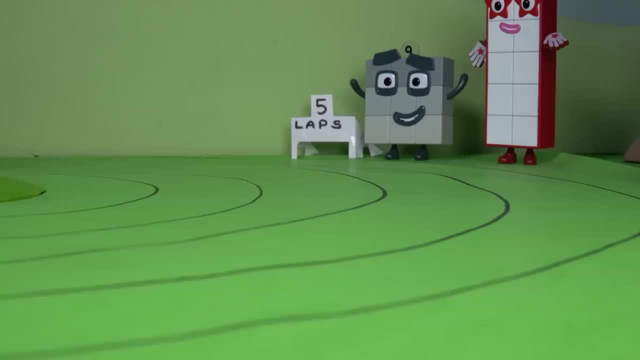 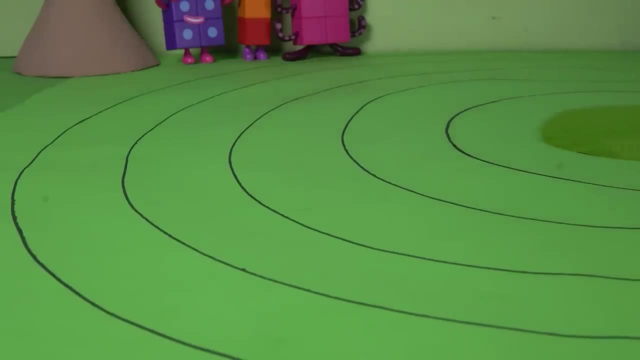 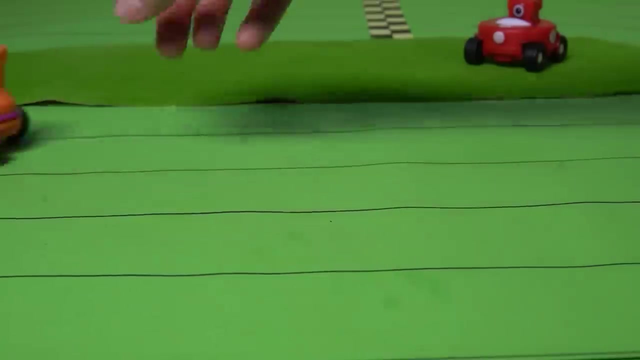 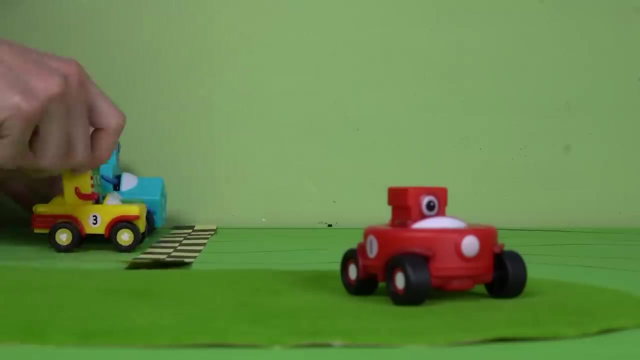 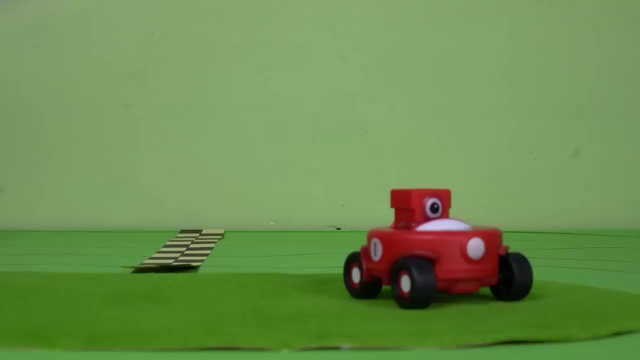 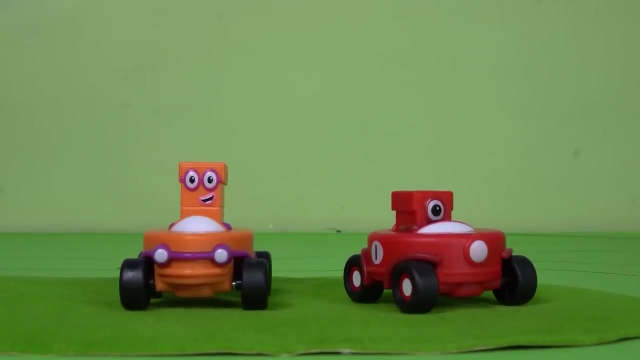 go And they're off. The number blocks. grand race day has begun. Who do you think will win? Remember, she loves the number one, so she did one large lap. And here comes number block two. He's done two laps because 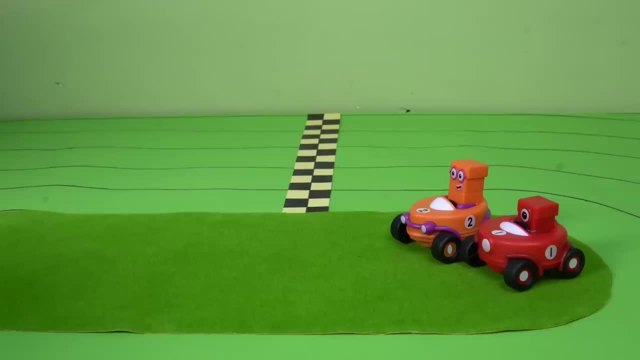 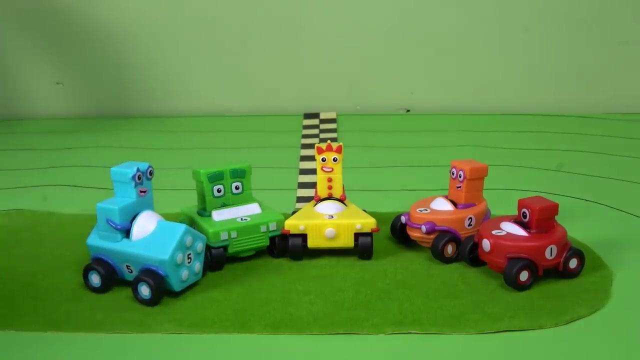 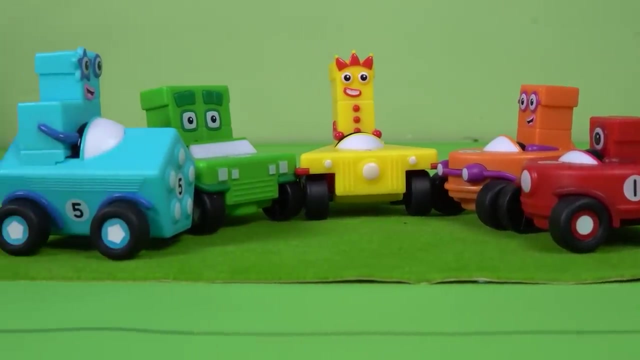 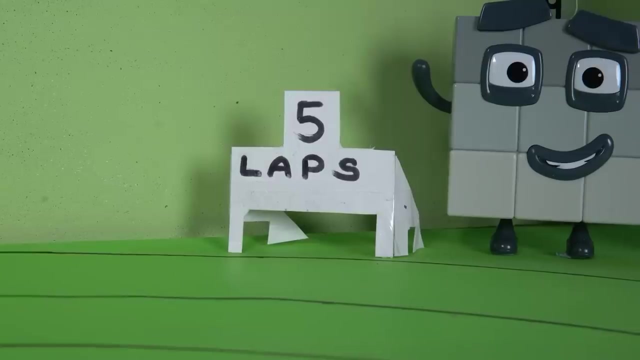 he loves the number two. Let's count the number blocks. Number blocks three, four and five are still racing, but one and two have stopped. I wonder why. Oh dear, It looks like our number blocks are unsure numbers. Number. 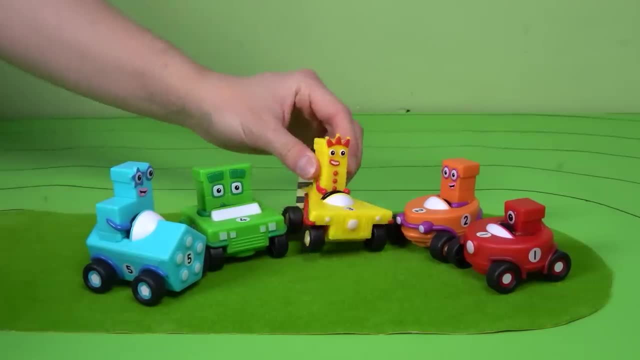 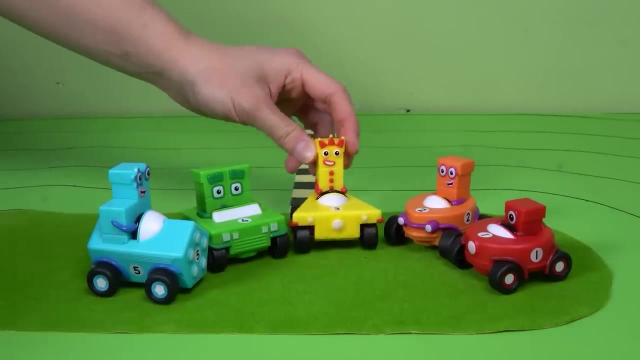 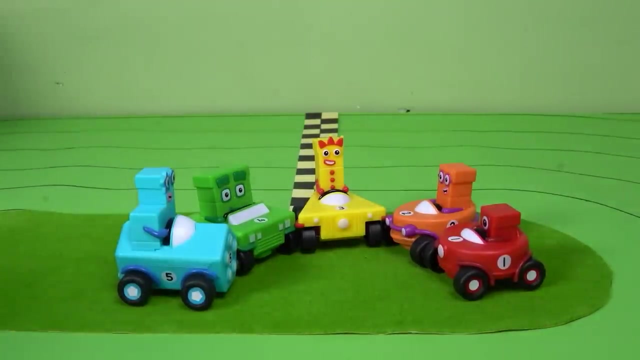 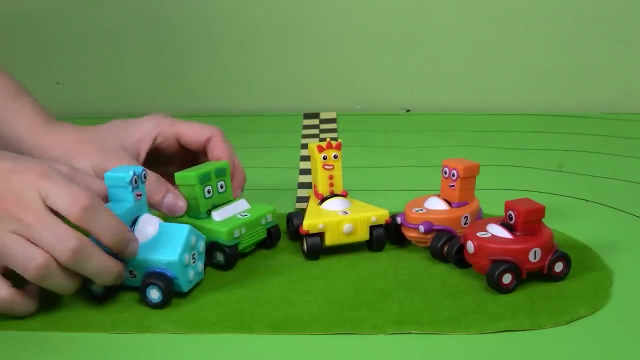 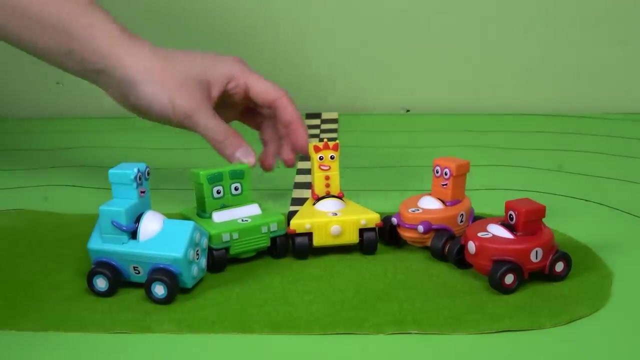 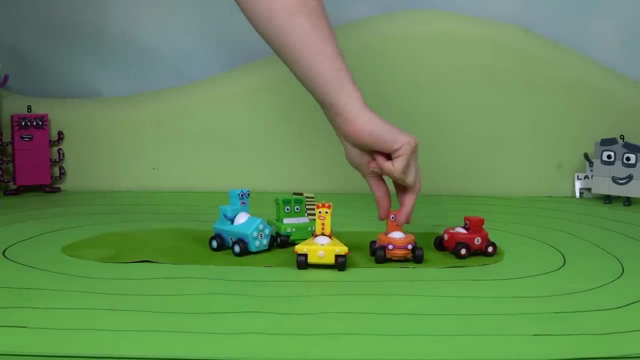 block one did one lap and number block two did two laps. What should they do? Aha, It looks like number block three has a brilliant idea. Number block needs to find a partner so that when their numbers are added together, they make. 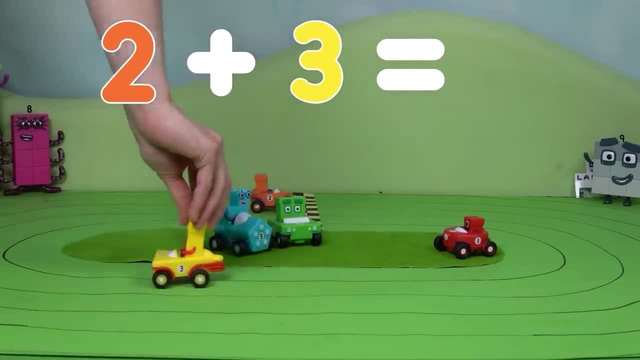 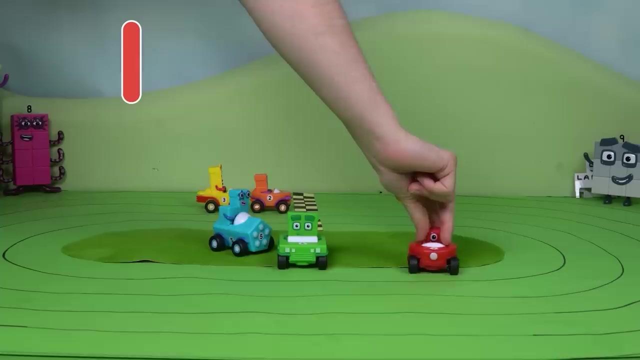 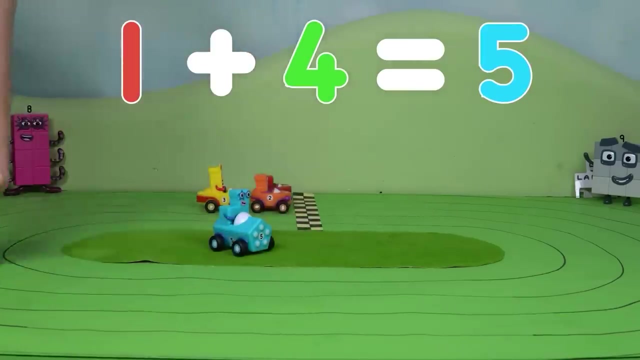 the number five. Look at that Number block two and number block three and one partnering with number block four. One plus four also equals five. Great job number blocks. Don't worry about number block five, Since she's already the number five. 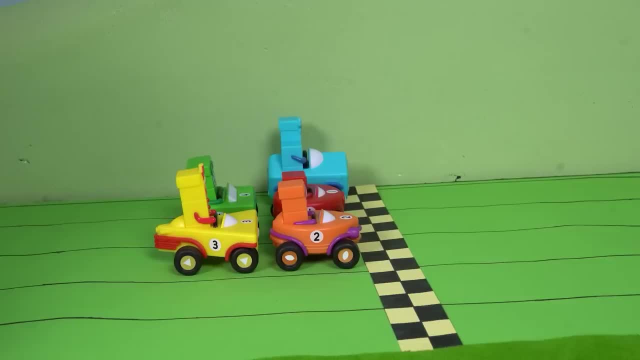 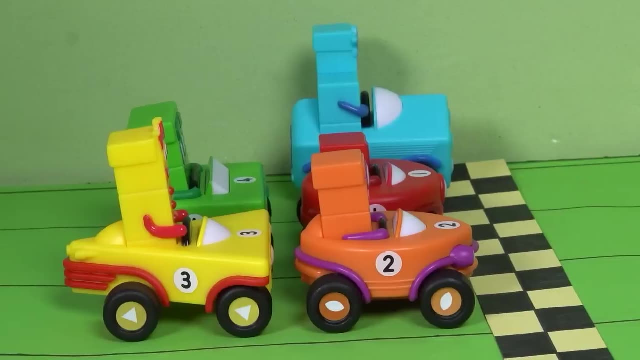 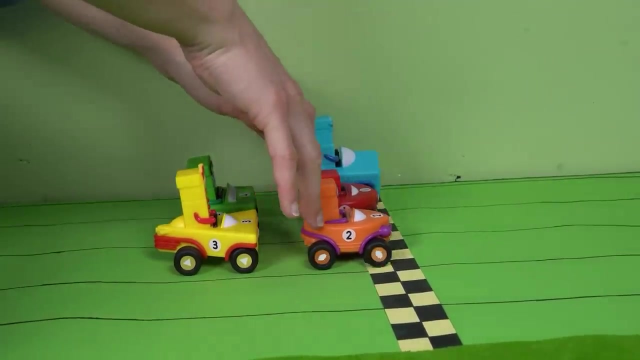 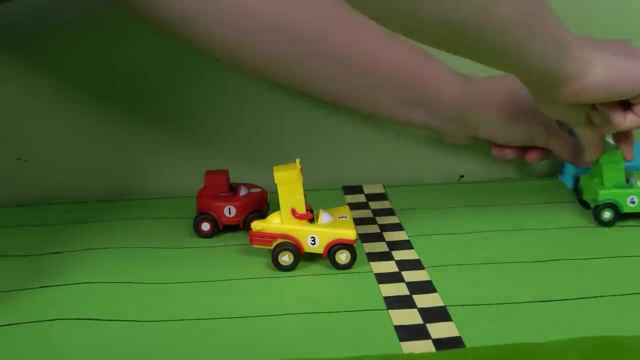 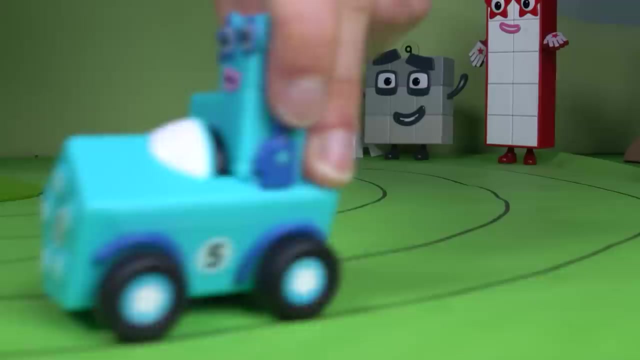 she needs to find her partner. Get ready, number explorers. The relay race is about to begin. Each number block will race their laps and then pass on to their partner. Let's cheer them on. Four laps for their team And number. 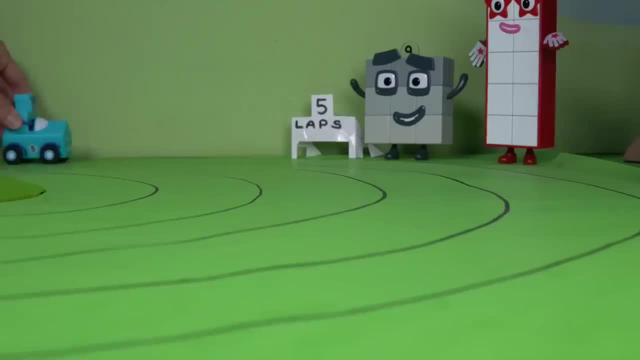 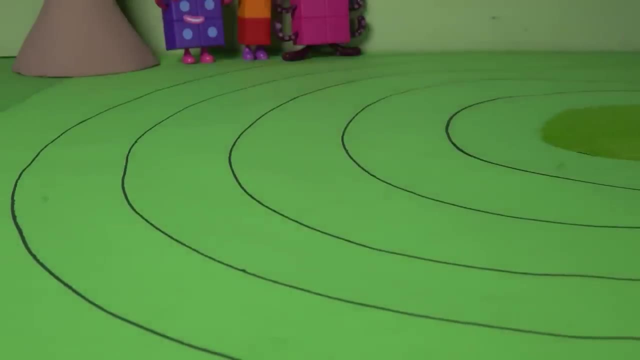 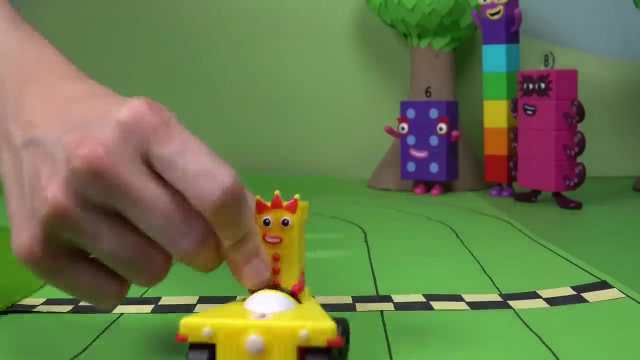 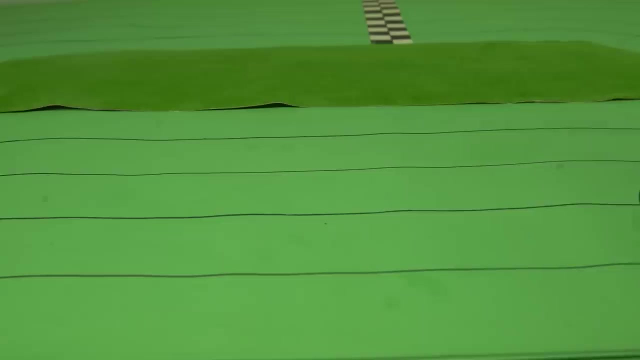 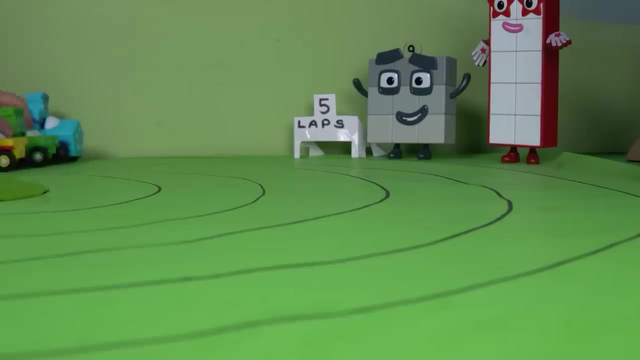 block two finishes her lap. She hands over to three. Look at five Go. She's racing all on her own and doing an amazing lap. So close, Who's going to win? One lap left? Woohoo, It's a. 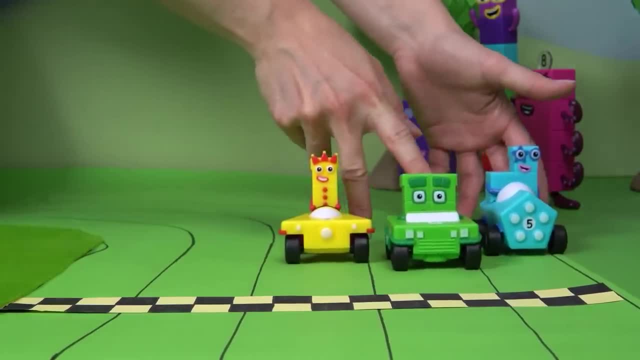 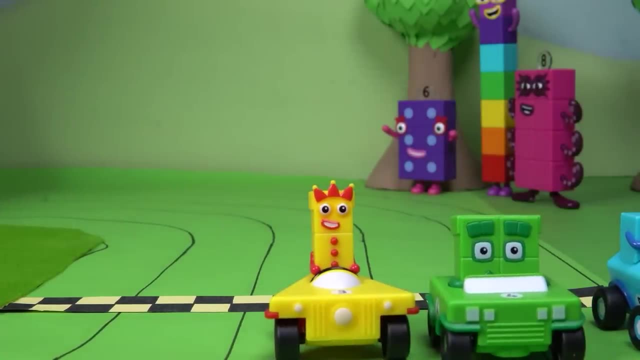 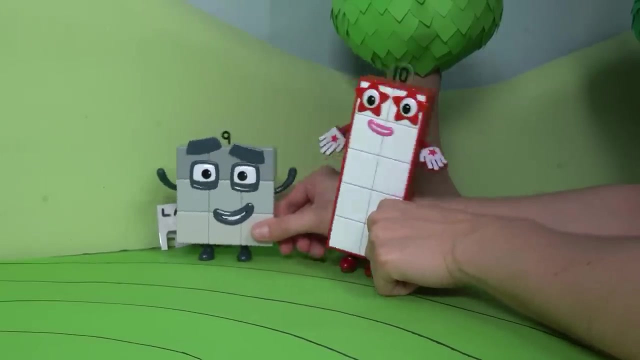 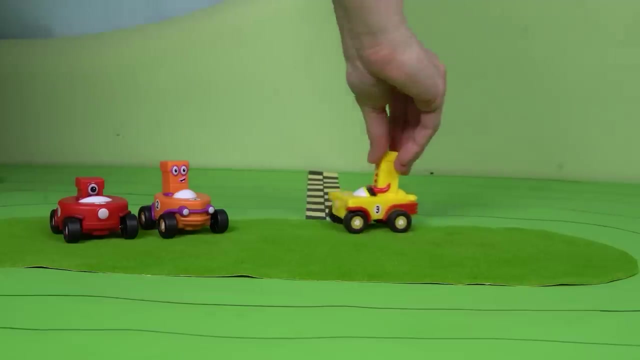 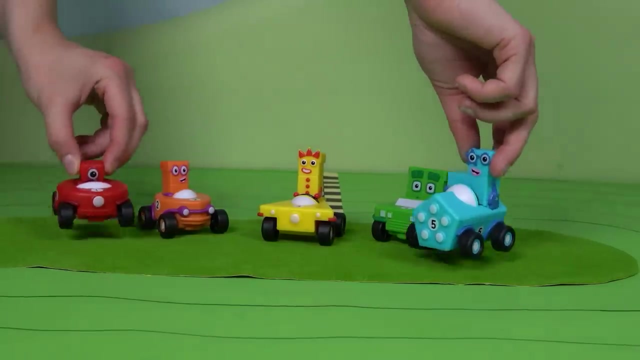 tie. What an exciting race. All the number blocks have shown great teamwork and racing skills. today In Numberland, it's not about winning or losing. It's about having fun working together and imagining wonderful stories. Well done, number blocks. 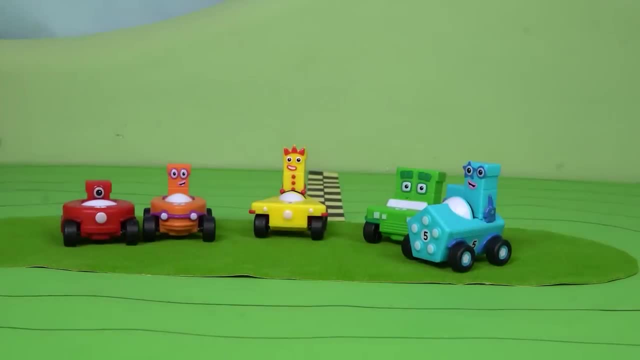 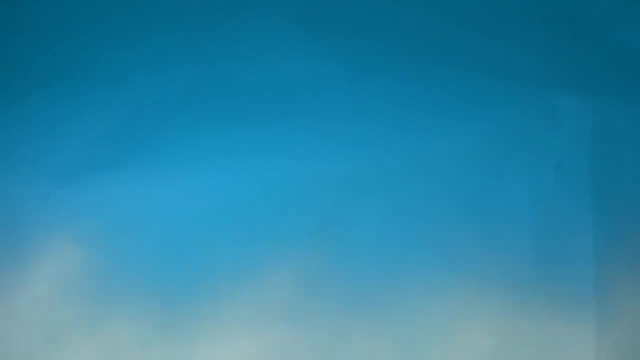 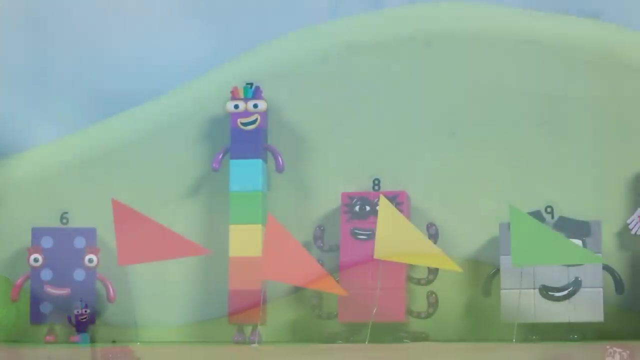 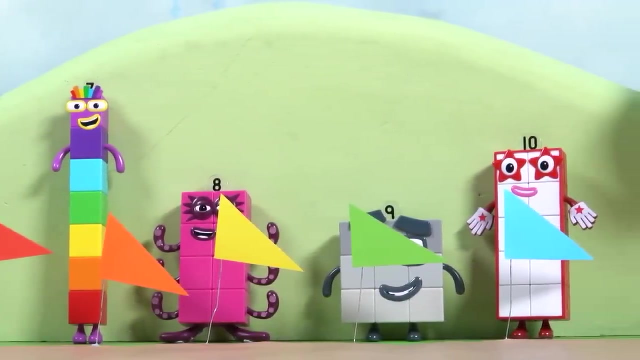 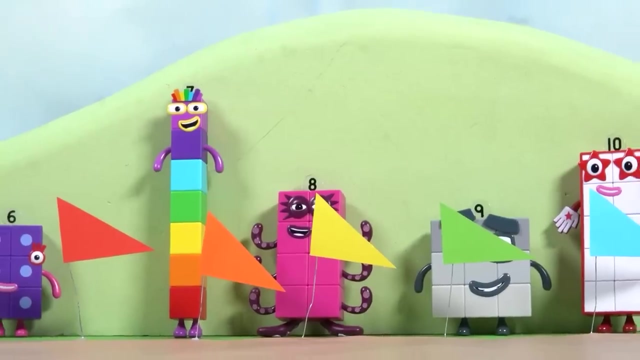 And well done to all our number explorers for cheering them on Welcome number blocks. I wonder what creative stories we're going to imagine today. Well, it's the grand number land race day Today. our favorite number blocks are gearing up. 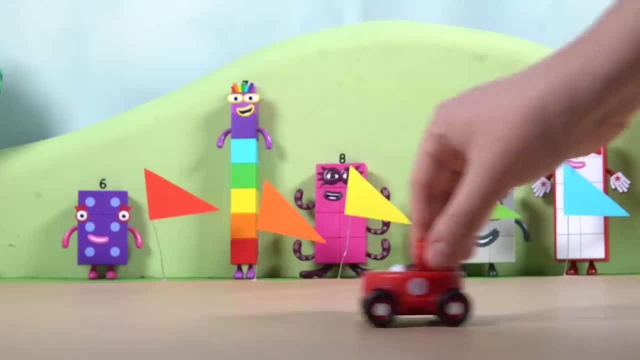 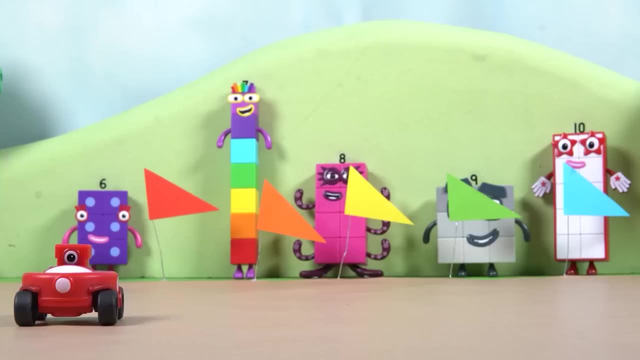 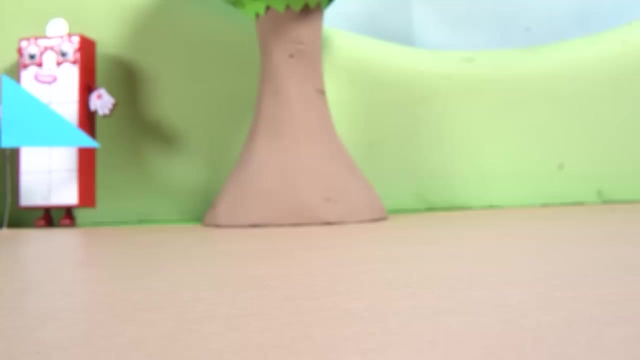 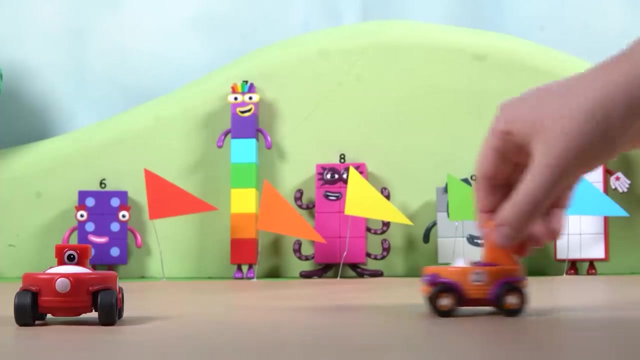 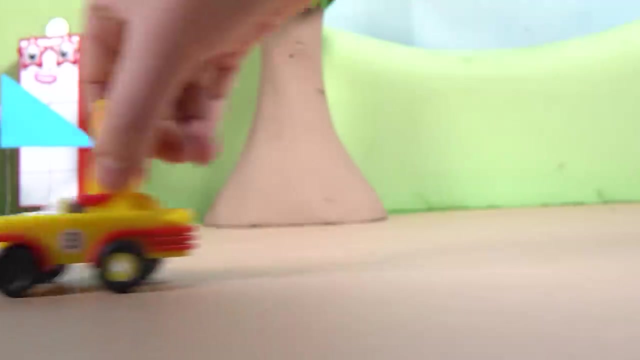 for an exciting race. But wait, these are just like her eye, her circle One, circle one car, one number block one. Can you see the number one on her car? And here's number block two, with his look at her car. 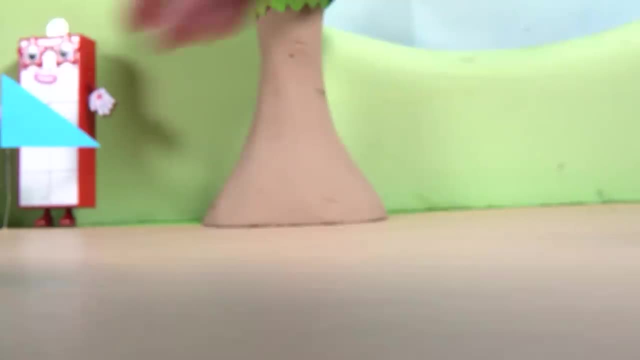 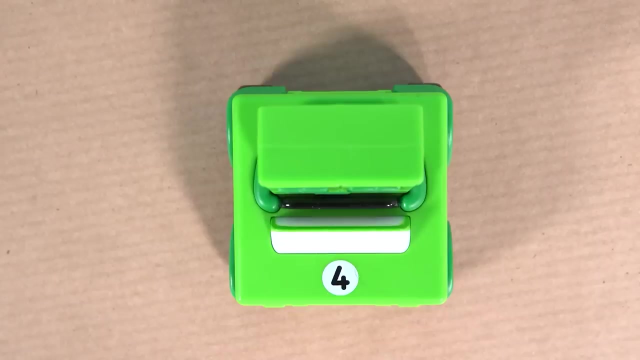 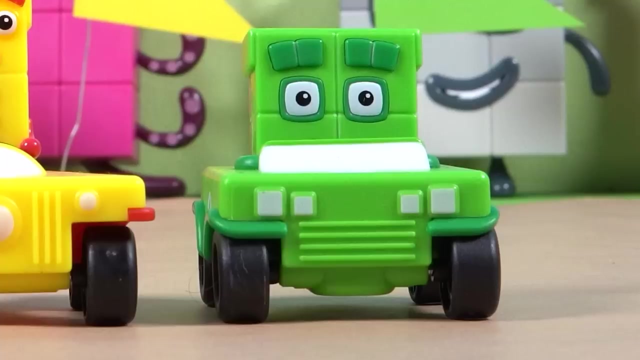 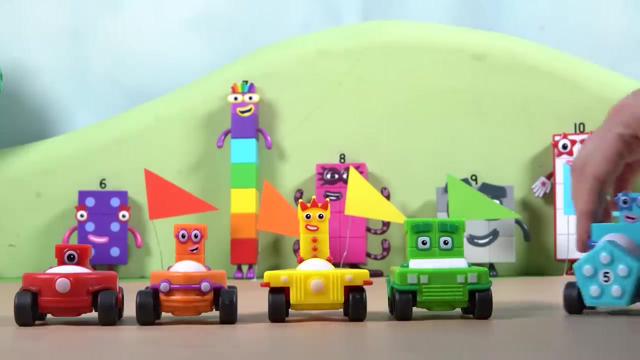 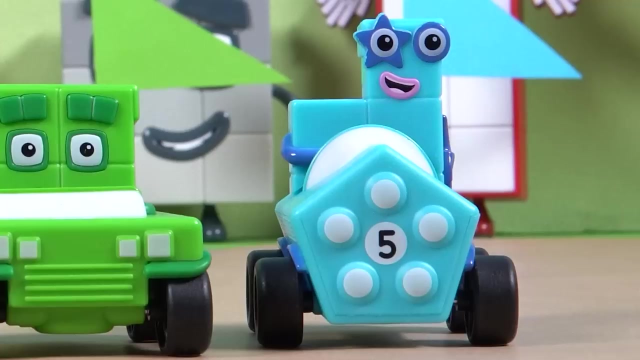 shaped like a perfect triangle. Over here we have number block four with his square car, Four sides, four corners, four wheels- Everything is just right for number block five And they're off. Look at them. go speeding down the number. 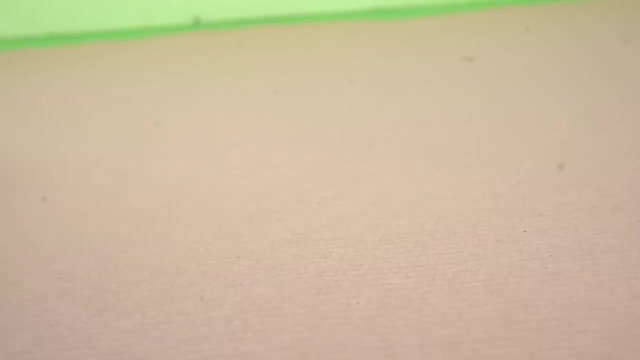 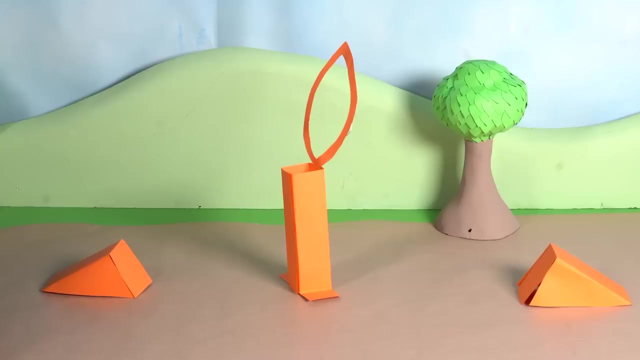 land track. But wait, what's up ahead? Oh, a round tunnel up ahead. Who do you think can walk one and her circle car fit perfectly. Well done one. Uh-oh, a leafy hoop. But which car is? 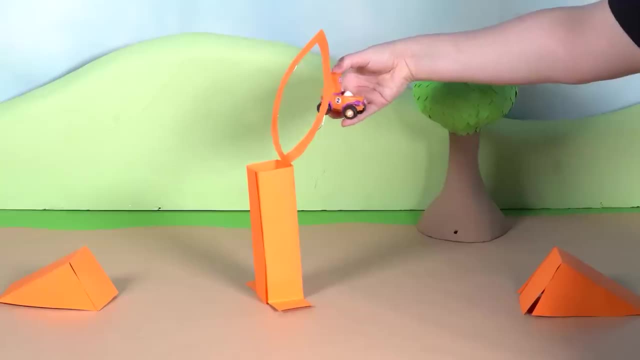 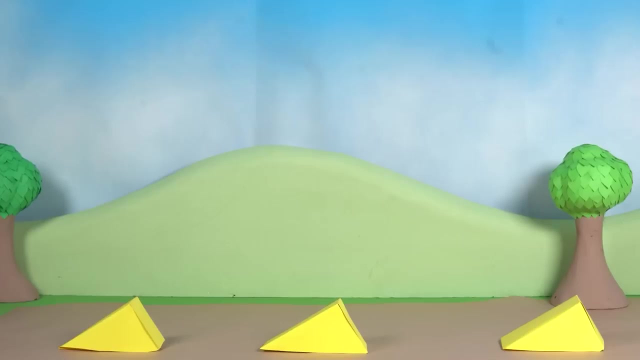 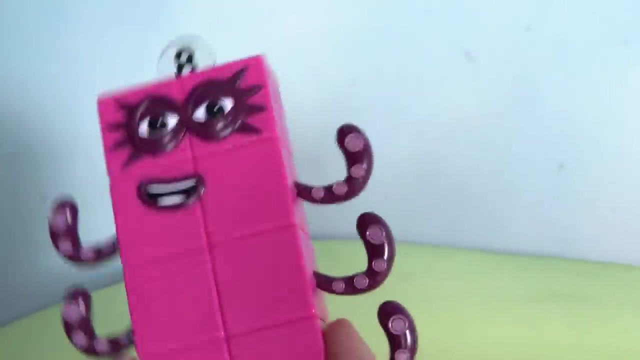 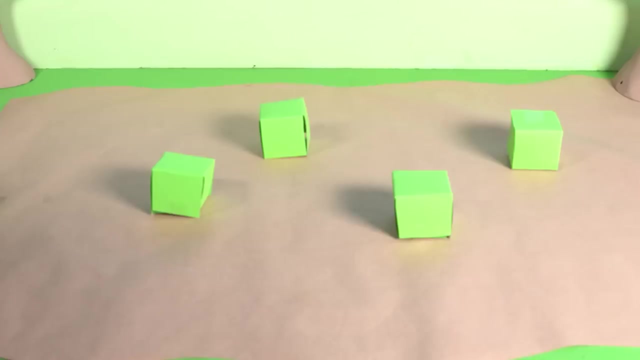 shaped just right to navigate it. Oh, fantastic Number block four's triangle obstacles. Only someone with a triangle car will be able to move those out of the way. Three makes it look so easy with her triangle car. Way to go. three: 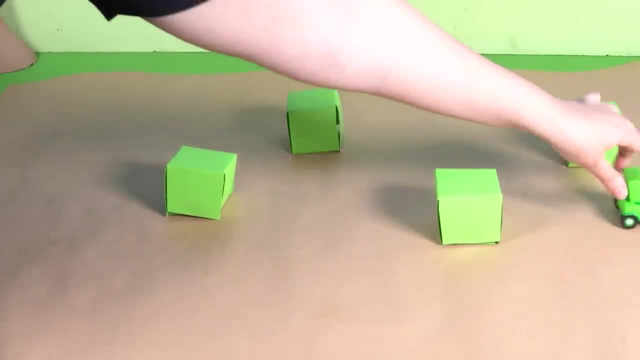 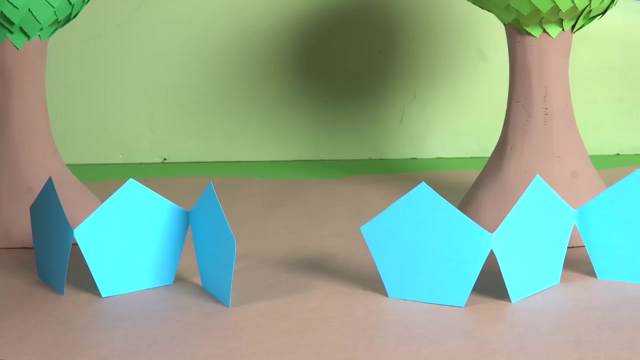 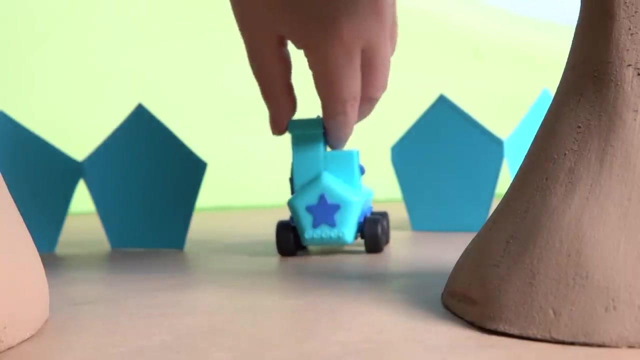 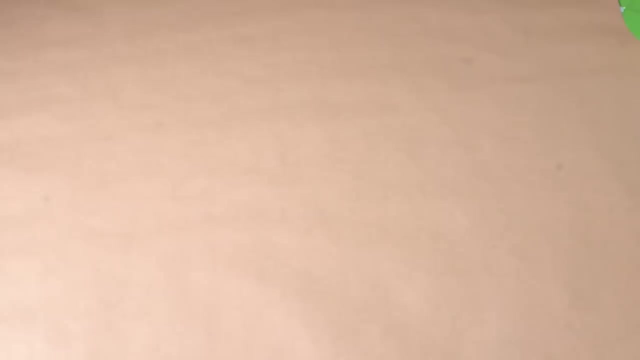 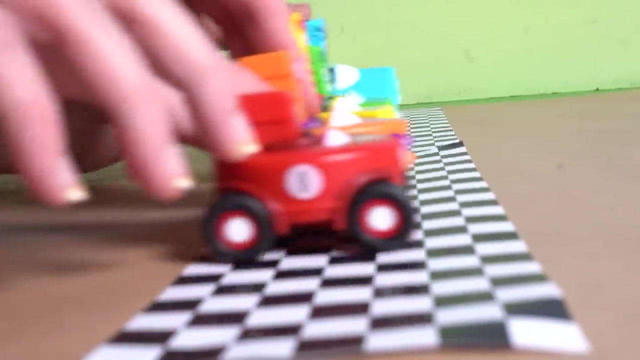 Square fits right between the blocks. Onward four. Last obstacle: pentagon gates. They might be narrow, but who has the perfect car to pass through? Hooray for number block five: Look at that, They're crossing the finishing line. 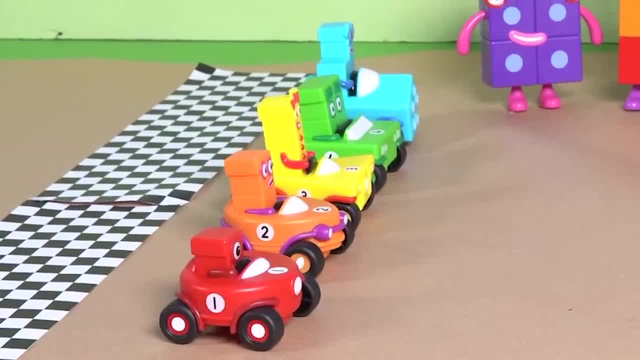 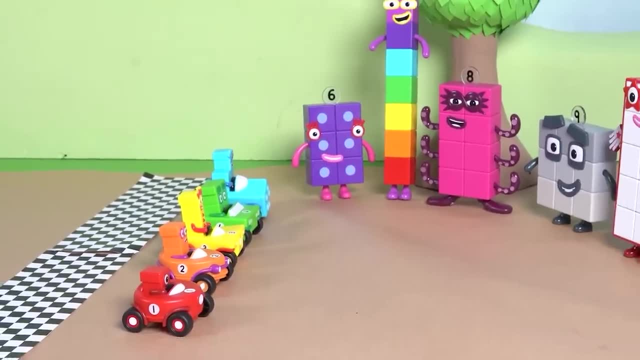 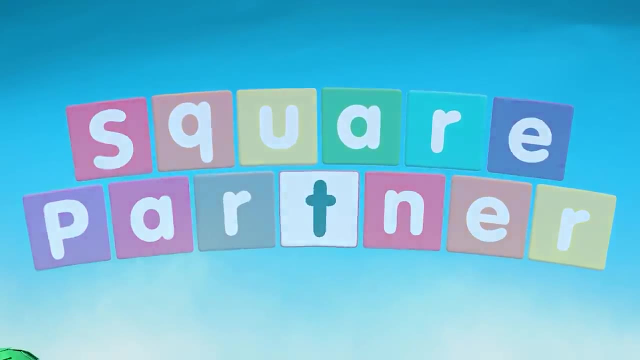 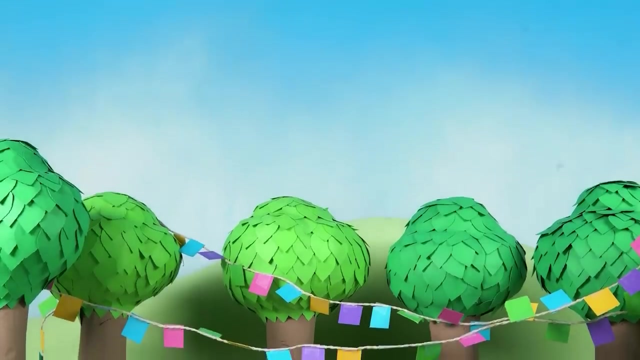 together It's a tie. What a race. Today, our number block showed us that it's not always about winning, but about having fun and facing challenges. Well done, number block. Hello number explorers, Welcome to Number Block One. 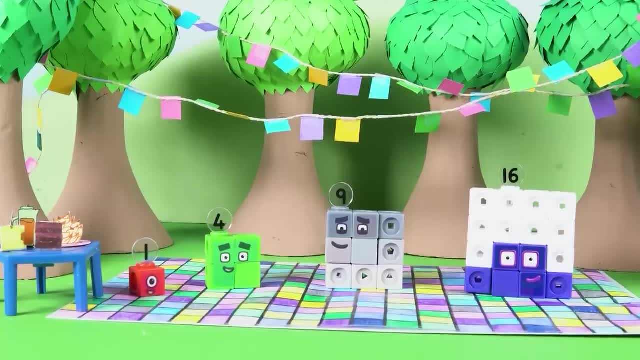 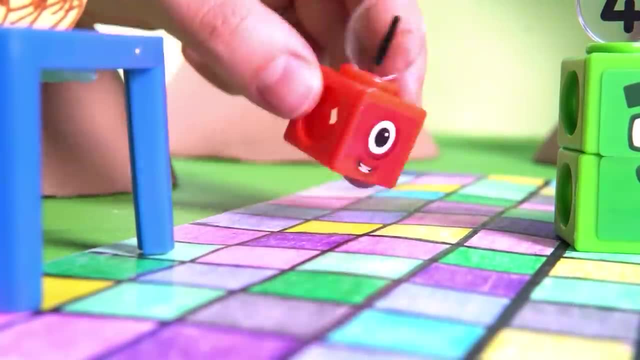 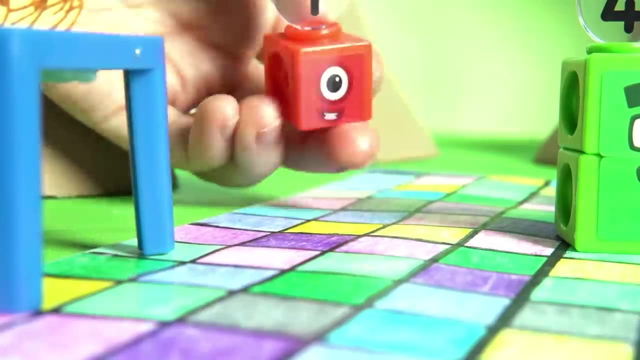 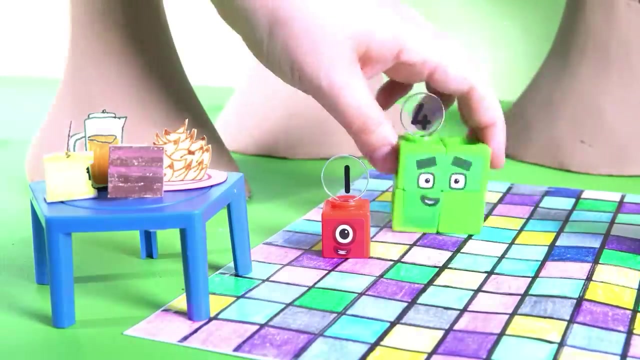 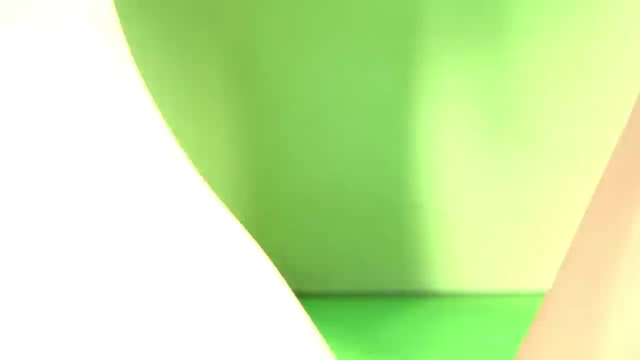 Today we have a special celebration for our square number friends. Let's get playing. Look at number block one. She's jumping onto her side. Each side is the number block four, Setting up a snack table with square treats. Yummy. 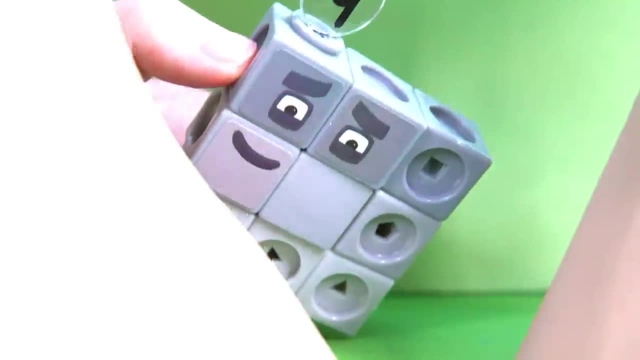 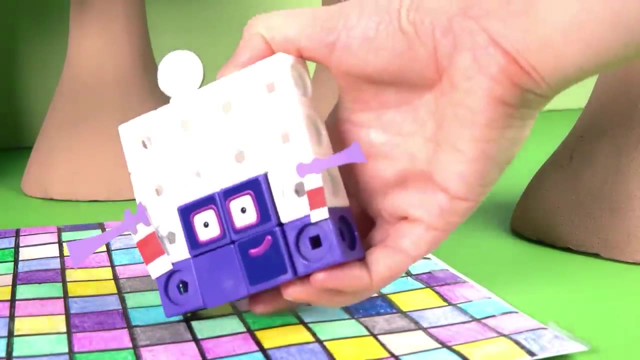 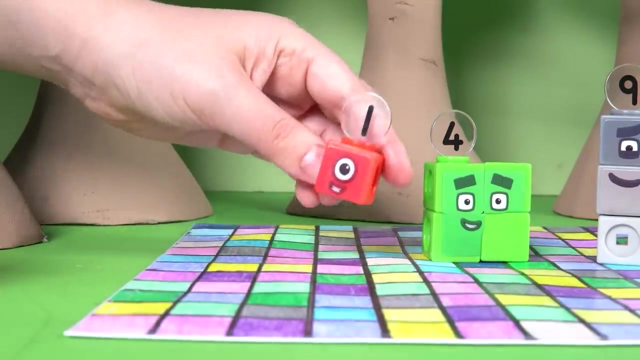 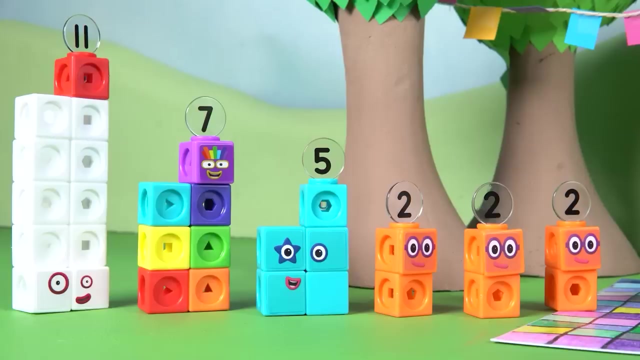 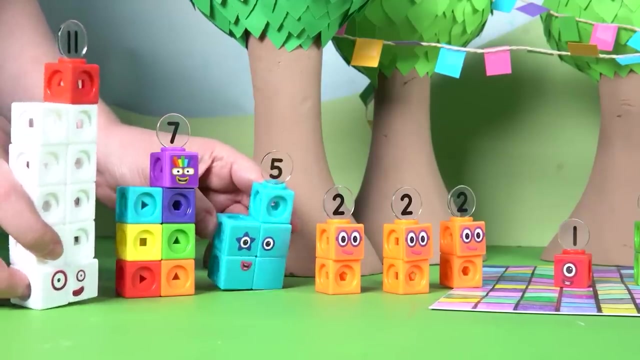 Shhh, Number block nine is playing hide and square. There he is peeking out. Wow, Look at number block one. It's a little bit different than the square party fun, But wait, They're not square numbers. What will? 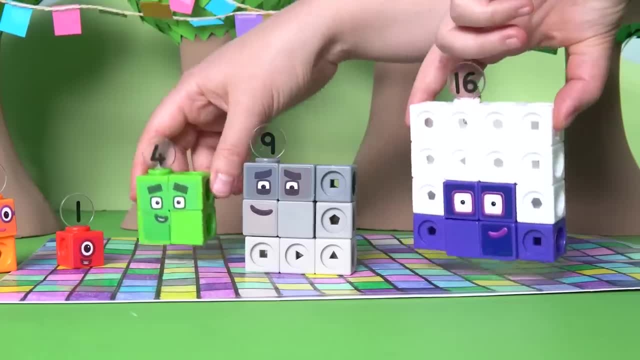 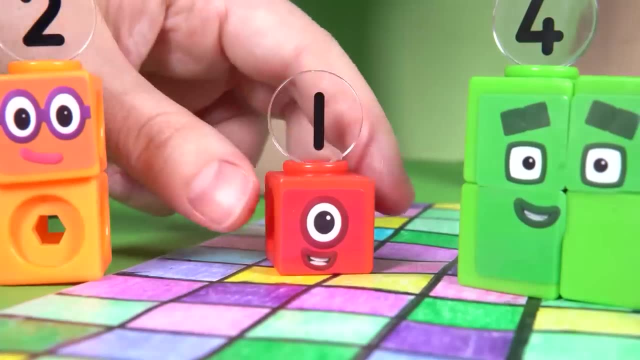 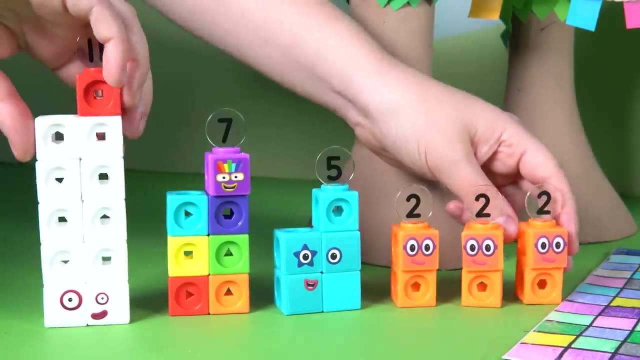 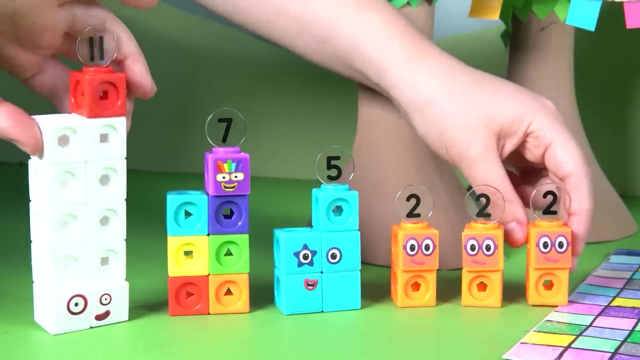 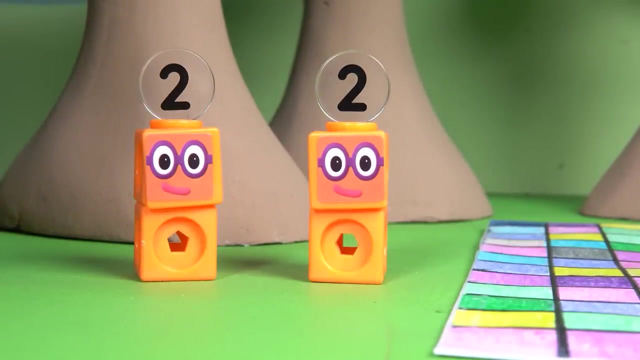 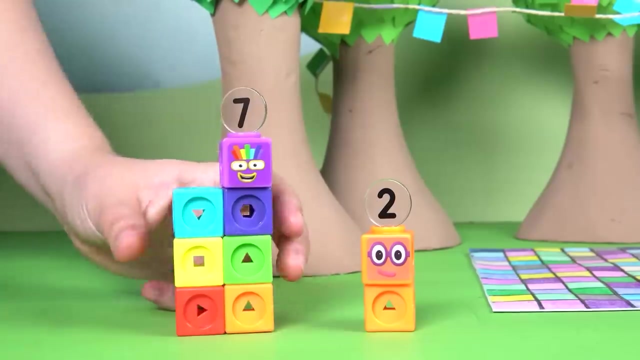 they do. Our square friends are thinking hard. They want to find a square partner. Aha, Number block one has a brilliant idea: Why not find a square partner Together? two number blocks can combine to make a square number, And there's. 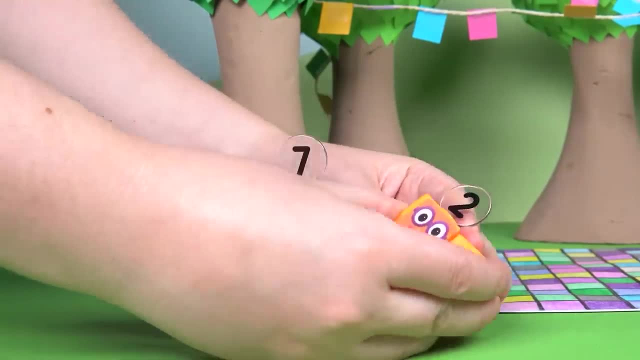 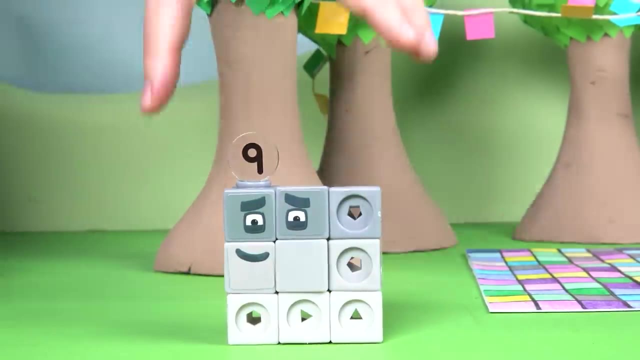 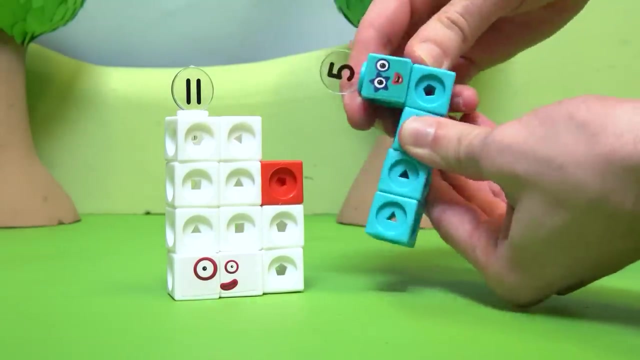 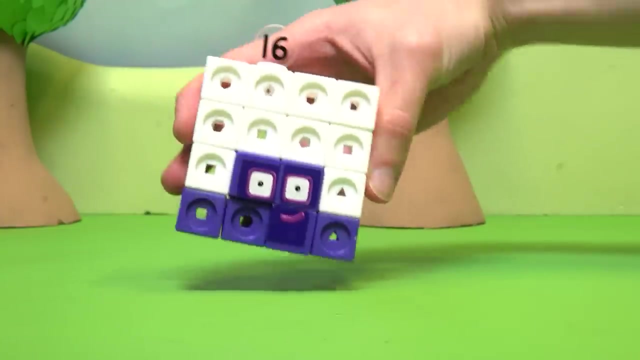 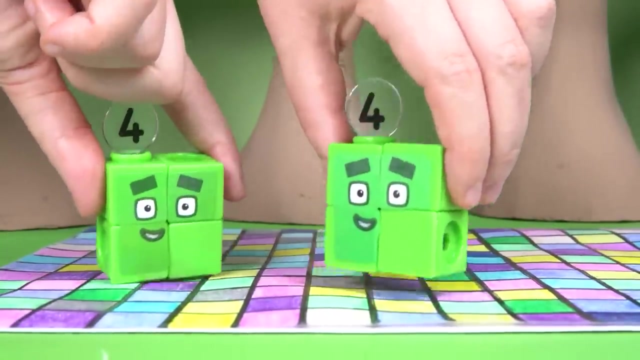 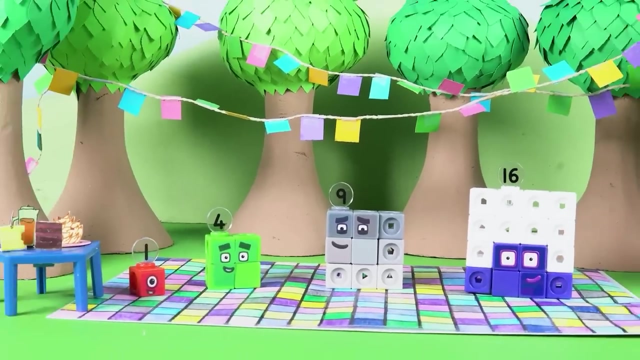 more. Number block two is pairing up with number block seven. Two plus seven equals nine. Another perfect square. Oh, and look over there. Number block five is a beautiful square. All the number blocks are coming together, Square or not they. 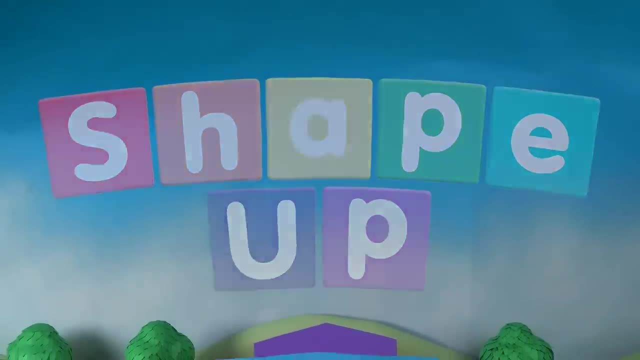 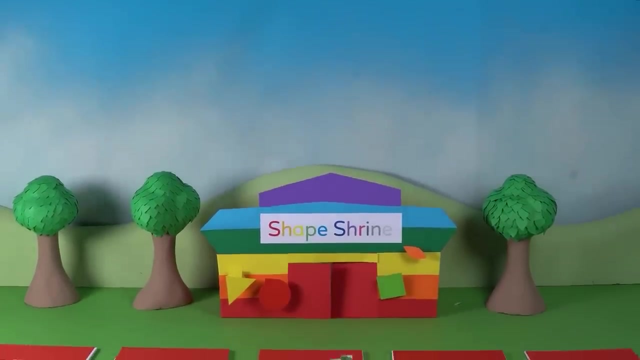 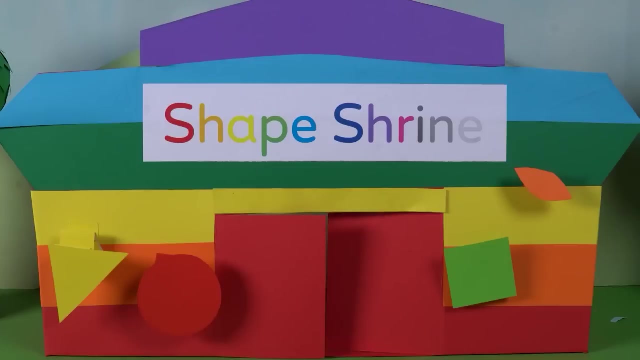 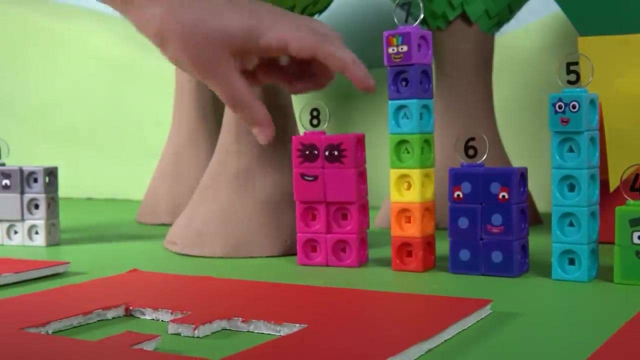 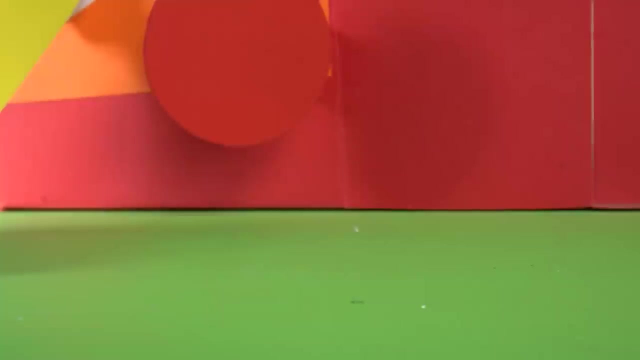 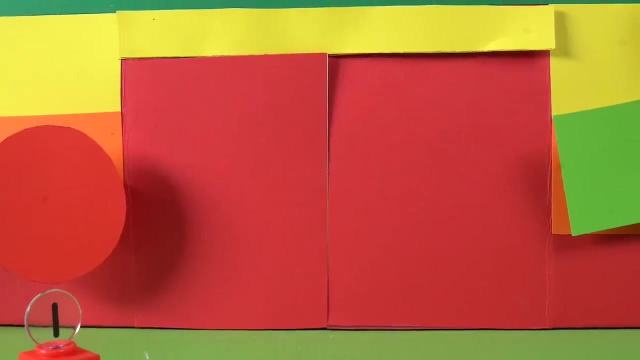 all enjoy the party and have a great time together. Wow, Welcome number explorers to Numbers of Different Shapes. Ah, and here are our number blocks, ready for a new adventure. They've travelled far and wide to explore the mysteries of 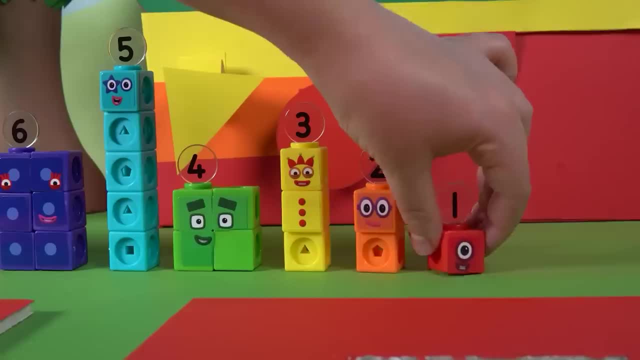 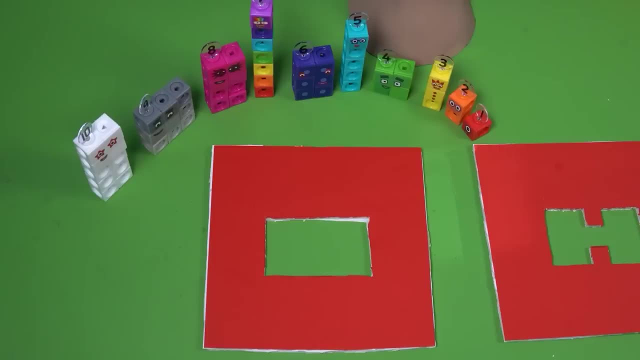 the Shape Shrine. But oh no, we haven't found the number block yet. Let's see what number block one has found In this puzzle. there are shapes to fill, Then more puzzles to solve. Let's try to solve this puzzle. 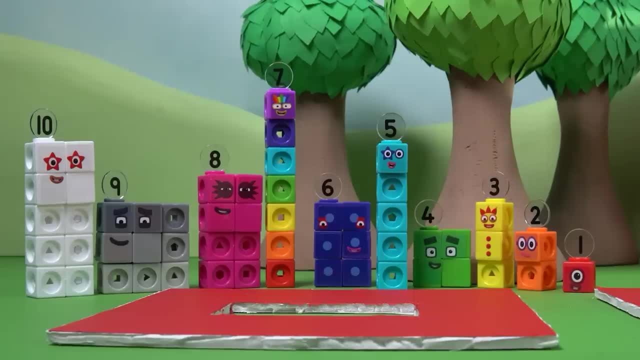 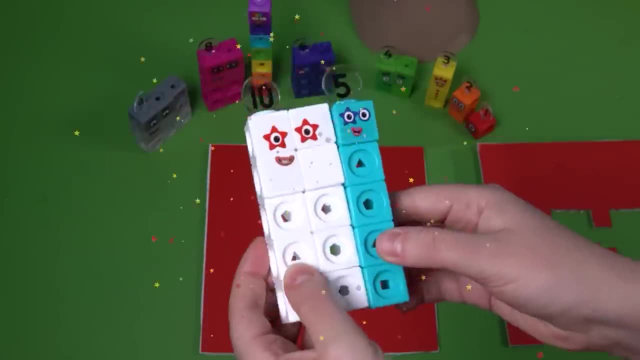 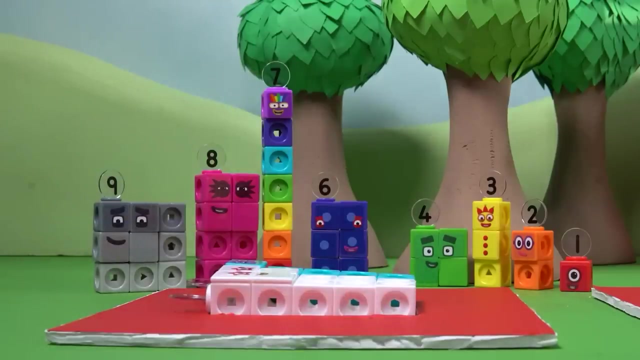 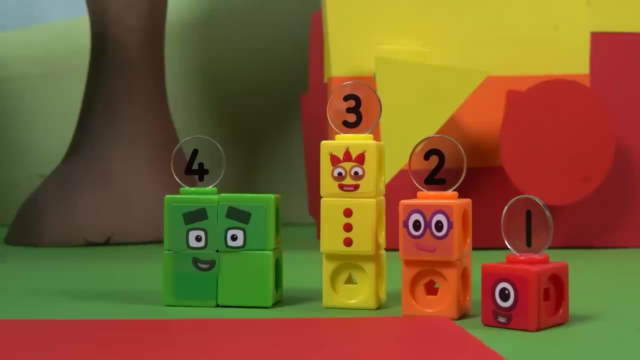 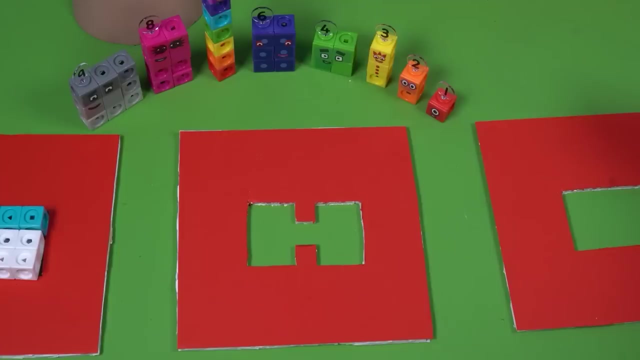 Number block five is ready, but she can't fill the shape alone. Who can help her? Yay, Ten and five make the perfect team. They've filled the first challenge with two spaces, both needing six blocks, with a tiny space in the. 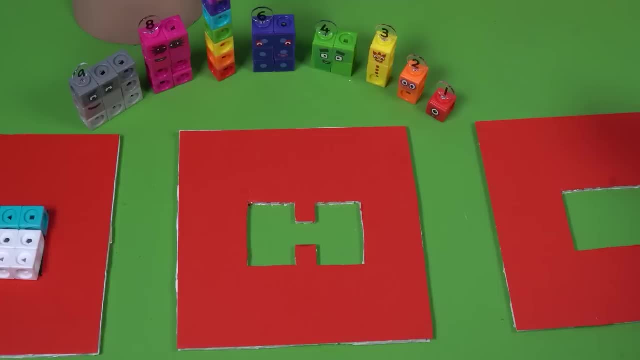 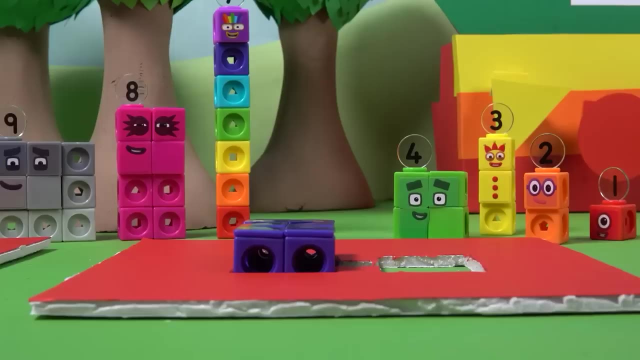 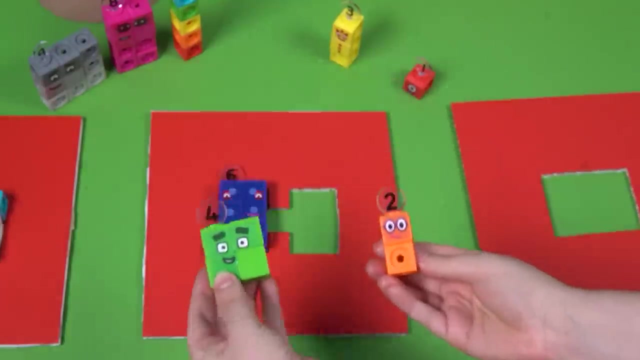 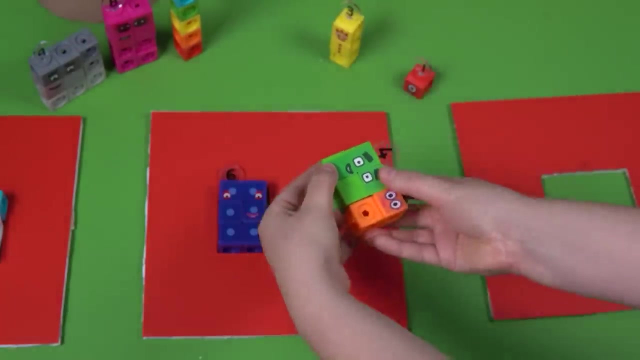 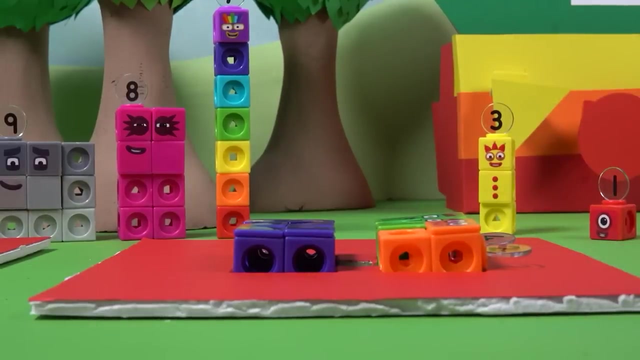 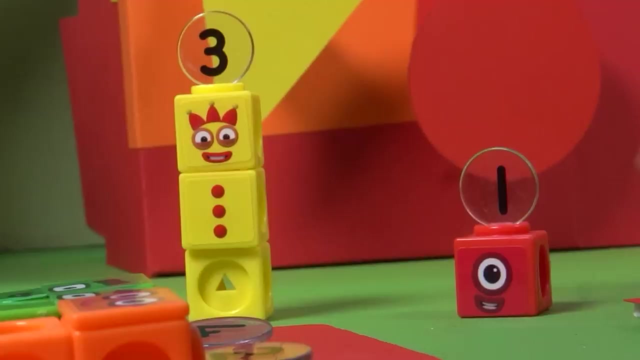 middle. I wonder how our number blocks will tackle this one. That's right number. block six is up for the challenge. Four and two have come together to fill the second space. But oh, what about the tiny space in the middle? Hmm, 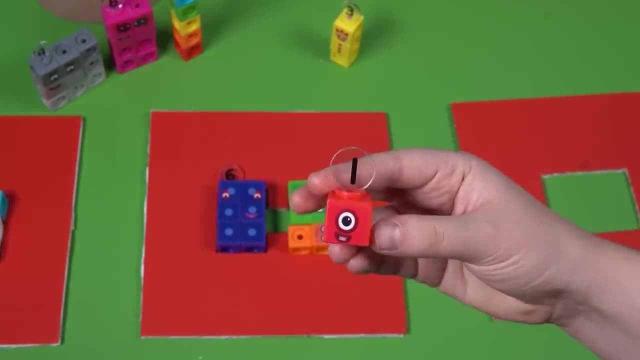 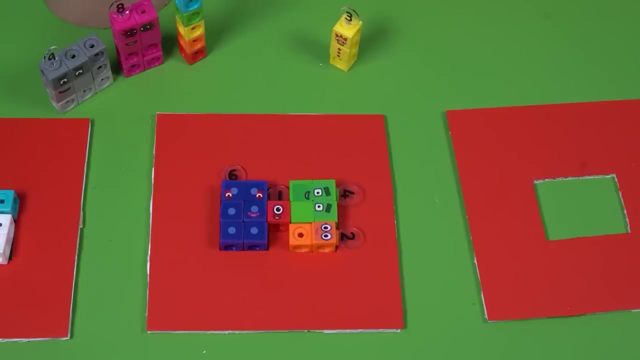 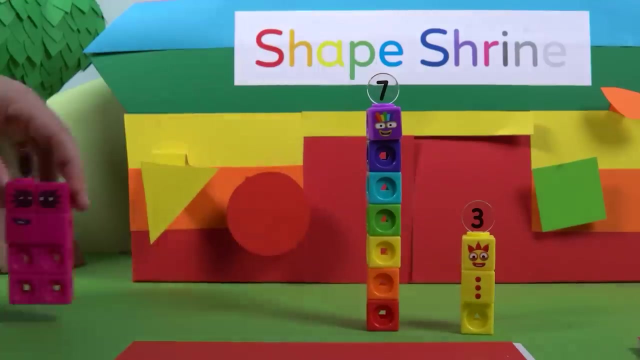 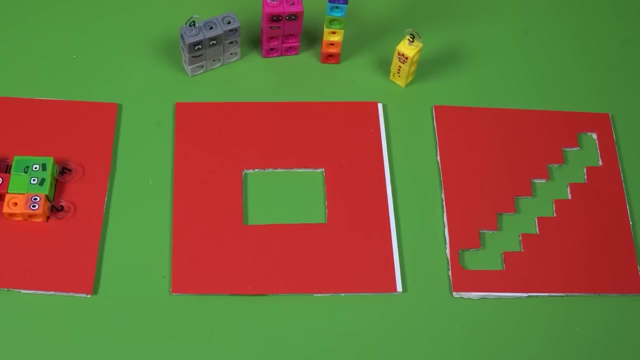 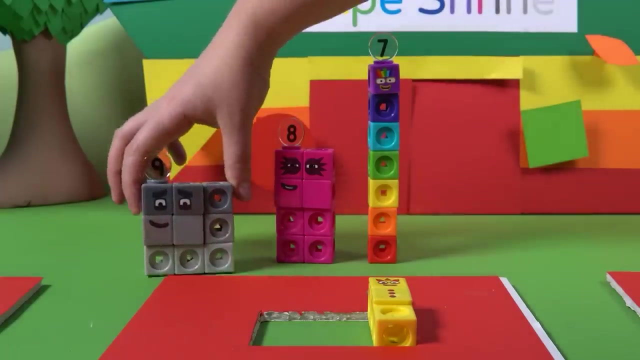 I wonder which number block is just that? Our number blocks have filled the second puzzle. Fantastic job, Aha, Here's our next puzzle. This one looks extra rectangle-y. I wonder which of our number blocks will step up to the next shape. 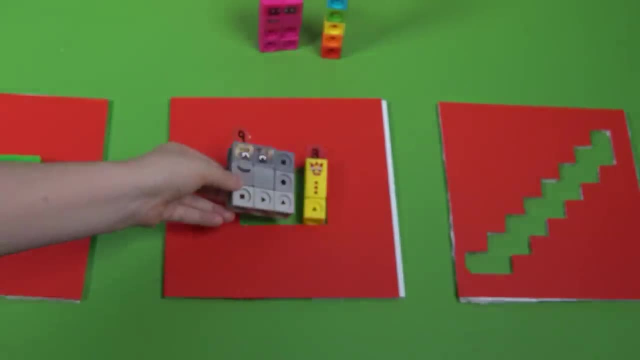 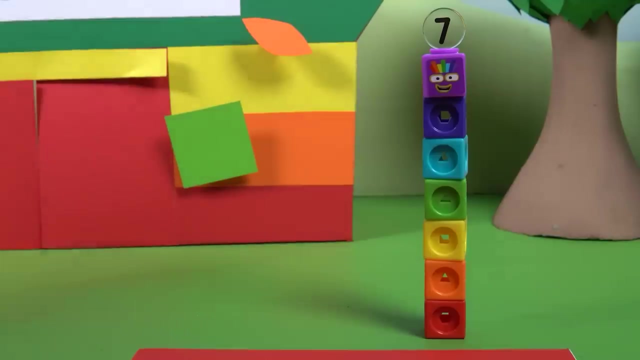 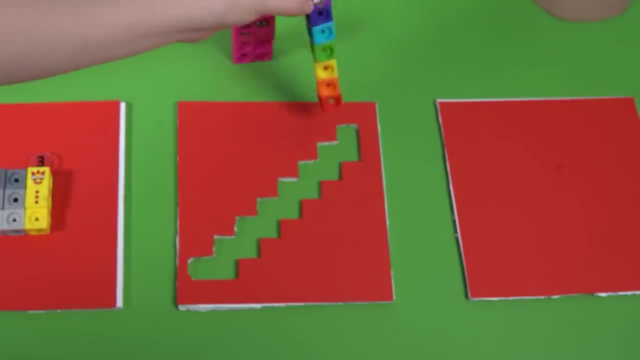 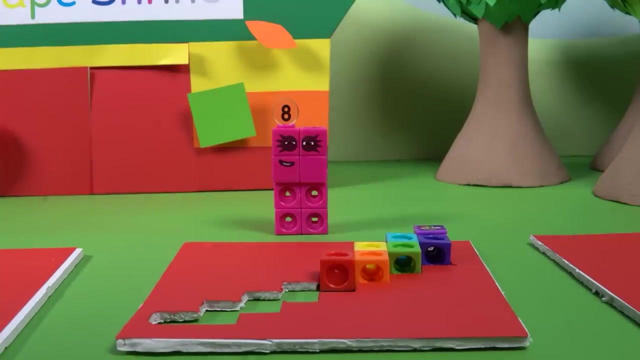 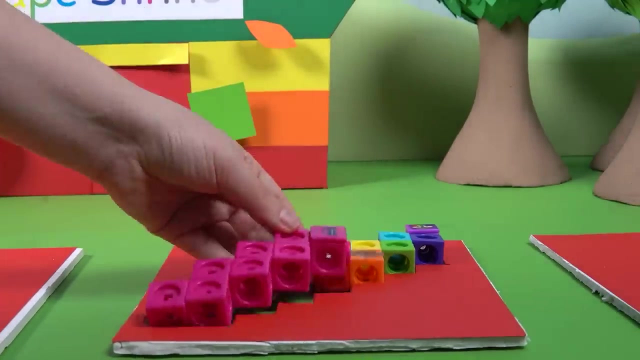 That means Amazing. Three times three makes nine. They've perfectly filled the shape. And now onto the next shape. Oh, this one's a zig-zag shape. What's this left? Fantastic, Seven and eight have come together to fill. 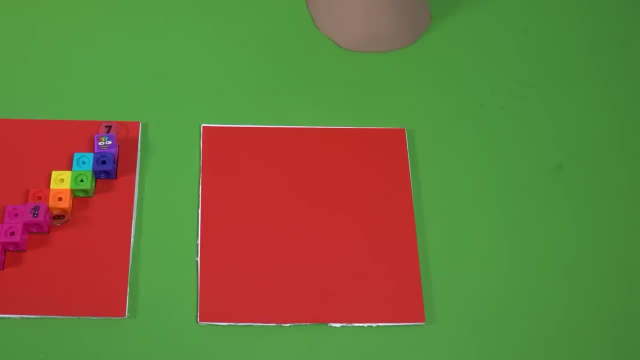 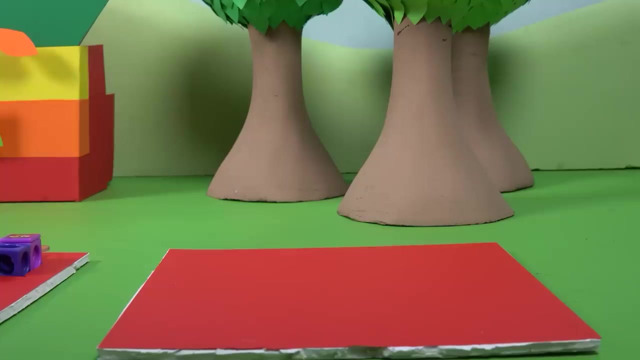 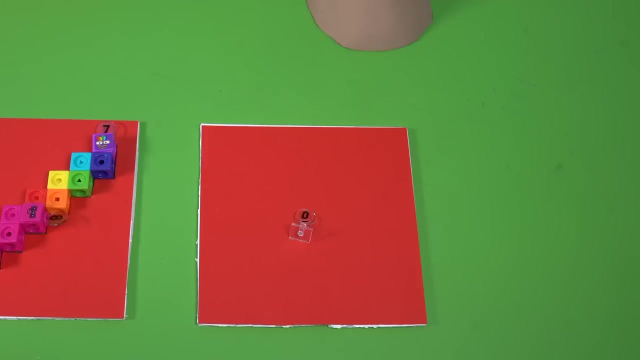 the zig-zag shape. Look at that. teamwork, The final puzzle. But wait, this pillar doesn't have a shape. There's nothing there. Look, there are zero shapes in this puzzle And zero corners And zero edges. There's. 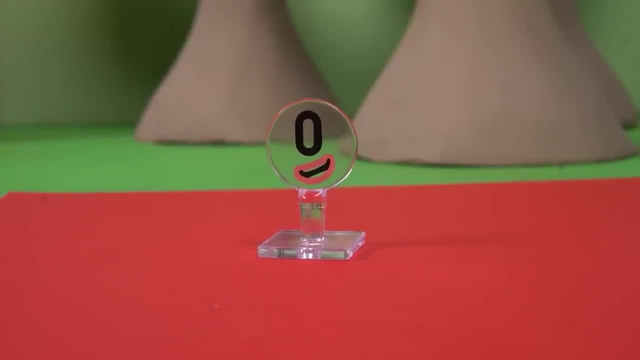 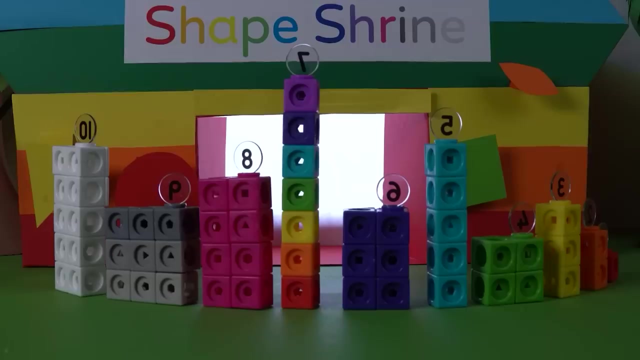 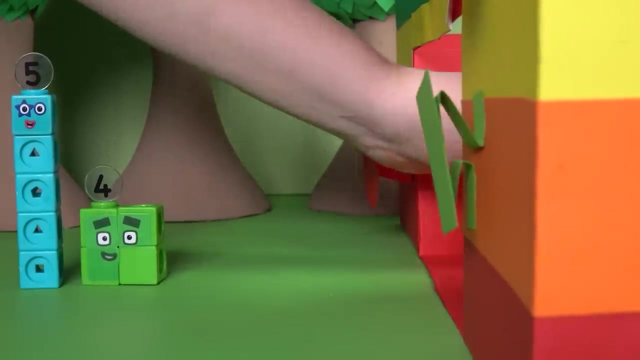 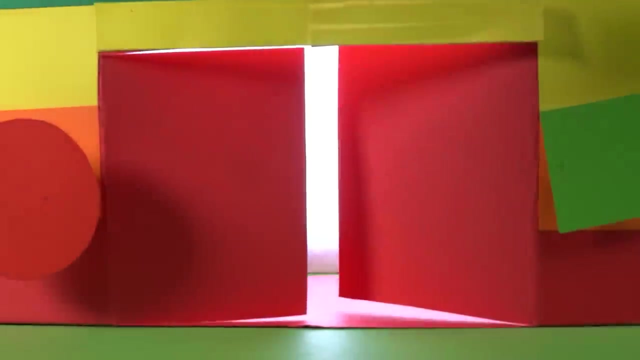 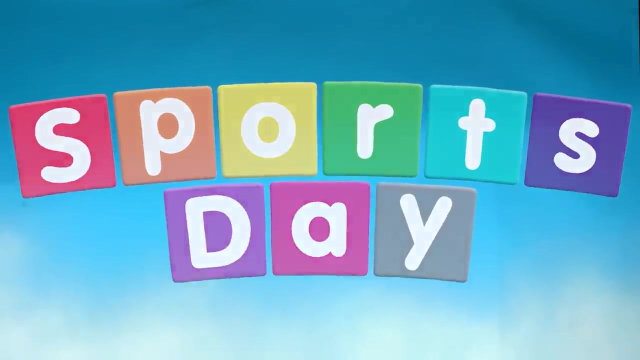 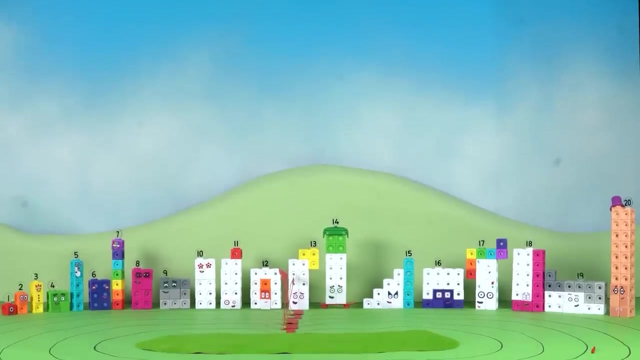 nothing there at all. That's perfect for zero. They did it. The door to the shape shrine has unlocked, And so our number block 10 has unlocked the mysteries of the shape shrine. Hello, number explorers, Welcome back to another imagination. 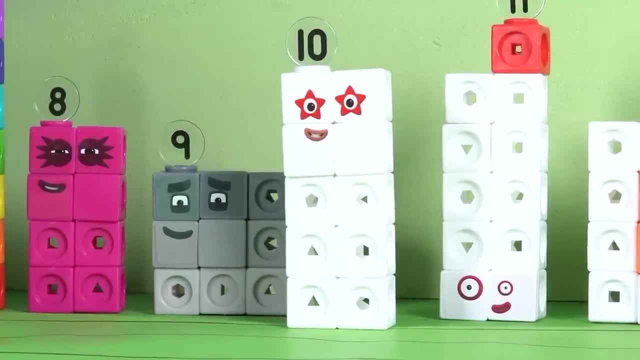 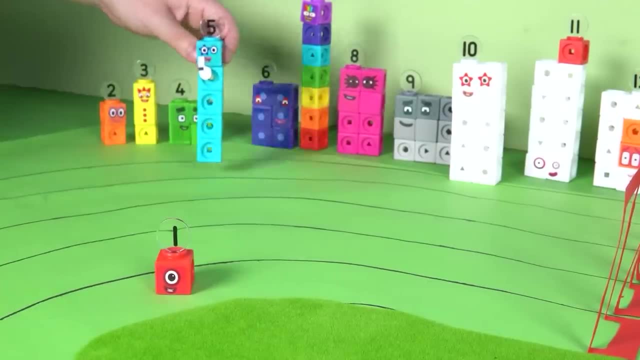 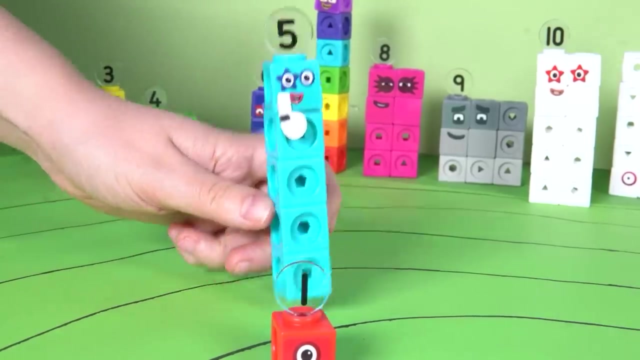 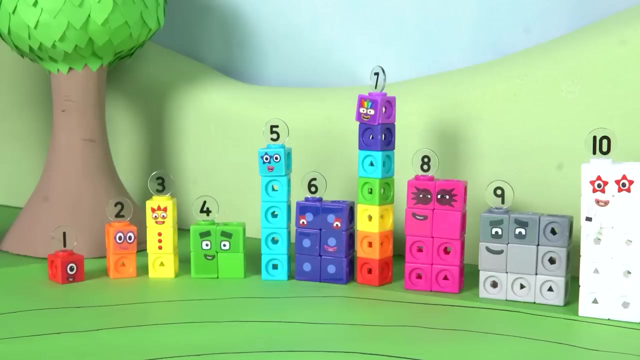 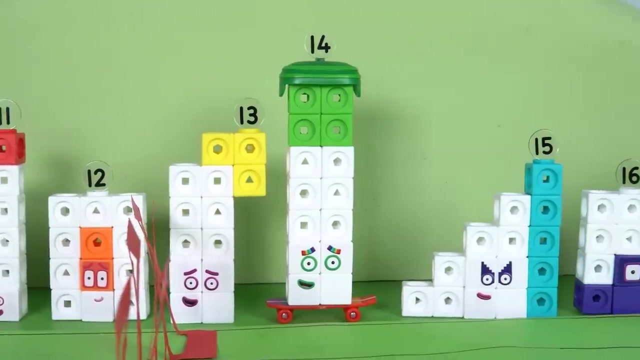 adventure with the number blocks. Here's number block one, waiting at the starting point One and ready to go, Whistles blown. It's number block five, our sports day organizer. She's making sure everything is in order From one to the. 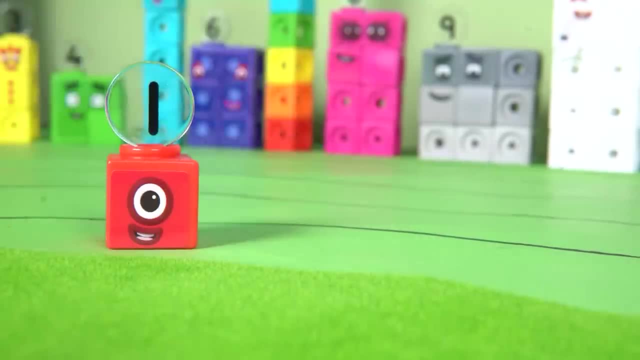 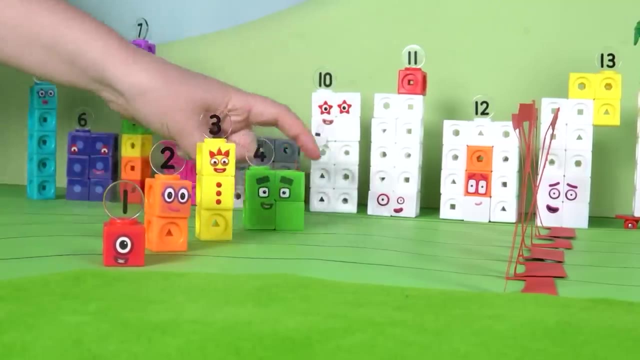 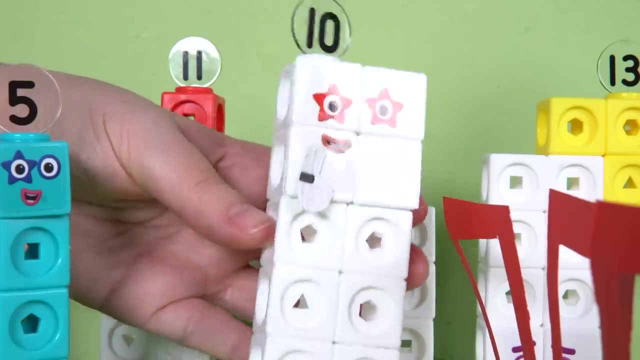 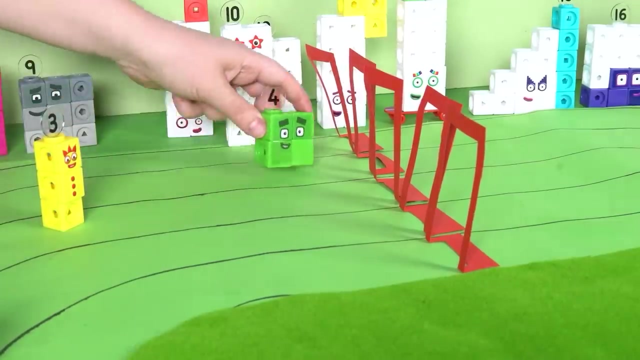 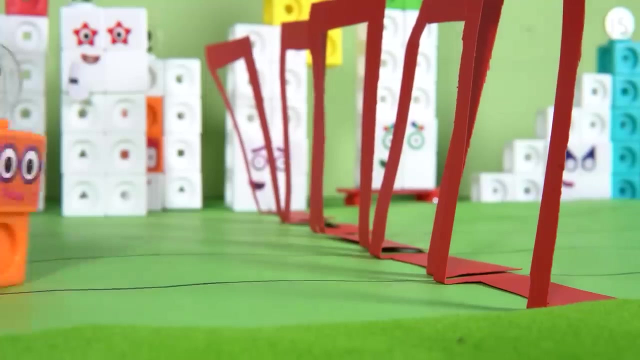 next, Ready for the big day. And now number blocks. one and five are eager to race, And they're off. Here come the rainbow hurdles. Let's see what they're made of. Three, four and five make it look easy. 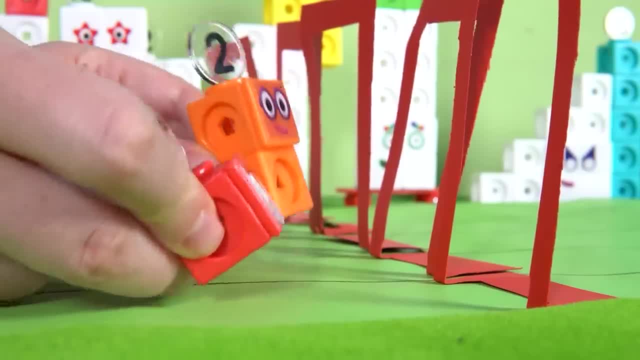 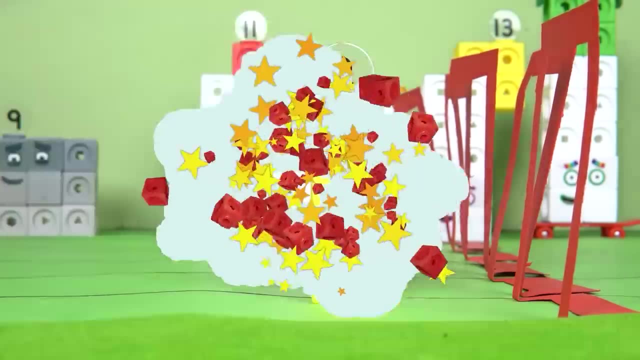 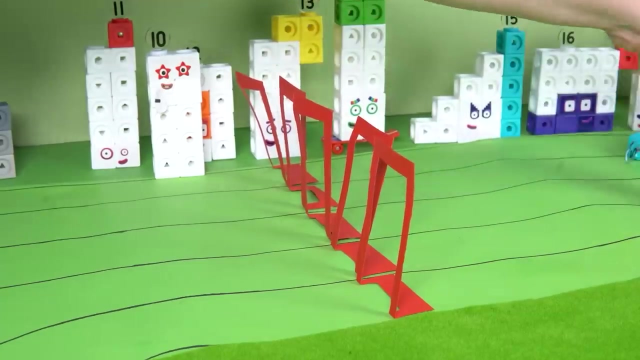 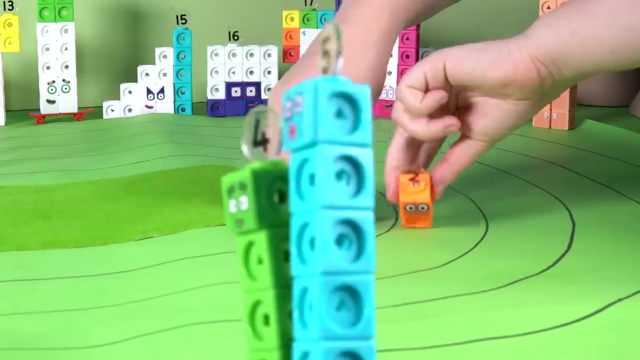 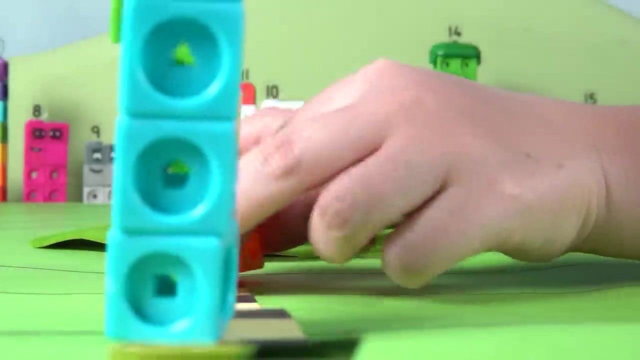 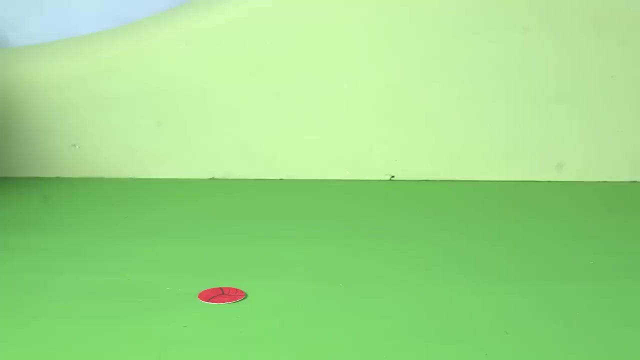 soaring over the hurdles. Oh no, Number block one and two are too short to jump over the hurdle with ease And they're back. One and two working together show that teamwork makes the dream work And the winner is, oh, too close.